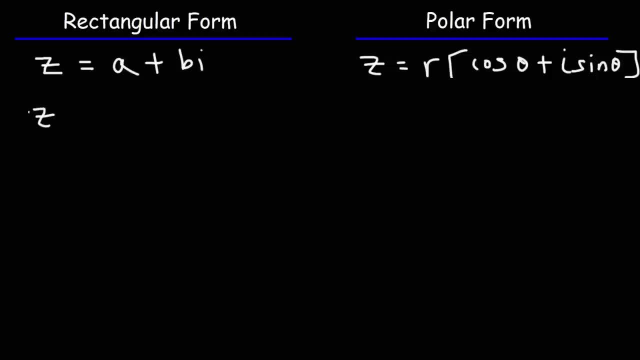 Feel free to do that. Now, the absolute value of a complex number is going to be the square root of a squared plus b squared. r is equal to the same thing. r is equal to a squared plus b squared, The square root of that, of course. 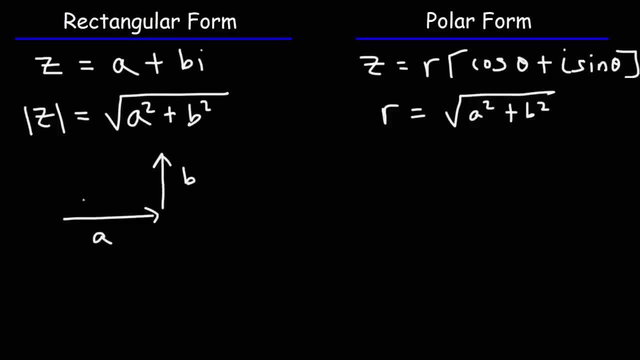 So this is a, this is b and the hypotenuse is going to be the absolute value of z, And the same is true for r. This is a, this is b and this is r. Inside of that we have the angle theta. 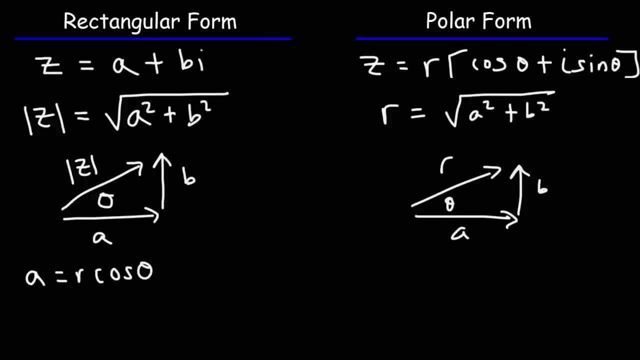 a is equal to r cosine theta And b is equal to r sine theta, So these two formulas are useful if you need to convert it from polar form to rectangular form. Now, to go from rectangular form to polar form, you need this equation. 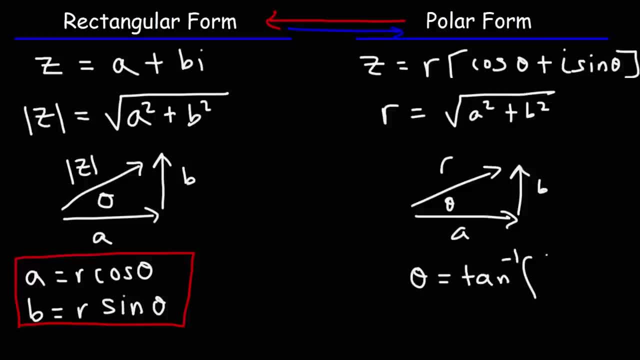 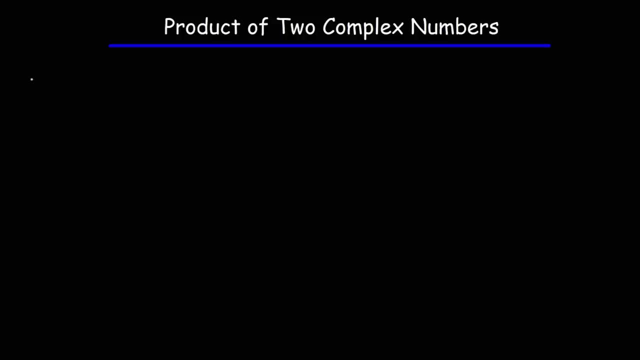 Theta is equal to r tangent b over a. So if you know a and b, you can calculate r using this formula And you can calculate theta using that formula. Now let's say if you have two complex numbers, z1 and z2.. 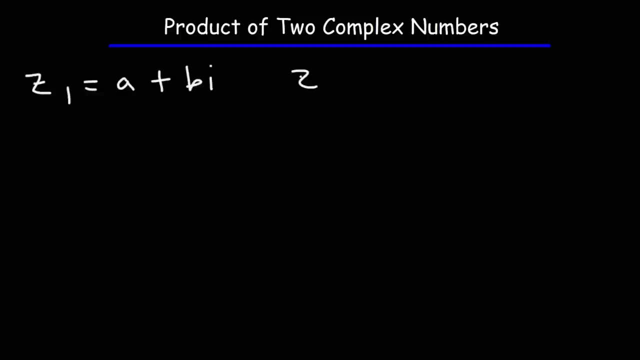 If they're given to you in rectangular form, you could simply multiply them. this way It's going to be a plus bi times a plus bi, And you could FOIL it. So that is not too difficult to do. But more often than not it's going to be given to you in polar form. 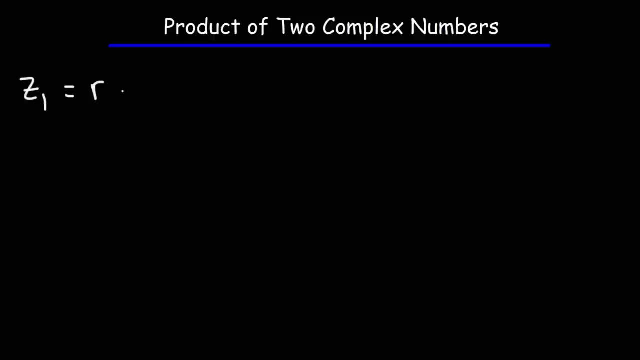 So let's say, if you have z1 in polar form, which is r1 times cosine theta 1.. And you have z2, which is r2 cosine theta 1 plus i sine- actually this should be theta 2.. And then plus i sine theta 2.. 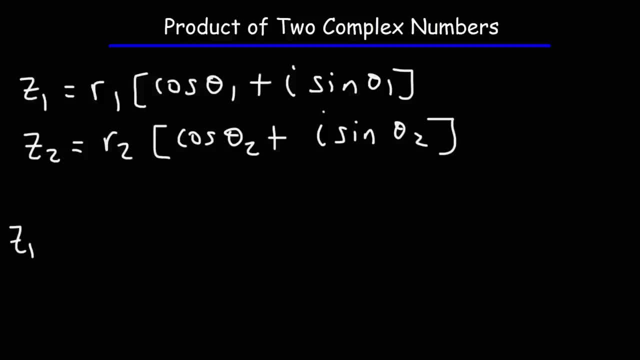 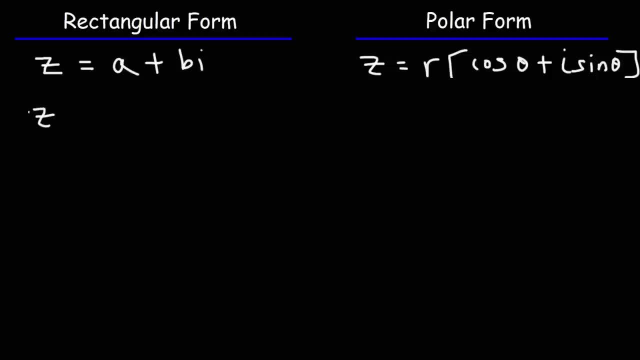 Feel free to do that. Now, the absolute value of a complex number is going to be the square root of a squared plus b squared. r is equal to the same thing. r is equal to a squared plus b squared, The square root of that, of course. 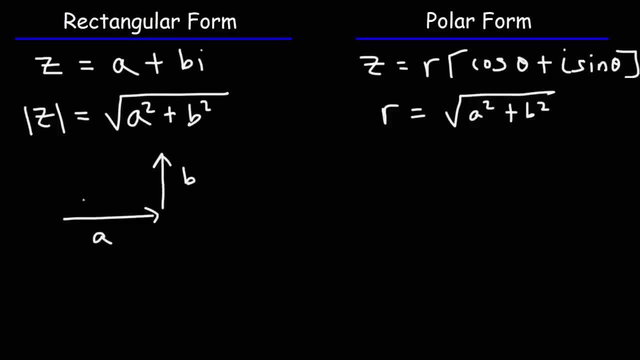 So this is a, this is b and the hypotenuse is going to be the absolute value of z, And the same is true for r. This is a, this is b and this is r. Inside of that we have the angle theta. 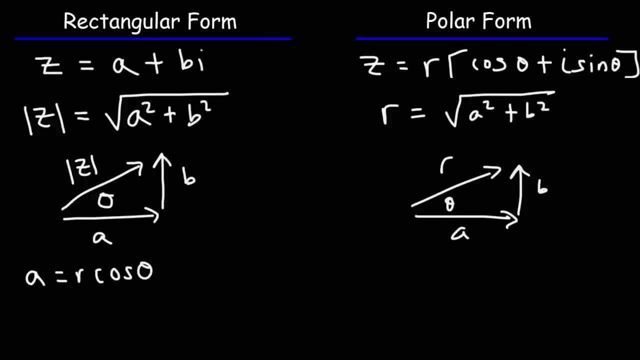 a is equal to r cosine theta And b is equal to r sine theta, So these two formulas are useful if you need to convert it from polar form to rectangular form. Now, to go from rectangular form to polar form, you need this equation. 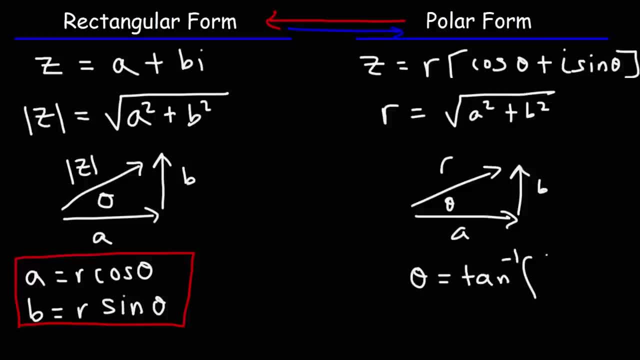 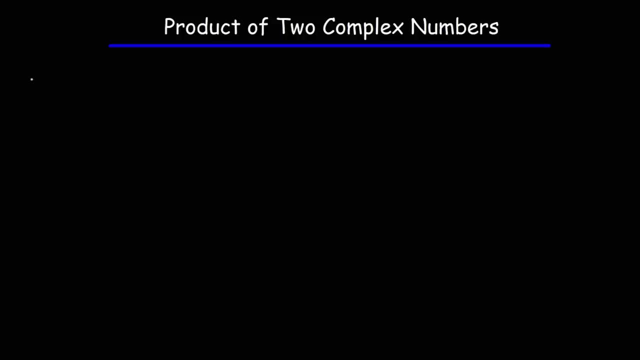 Theta is equal to r tangent b over a. So if you know a and b, you can calculate r using this formula And you can calculate theta using that formula. Now let's say if you have two complex numbers, z1 and z2.. 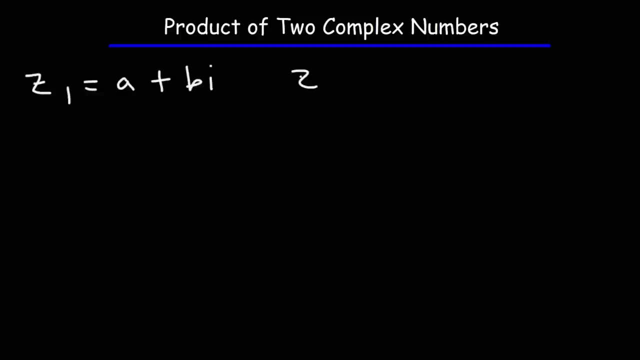 If they're given to you in rectangular form, you could simply multiply them. this way It's going to be a plus bi times a plus bi, And you could FOIL it. So that is not too difficult to do. But more often than not it's going to be given to you in polar form. 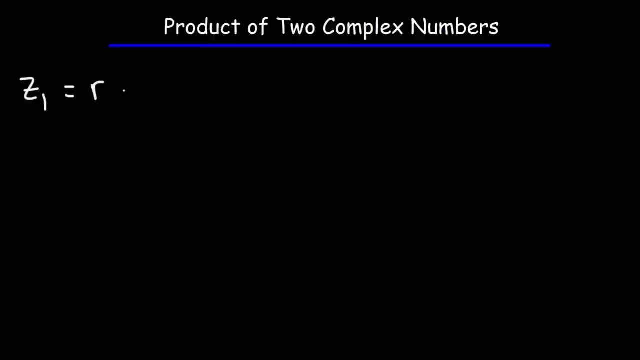 So let's say, if you have z1 in polar form, which is r1 times cosine theta 1. plus i sine theta 1.. And you have z2, which is r2 cosine theta 1 plus i sine, actually this should be theta 2.. 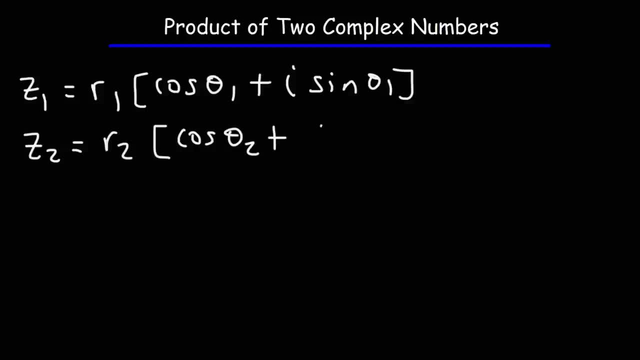 And then plus i sine theta 2.. The product of z1 is going to be theta 2.. And then plus i sine theta 2.. The product of z1 is going to be theta 2.. The product of z1 and z2 is going to be. 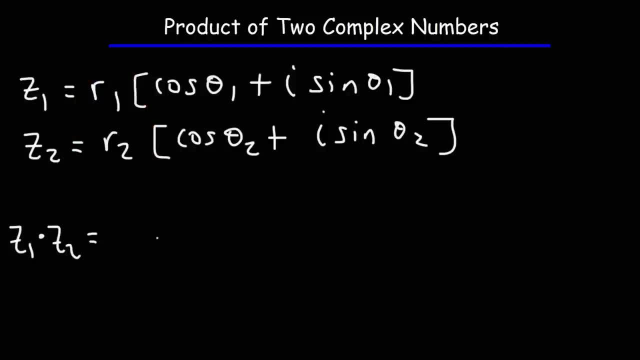 So what you would do is you would multiply r1 and r2.. And then it's going to be cosine, And then you would add the two angles, So cosine theta 1 plus theta 2.. And then, plus i sine, theta 1 plus. 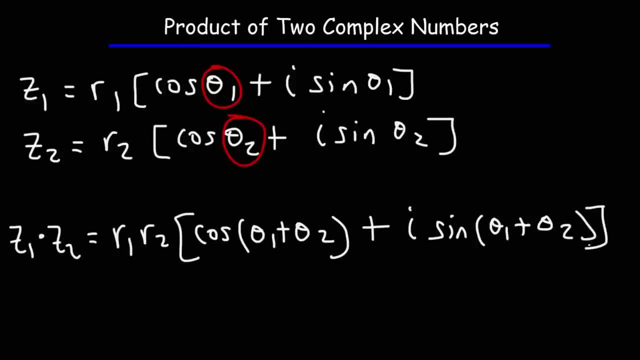 theta 2.. So that's how you could find the product of two complex numbers. So you could find the product of two complex numbers in polar form. So multiply the r values out of the angles. Now, the next thing that you need to be able to do, 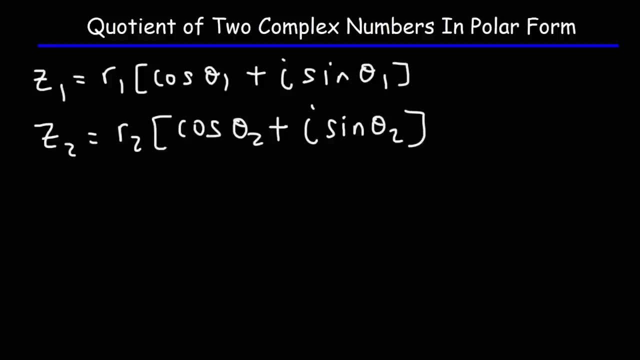 is you need to be able to find the quotient of two complex numbers in polar form. The way you would do that, the way you would find z1 divided by z2, is first you would divide the two r values, So it's going to be r1 divided by. 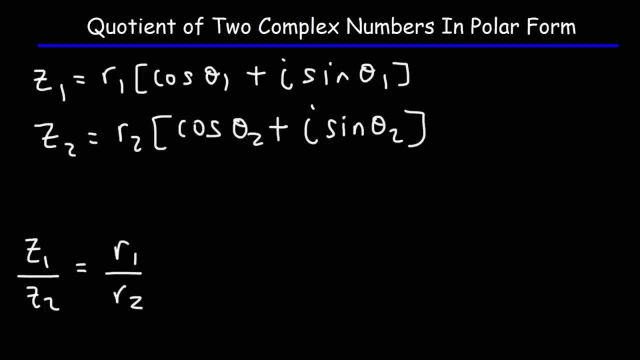 r2.. And then you need to subtract the two angles, So it's theta 1 minus theta 2.. So this is going to be times cosine theta 1 minus theta 2, plus i sine theta 1 minus theta 2.. So that's how you could find the quotient. 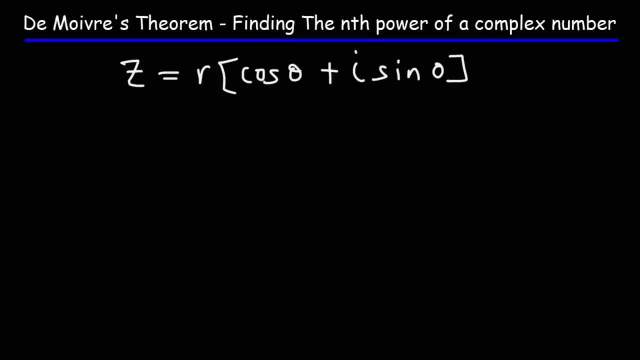 of two complex numbers. Now let's write down the formula for using de Morvier's theorem in order to find the nth power of a complex number. So here we have z in polar form, But let's say, if we want to find z raised. 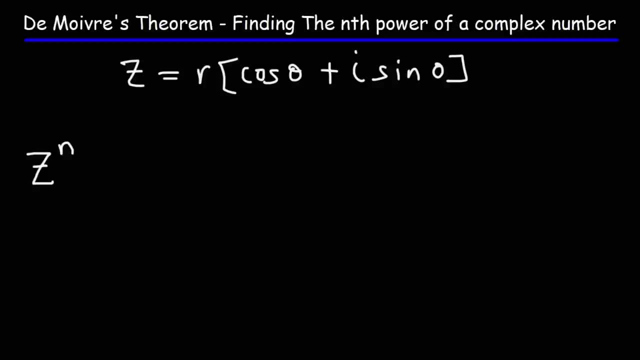 to some n power, like z squared or z to the third power. So here's what we need to do. This is basically all of this raised to the n power, So this is equal to r cosine theta plus i sine theta, all raised to the n power. 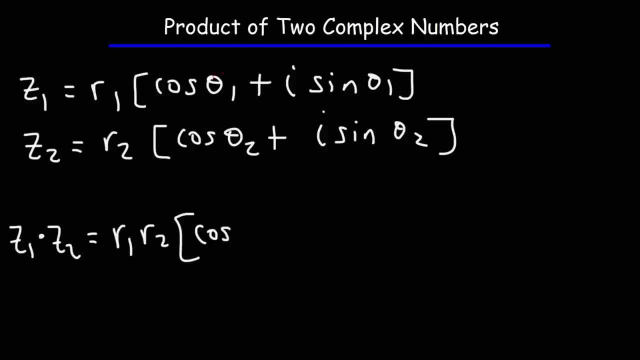 And then it's going to be cosine, And then you would add the two angles, So cosine, theta 1 plus theta 2.. And then plus i sine, theta 1 plus theta 2.. So that's how you could find the product of two complex numbers. 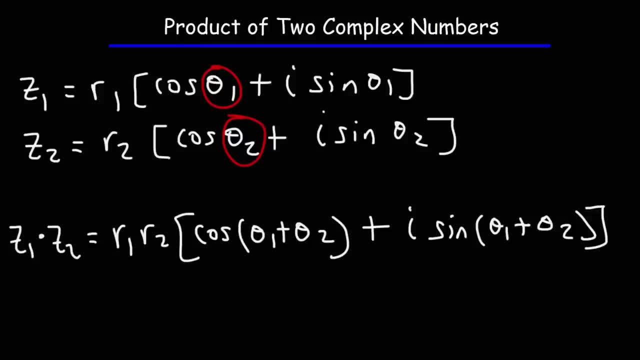 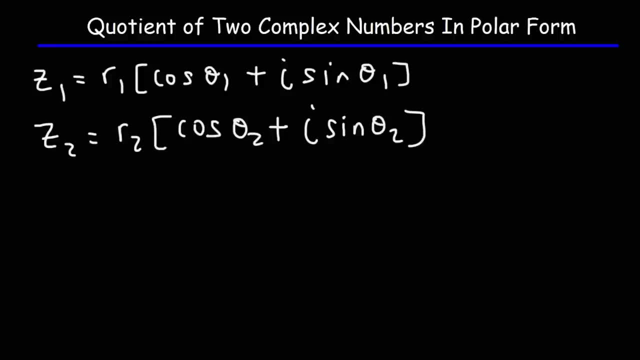 In polar form. So multiply the r values out of the angles. Now the next thing that you need to be able to do is you need to be able to find the quotient of two complex numbers in polar form. The way you would do that, the way you would find. 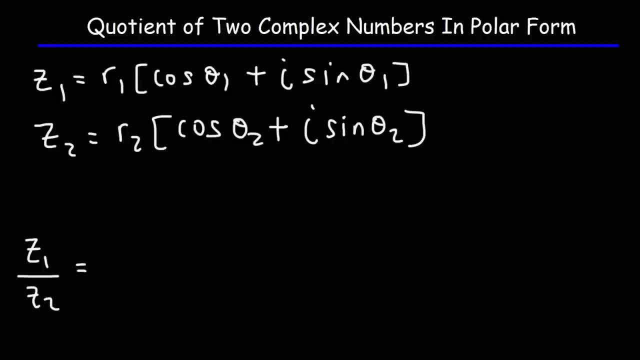 z1 divided by z2 is: first you would divide the two r values, So it's going to be r1 divided by r2.. And then you need to subtract the two angles, So it's theta 1 minus theta 2.. So this is going to be. 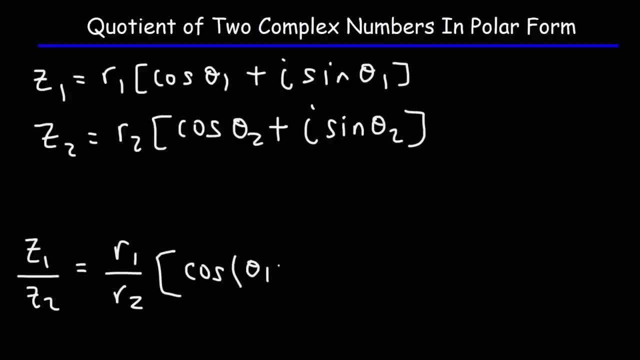 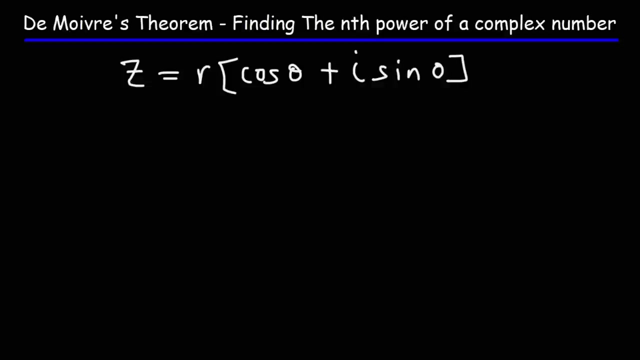 times cosine theta 1 minus theta 2, plus i sine theta 1 minus theta 2.. So that's how you could find the quotient of two complex numbers. Now let's try down the formula for using de Morvier's theorem in order to find the. 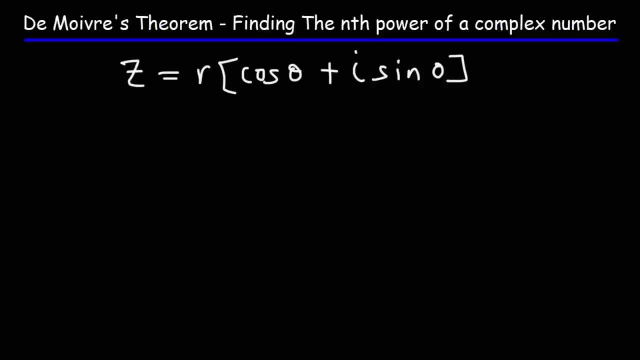 nth power of a complex number. So here we have z in polar form, but let's say, if we want to find z raised to some n power, like z squared or z to the third power, So here's what we need to do. This is basically all of. 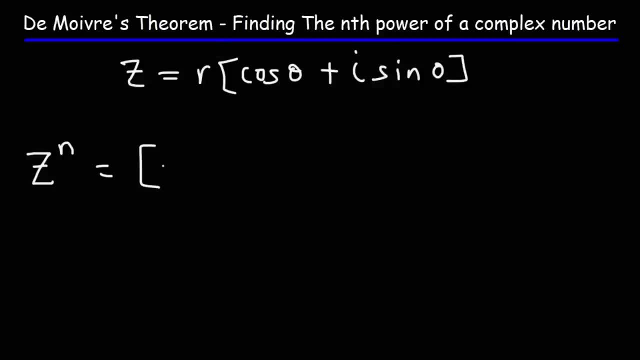 this raised to the nth power, So this is equal to r cosine theta plus i sine theta, all raised to the n power. So first we're going to raise r to the n, So this is r to the n. And for the other part, 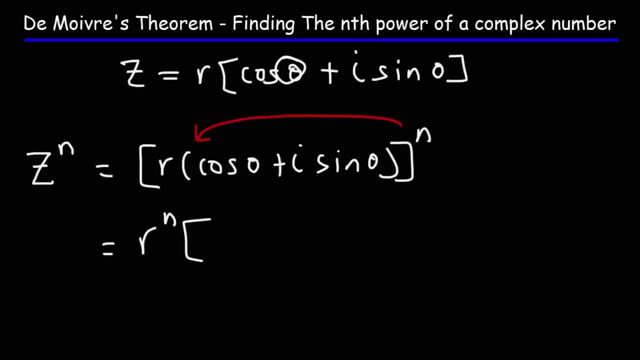 we're going to multiply theta by n, So it's going to be r to the n times cosine n. theta plus i sine theta Or theta n. So that's how you could use de Morvier's theorem to find the nth power of a complex number. 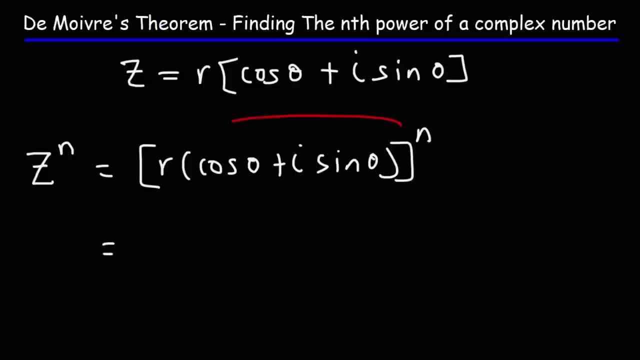 So first we're going to raise r to the n, So this is r to the n, And for the other part we're going to multiply theta by n, So it's going to be r to the n times. cosine n, theta plus i sine. 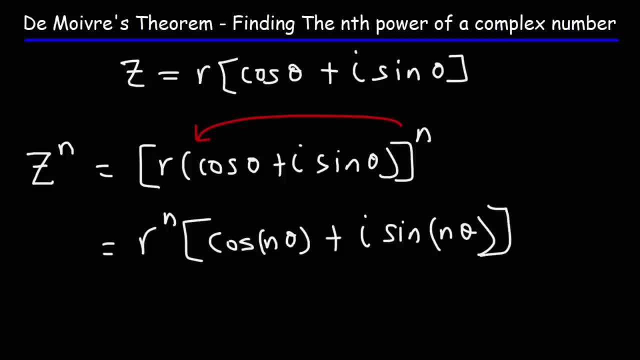 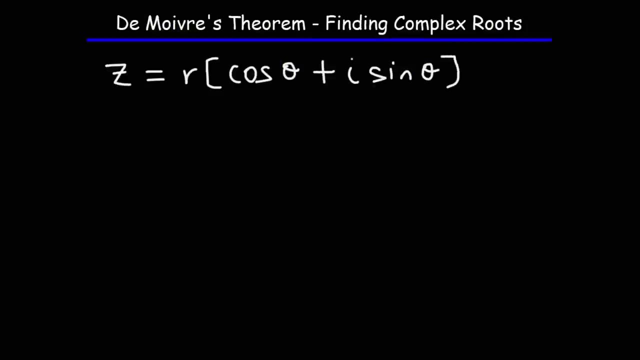 n, theta or theta n. So that's how you could use de Morvier's theorem to find the nth power of a complex number. So all you need to do is raise r to the n and multiply the angles by n. Now let's talk about how we could use 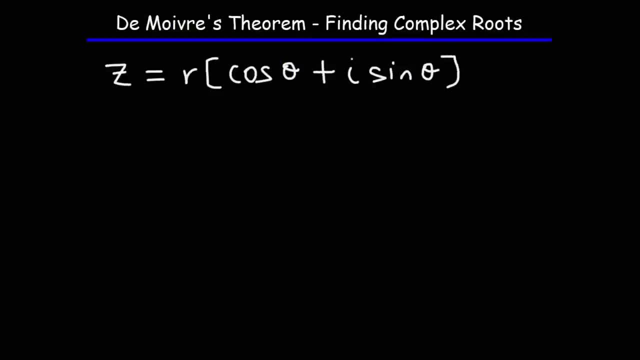 de Morvier's theorem to find complex roots. So here's the formula Z sub k, where k is an integer like 0,, 1,, 2, or 3.. This is going to be the nth root of r. So rather than 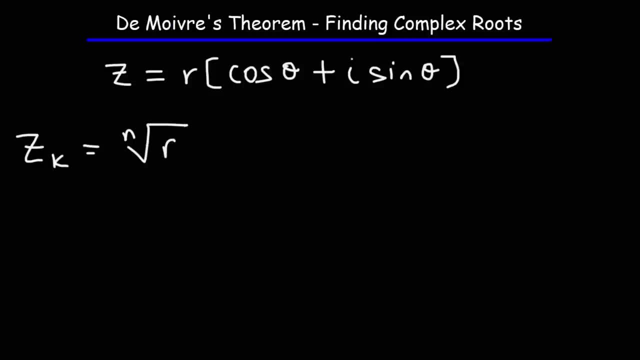 raise an r to the n, you raise an r to the 1 over n, or the nth root of r, And then it's going to be times cosine and this is going to be theta plus 2 pi k, By the way, instead of 2 pi k. 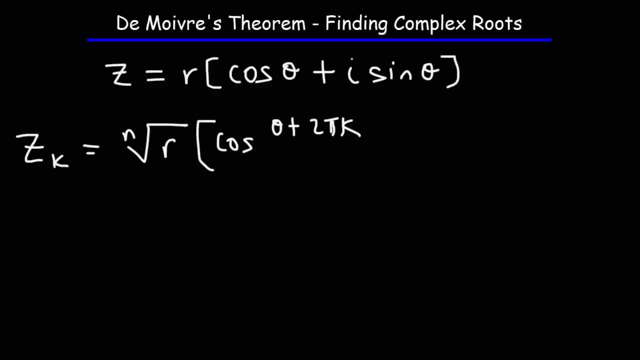 it could be 360 degrees If you want the angle in degrees. So theta plus 2 pi k over n, and then plus i sine, and it's going to be the same thing: theta plus 2 pi k over n. So that's the formula. 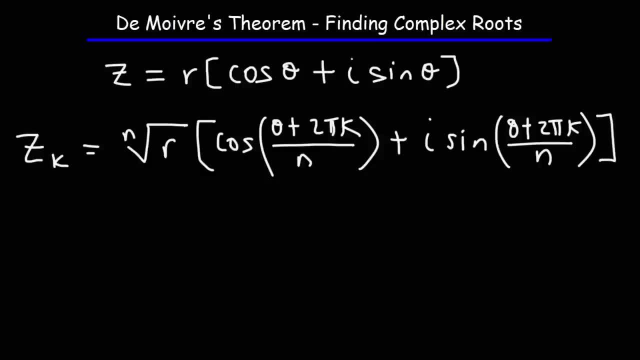 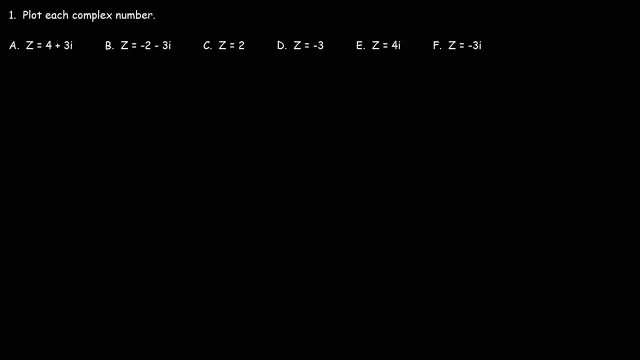 that you need to use if you want to find the nth roots of a complex number. So now let's work on some practice problems. Let's begin with this problem: Plot each complex number. So what we're going to do is we're going to draw a graph. 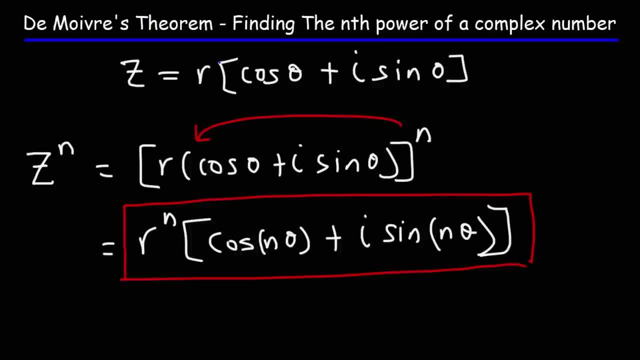 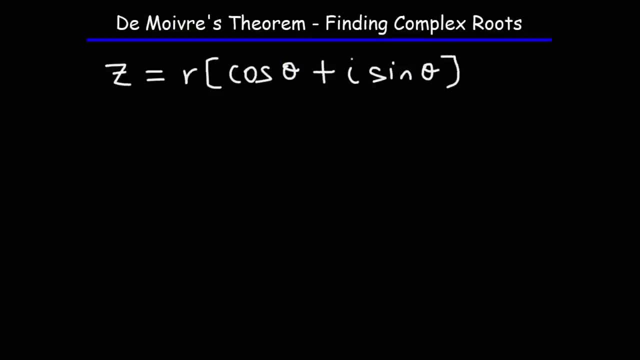 So all you need to do is raise r to the n and multiply the angles by n. Now let's talk about how we could use de Morvier's theorem to find complex roots. So here's the formula z sub k, where k is an integer like 0,. 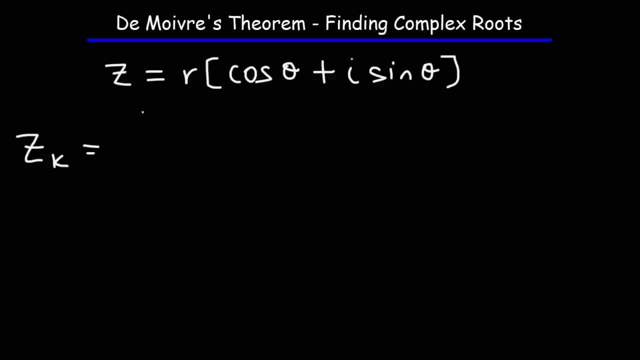 1,, 2, or 3.. This is going to be the nth root of r. So rather than raise an r to the n, you raise an r to the 1 over n or the nth root of r, And then it's going to be times cosine. 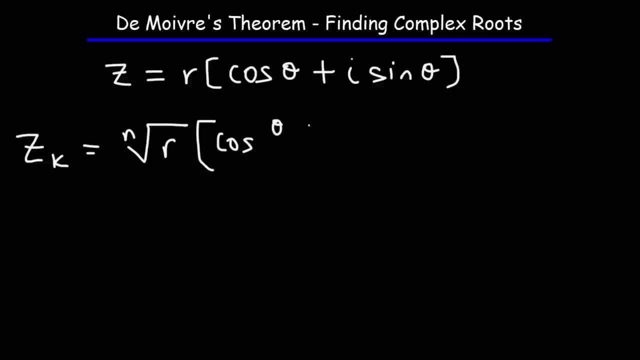 and this is going to be theta plus 2 pi k. By the way, instead of 2 pi k it could be 360 degrees, If you want the angle in degrees. So theta plus 2 pi k over n, and then plus i. 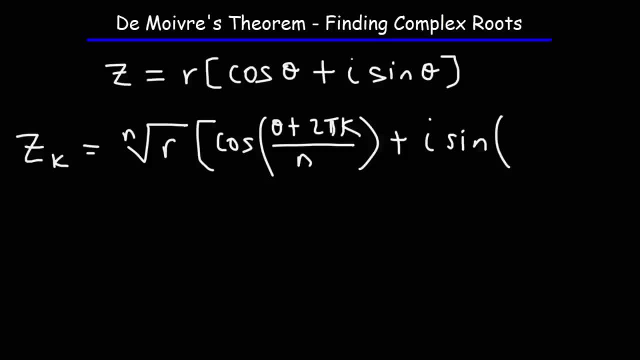 sine, and it's going to be the same thing: Theta plus 2 pi k over n. So that's the formula that you need to use if you want to find the nth roots of a complex number. So now let's work on some practice problems. 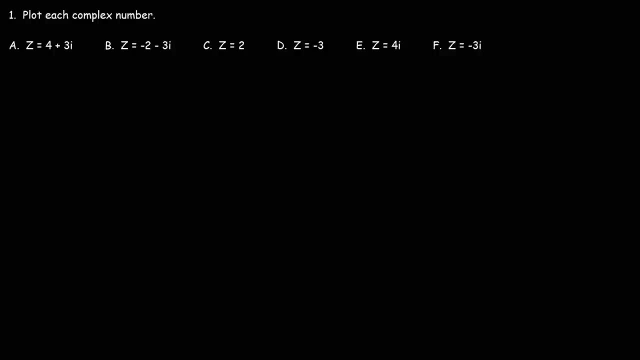 Let's begin with this problem, Plot each complex number. So what we're going to do is we're going to draw a graph And let's put some marks on the graph. So the x-axis is the real axis, The y-axis is going to be the imaginary axis. 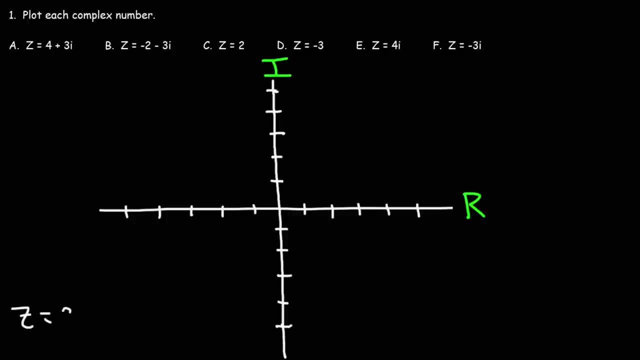 So keep in mind: z is in a plus bi form. a is the number that is basically the real number, b is associated with the imaginary number. So let's start with point a. We want to plot: z is equal to 4 plus 3i. 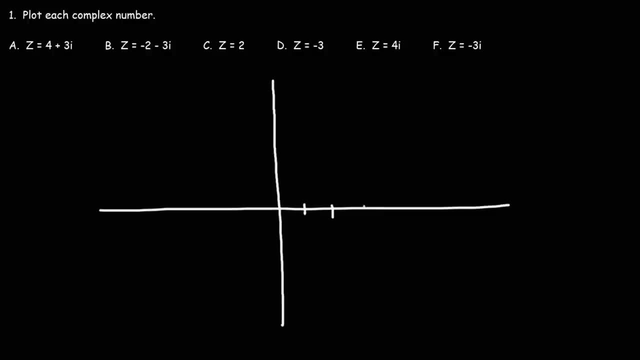 And let's put some marks on the graph. So the x-axis is the real axis, The y-axis is going to be the imaginary axis. So keep in mind: z is in a plus bi form, a is the number. that is basically the real number. 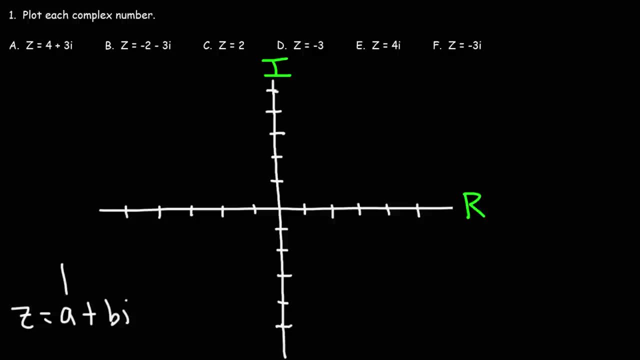 b is associated with the real number, b is associated with the imaginary number. So let's start with point a. We want to plot. z is equal to 4 plus 3i, So we're going to travel 4 units along the x-axis or the real axis. 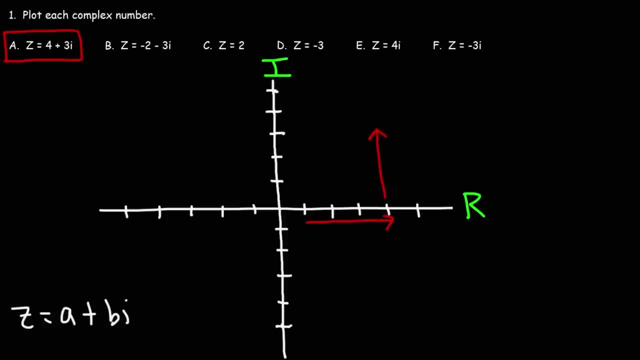 and then up 3 units along the imaginary axis. So 4 comma 3, we're going to get this point. So that's point a. Now b, So we have negative 2 minus 3i. So we're going to travel 2 units to the left. 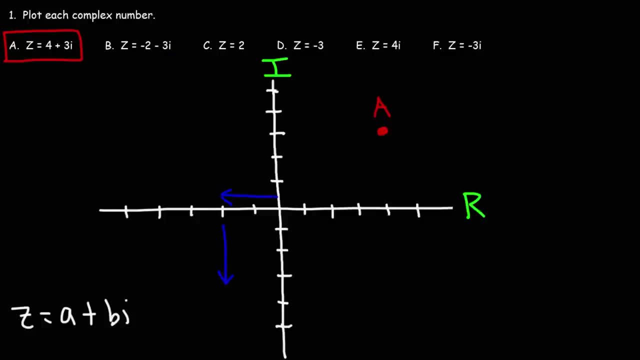 and then down 3 along the imaginary axis. So negative 2, negative 3, that's going to be right here. So that's point b, c, z is equal to 2.. You can see that as 2 plus 0i. 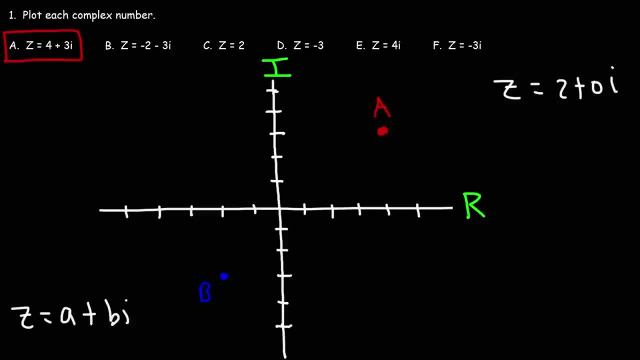 because there's no number in front of i. So we're going to travel 2 units along the real axis And since b is 0, we're not going to go up or down, So this is just going to be on the real axis. 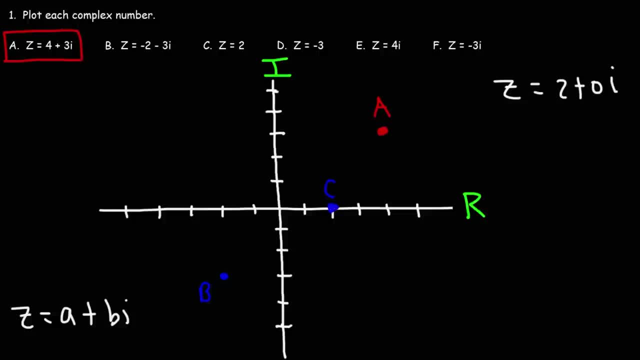 So that's point c. d, z is negative 3.. So we're just going to go 3 units to the left, So point d will be here. There's no i value associated with that. Now, for e, z is equal to 4i. 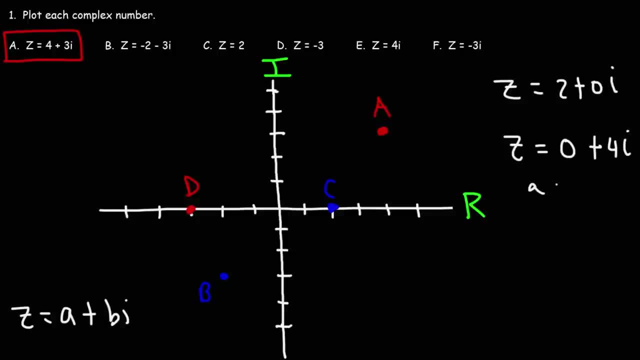 You can view this as 0 plus 4i, So a is 0, b is 4.. So think of it as plotting the point 0, 4.. This is going to be on the y axis, So that's going to be. 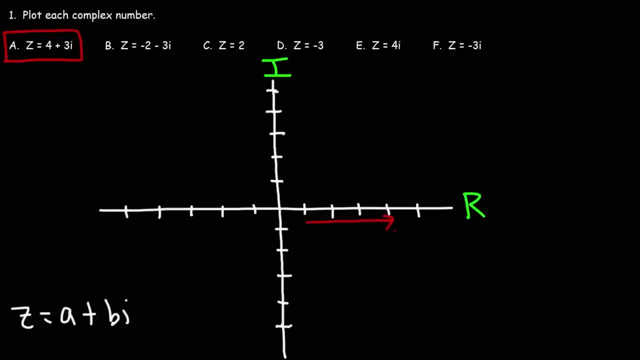 So we're going to travel 4 units along the x-axis or the real axis, And then up 3 units along the imaginary axis. So 4 comma 3. we're going to get this point. So that's point a. Now b: 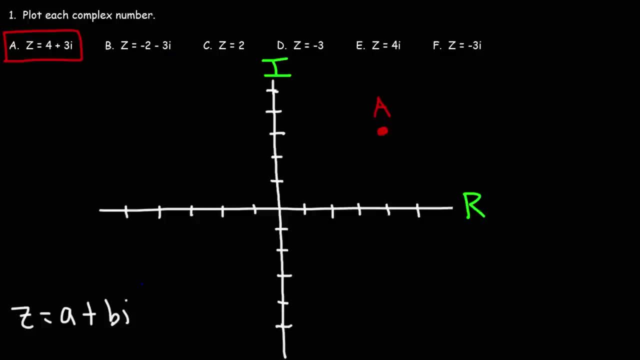 So we have negative 2 minus 3i. So we're going to travel 2 units to the left and then down 3 along the imaginary axis. So negative 2, negative 3. that's going to be right here. So that's point b. 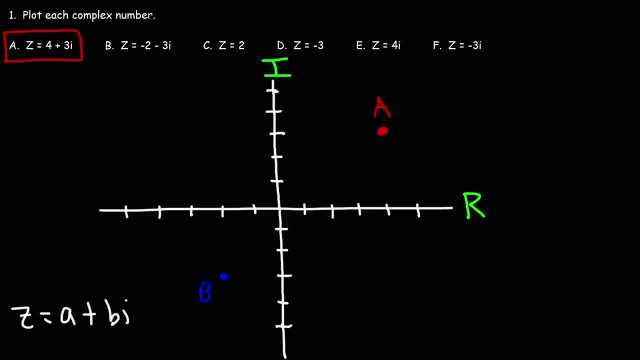 c, z is equal to 2.. You can see that as 2 plus 0i, because there's no number in front of i. So we're going to travel 2 units along the real axis And since b is 0, we're not going to go up or down. 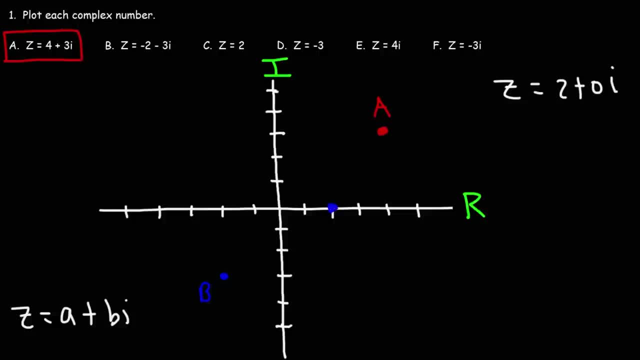 So this is just going to be on the real axis. So that's point c, d. z is negative 3, so we're just going to go 3 units to the left, So point d will be here. There's no i value associated. 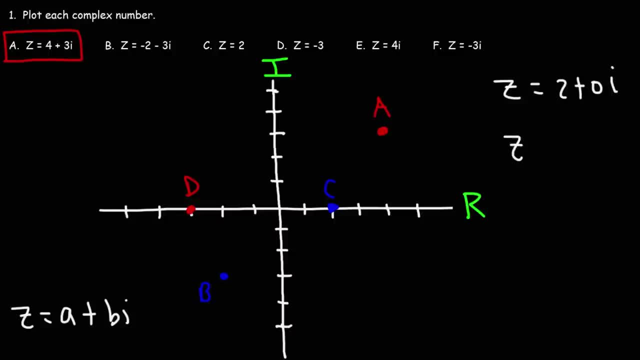 with that Now for e, z is equal to 4i. you can view this as 0 plus 4i, So a is 0, b is 4.. So think of it as plotting the point 0 comma 4.. 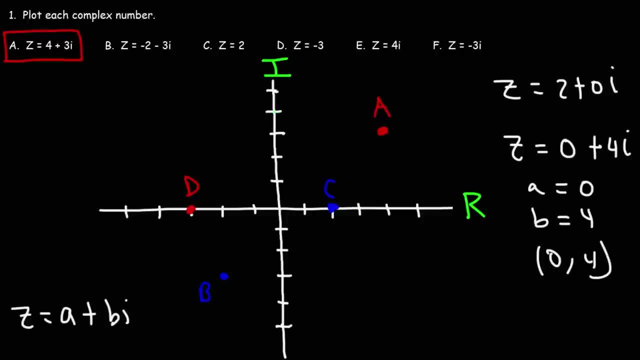 This is going to be on the y axis, So that's going to be over here. So that's point e. Now f, f is negative 3i, so it's going to be on the y axis or the imaginary axis, but at negative 3.. 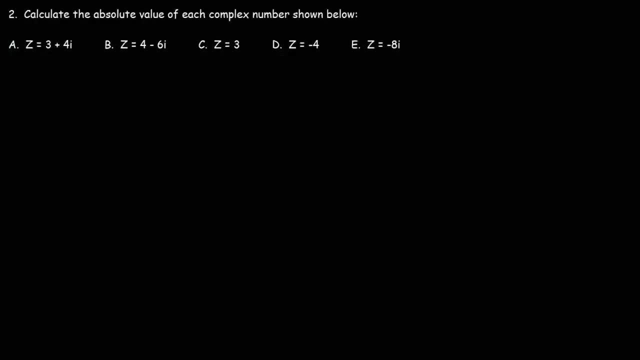 So this is point f. Now let's move on to the next problem. Calculate the absolute value of each complex number shown below. So the absolute value of z, which is the absolute value of a plus bi, that's equal to the square root of a squared plus b squared. 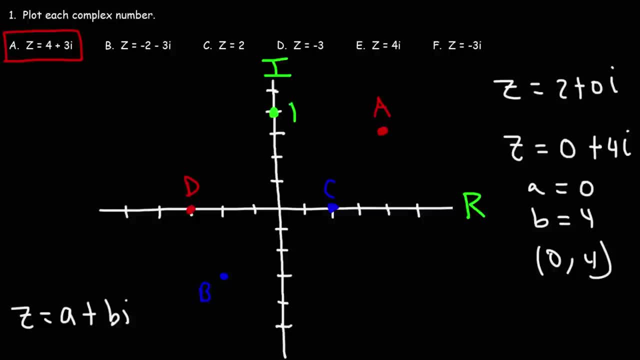 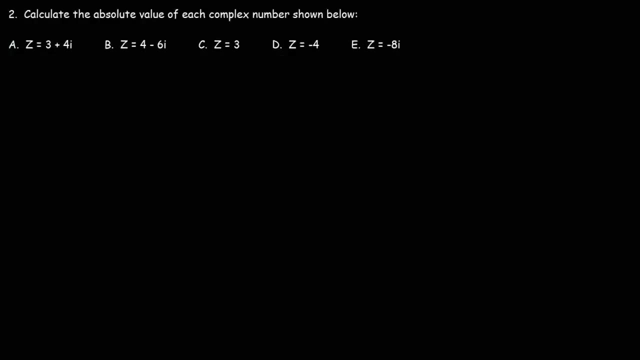 over here. So that's point e. Now f: f is negative 3i, so it's going to be on the y axis or the imaginary axis, but at negative 3.. So this is point f. Now let's move on to the next problem. 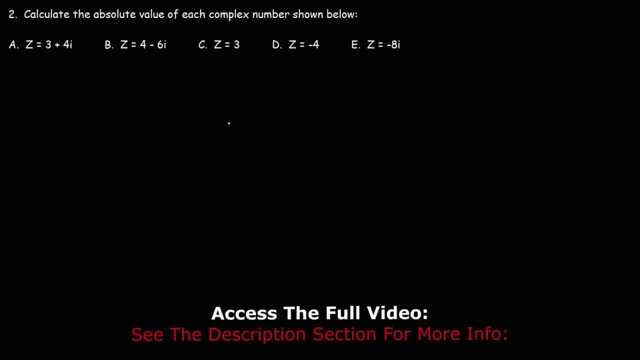 Calculate the absolute value of each complex number shown below. So the absolute value of z, which is the absolute value of a plus b, i, that's equal to the square root of a squared plus b squared. So let's focus on part a, The absolute. 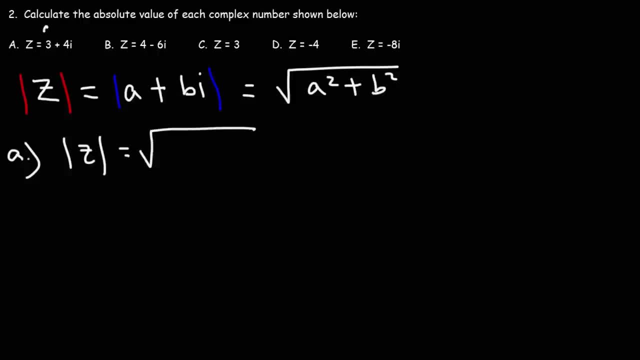 value of z is going to be the square root of. a is 3, b is 4.. So this is the square root of 3 squared plus 4 squared. 3 squared is 9,, 4 squared is 16.. The sum of those two is 25. 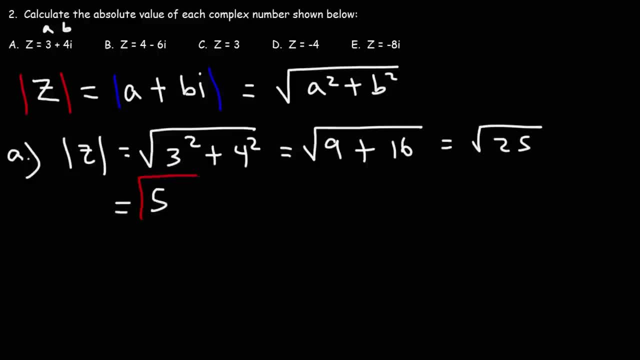 and the square root of 25 is 5.. So that's the answer for part a. For part b, the absolute value of z equals 4 minus 6i. that's going to be the square root of 4 squared plus negative 6 squared. 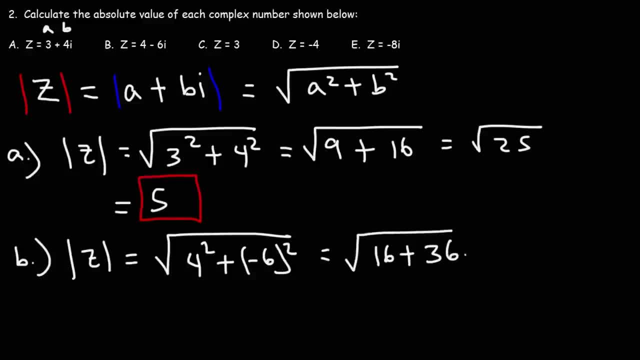 4 squared is 16. negative 6 squared is positive 36. 16 plus 36 is 52.. Now we could simplify this: radical 52 is 4 times 13 and the square root of 4 is 2.. So the answer for part b is: 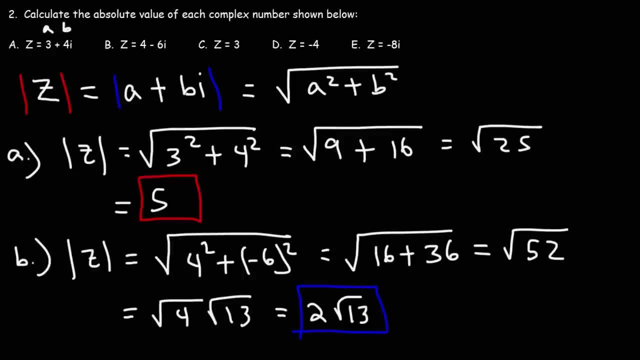 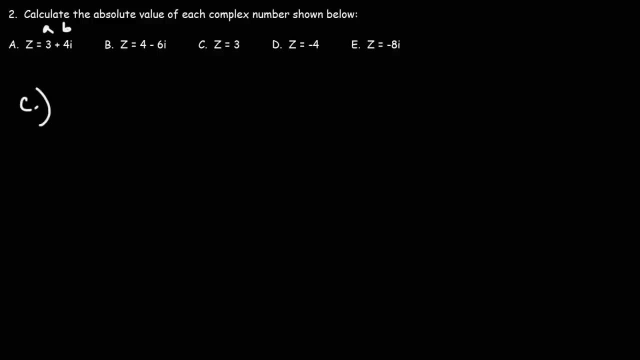 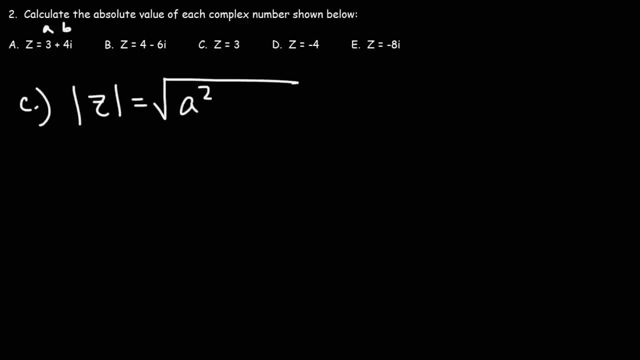 So what's the absolute value of that? So we're going to use the formula a squared plus b squared. a squared plus b squared z equals 3 can be rewritten as 3 plus 0i, as 3 plus 0i, So a is 3. 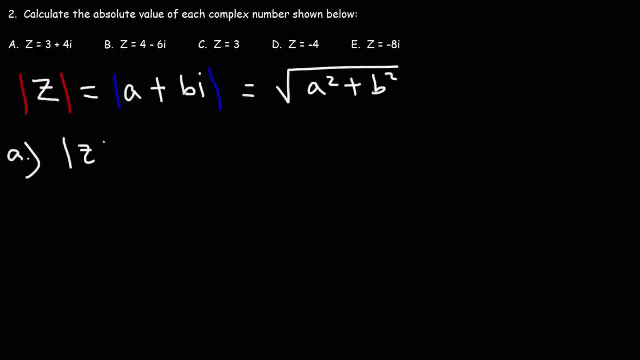 So let's focus on part a. The absolute value of z is going to be. the square root of a is 3, b is 4.. So this is the square root of 3 squared plus 4 squared. 3 squared is 9,. 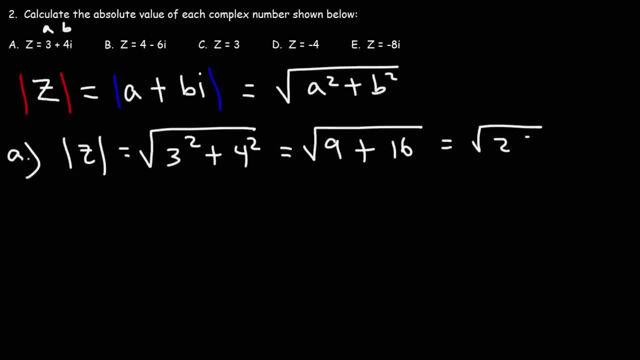 4 squared is 16.. The sum of those two is 25 and the square root of 25 is 5.. So that's the answer for part a. For part b, the absolute value of z equals 4 minus 6i. 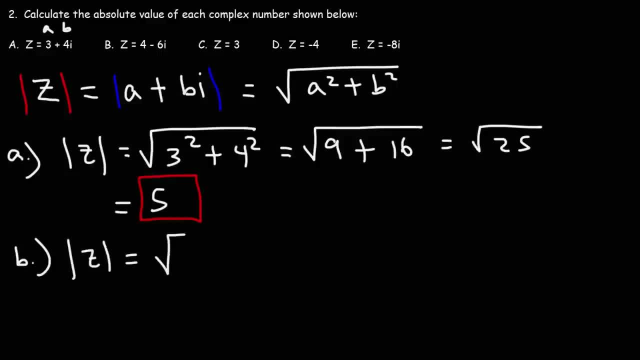 that's going to be the square root of 4 squared plus negative 6 squared. 4 squared is 16.. Negative 6 squared is positive 36.. 16 plus 36 is 52.. Now we could simplify this: radical 52 is: 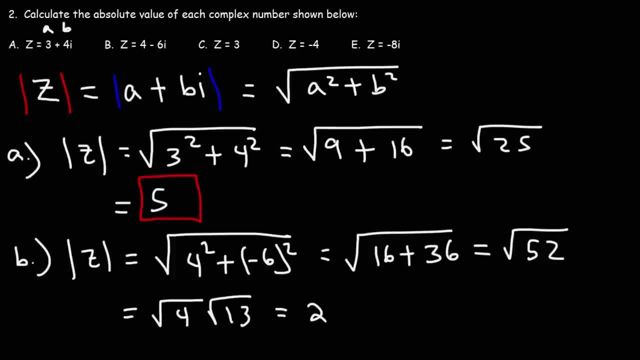 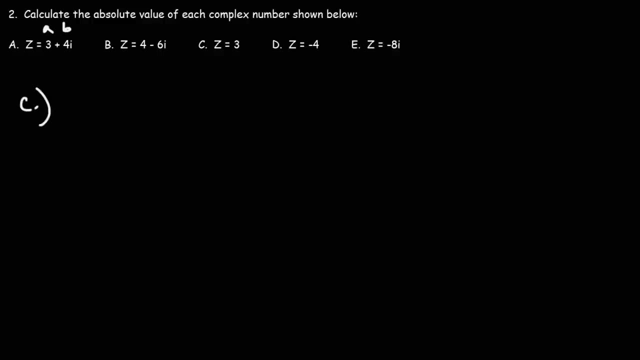 4 times 13.. And the square root of 4 is 2.. So the answer for part b is 2 square root 13.. Now let's move on to part c. z is equal to 3.. So what's the absolute value of? 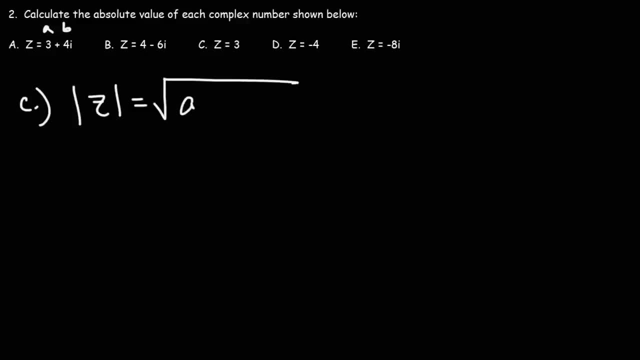 that. So we're going to use the formula: a squared plus b squared z equals 3, can be rewritten as 3 plus 0i, So a is 3, b is 0. So this is the square root of 3 squared plus. 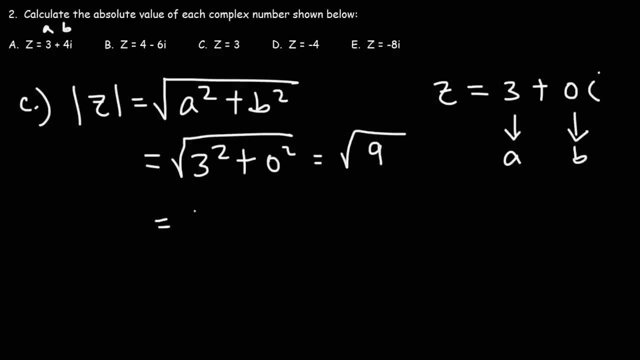 0 squared, 3 squared is 9 and the square root of 3, I mean the square root of 9- is 3.. So the answer is just 3.. Now let's move on to part d. So we have: z is equal to negative 4.. 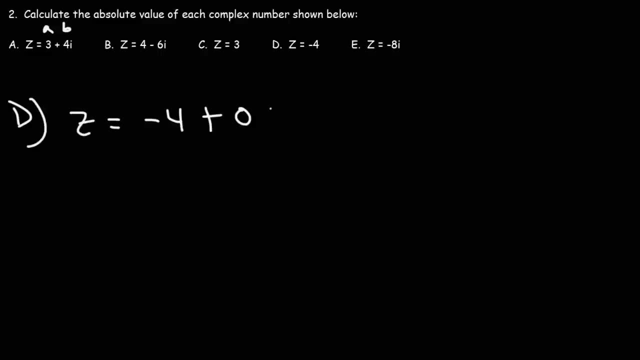 So we're going to rewrite this as negative 4 plus 0i, So we can see that a is negative 4.. b is 0.. So once you identify a and b, you can use the formula. So this is going to be negative 4 squared. 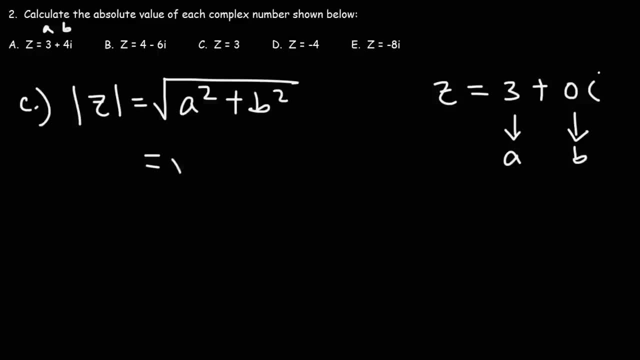 b is 0.. So this is the square root of 3 squared plus 0 squared. 3 squared is 9 and the square root of 3- I mean the square root of 9- is 3.. So the answer is just 3.. 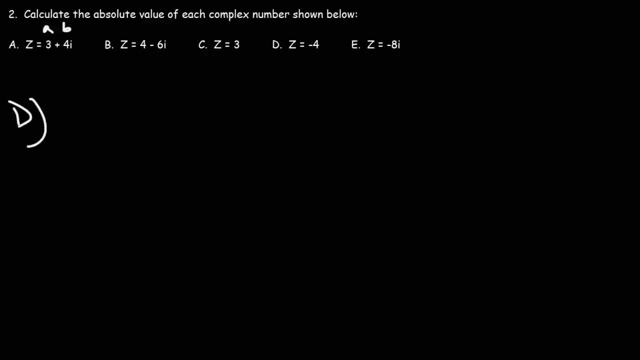 Now let's move on to part d. Now let's move on to part d. So we have: z is equal to negative 4.. So we're going to rewrite this as negative 4 plus 0i, So we can see that a is negative 4. 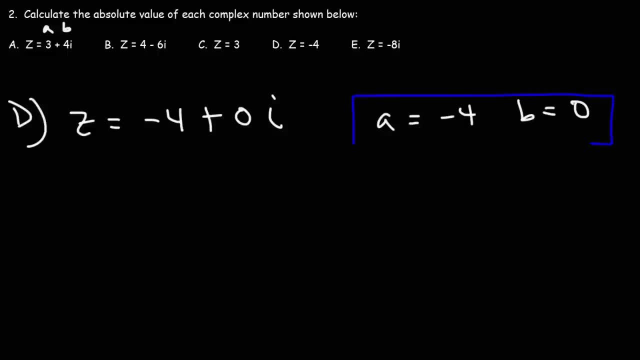 b is 0.. So once you identify a and b, you can use the formula. So this is going to be negative 4 squared plus 0 squared. negative 4 squared is 16 and the square root of 16 is positive 4.. 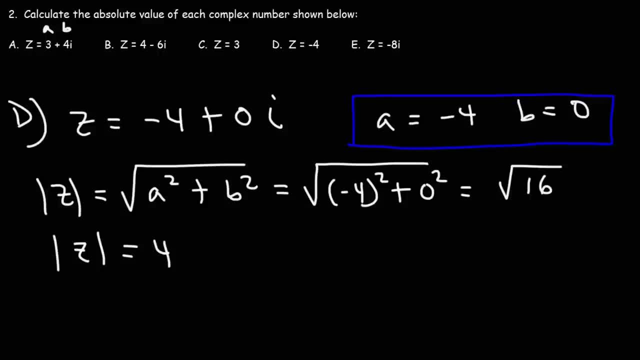 So whenever you're finding the absolute value of a complex number, you're going to find that the final answer is going to be positive. So keep that in mind. Now let's move on to part e. So we have: z is equal to negative 8i. 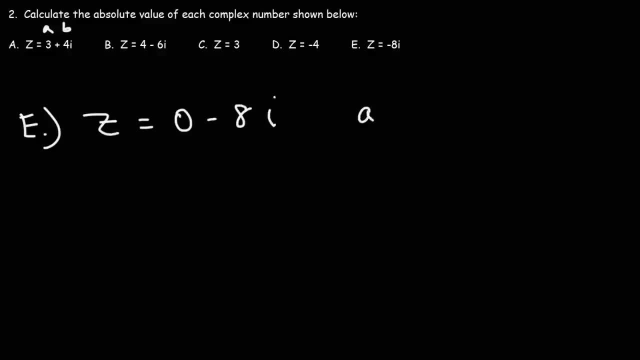 So this is 0 minus 8i. So a is 0, b is negative 8. So to find the absolute value of z that's going to be the square root of a squared plus b squared, a is 0, b is negative 8. 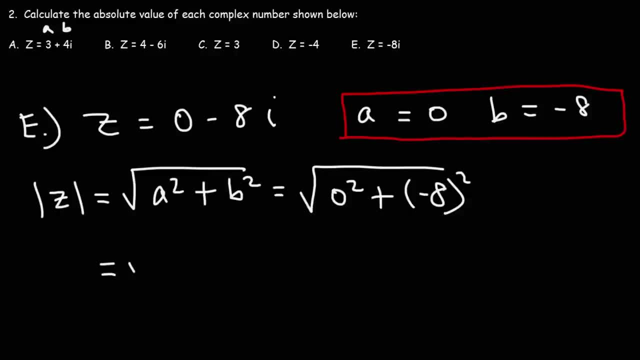 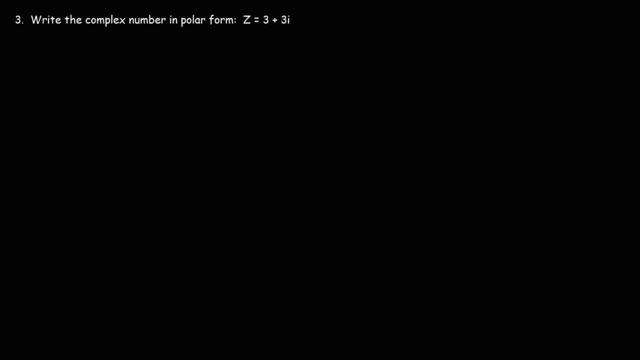 negative 8 squared is going to be positive 64, and the square root of 64 is 8.. So the final answer is simply positive 8.. So that's how you can find the absolute value of each complex number shown below. So now you have a systematic way of doing this. 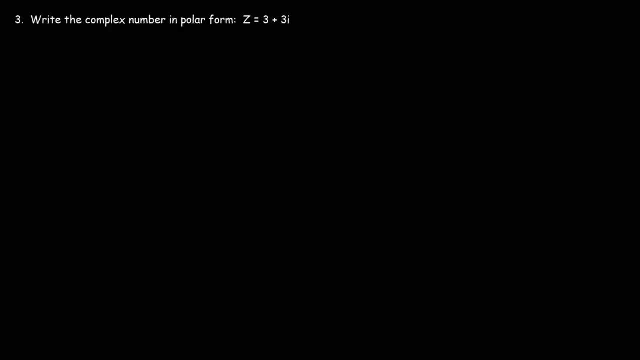 Number 3. So we're given z in rectangular form, that is, in a plus bi form, and we want to convert it to its polar form, that is, in this form, z is equal to r cosine theta plus i sine theta. So all we need to do is: 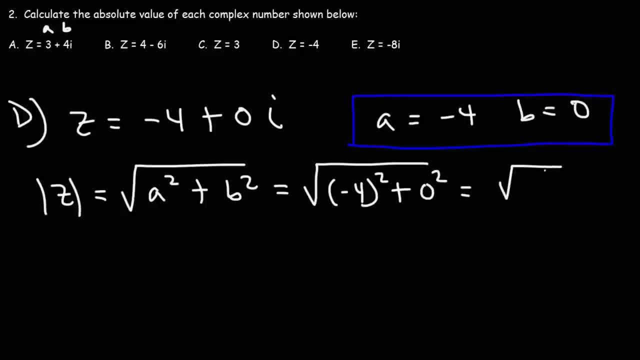 plus 0, squared Negative 4, squared is 16 and the square root of 16 is positive 4.. So whenever you're finding the absolute value of a complex number, your final answer is going to be positive, So keep that in mind. 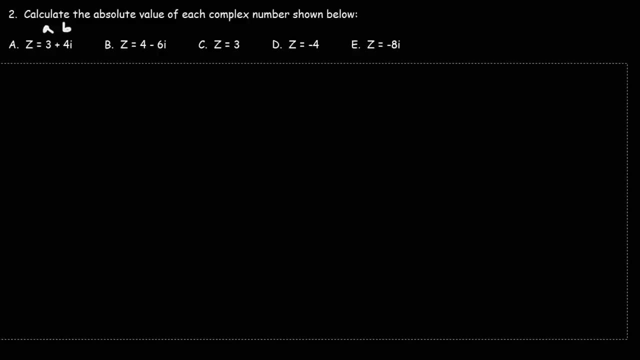 Now let's move on to part e. So we have: z is equal to negative 8i. So this is 0 minus 8i. So a is 0.. b is negative 8.. So to find the absolute value of z, that's going to be the square root. 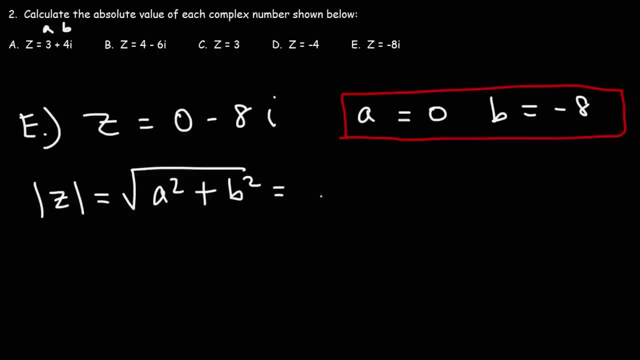 of a squared plus b squared, a is 0.. b is negative 8.. Negative 8 squared is going to be positive 64. And the square root of 64 is 8.. So the final answer is simply positive 8.. So that's how you. 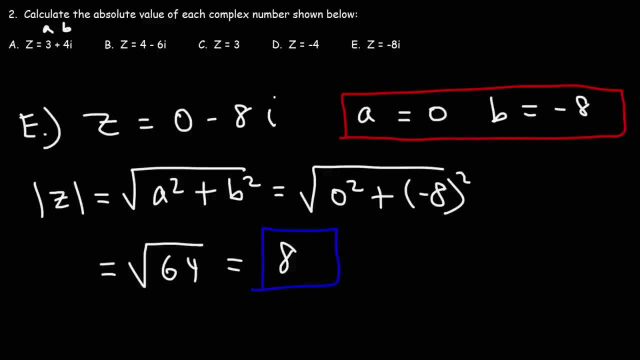 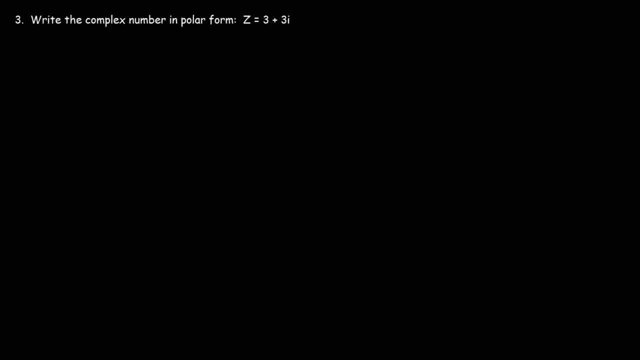 can find the absolute value of each complex number shown below. So now you have a systematic way of doing this Number 3. Write the complex number in polar form. So we're given z in rectangular form, That is, in a plus bi form. 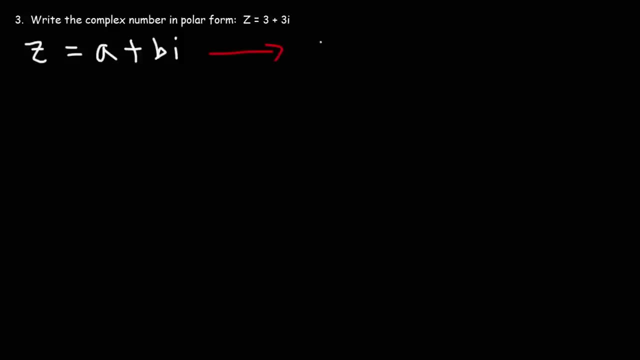 And we want to convert it to its polar form, That is, in this form, z is equal to r cosine theta plus i sine theta. So all we need to do is find the values of r and theta, And then we can write it in polar form. 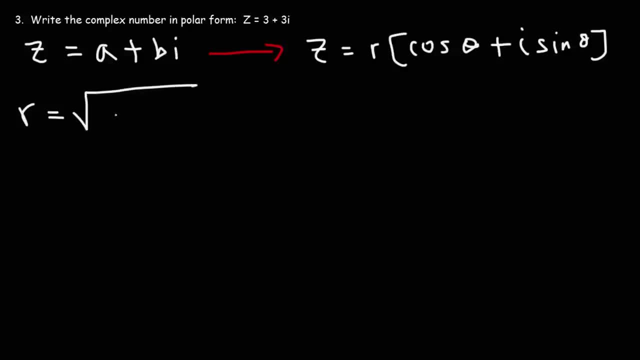 So we know that r is going to be the square root of a squared plus b squared. So this is the square root of 3 squared plus 3 squared. 3 squared is 9.. 9 plus 9 is 18.. So we've got to simplify. 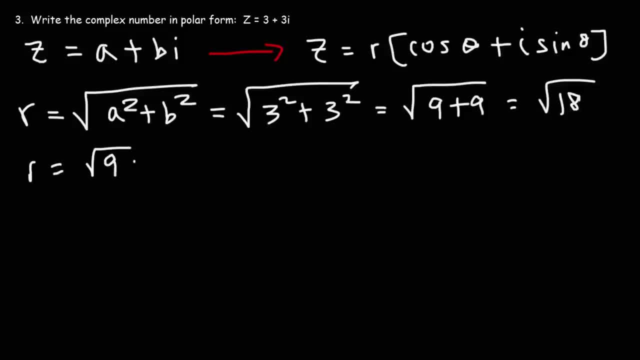 the square root of 18.. 18 is 9 times 2. And the square root of 9 is 3.. So r is square root of 2.. Now we need to calculate theta. So first let's draw a picture. 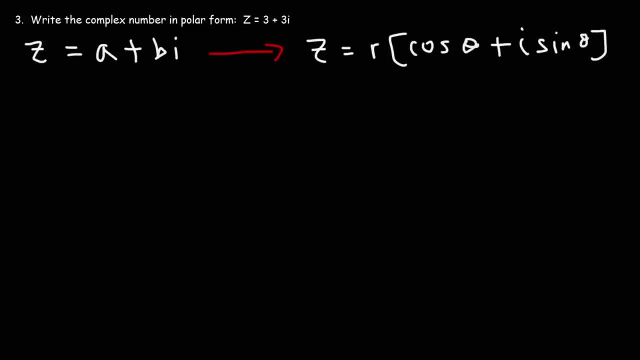 find the values of r and theta and then we can write it in polar form. So we're given z in rectangular form. So we know that r is going to be the square root of a squared plus b squared, So this is the square root of 3 squared plus. 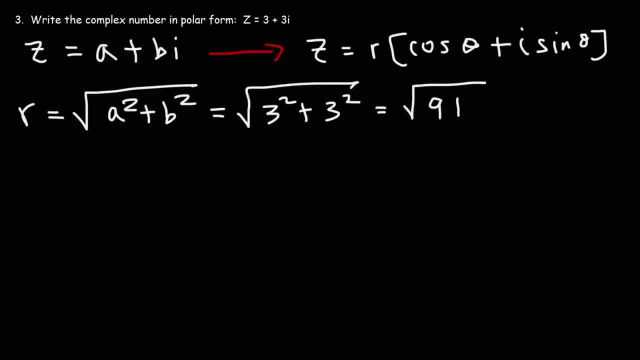 3 squared. 3 squared is 9. 9 plus 9 is 18. So we got to simplify the square root of 18: 18 is 9 times 2 and the square root of 9 is 3.. So r is 3. 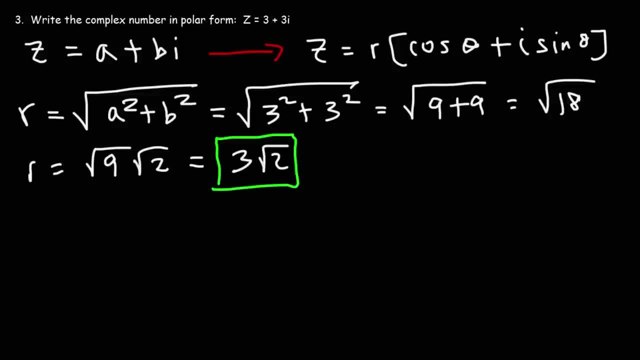 square root 2. Now we need to calculate theta. So first let's draw a picture. a is 3, so we're going to travel 3 units to the right. b is 3, so we're going to go up 3 units and we're going to make a triangle. 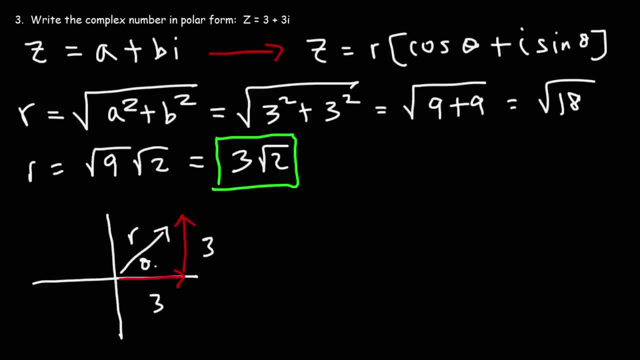 So this is our r value and this is theta. To get the reference angle of the triangle, we could use this formula: It's going to be r tangent b over a. b is 3, a is 3, So this is going to be r tangent of 1. 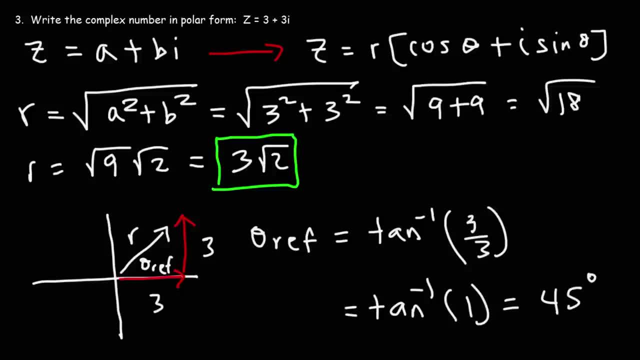 r tan of 1 is 45. Now this formula gives you the reference angle. Now in quadrant 1 the reference angle is going to be the same as the angle that we want. So in our quadrants we need to adjust the angle relative to the positive x axis. 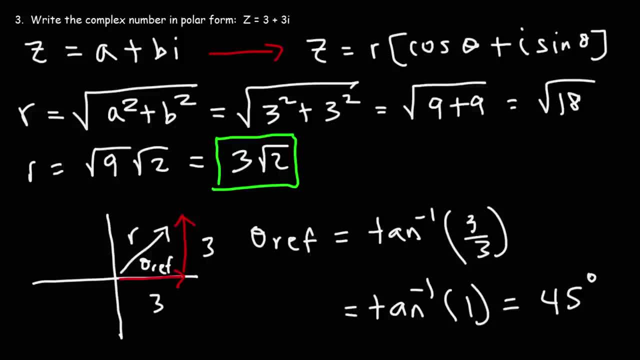 Now I'm going to give you some examples on that. So now that we know theta, we can write our answer. So theta is 45 degrees. So to write the complex number in polar form using this formula, simply replace r and theta. So we're going to replace r with. 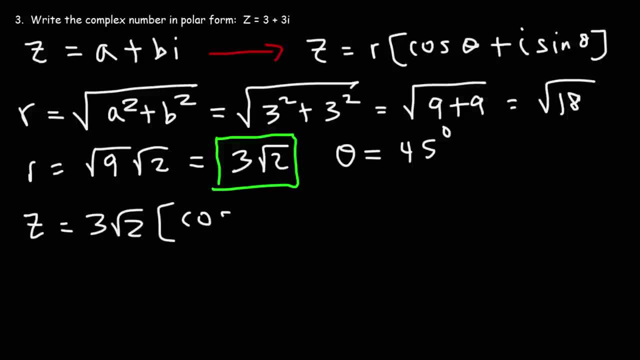 3 square root 2, and we're going to replace theta with 45 degrees. Now, sometimes your final answer will be in radians as opposed to degrees, So we're going to convert it to radians as well. To do that, take your angle in degrees and multiply it by pi. 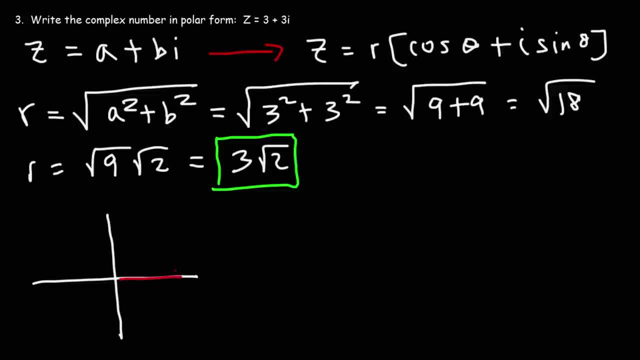 a is 3.. So we're going to travel 3 units to the right. b is 3.. So we're going to go up 3 units And we're going to make a triangle. So this is our r value and this is theta. 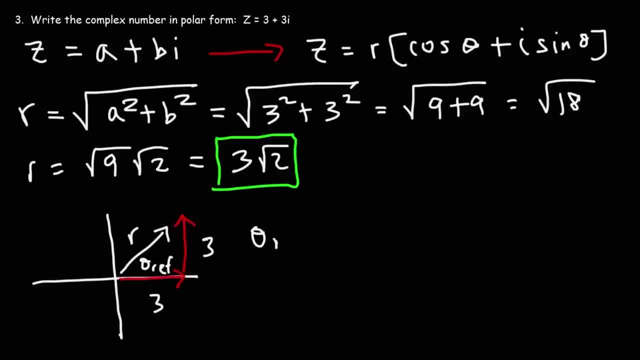 To get the reference angle of the triangle, we could use this formula. It's going to be arctangent b over a. b is 3.. a is 3.. So this is going to be arctangent of 1.. arctan of 1 is 45.. 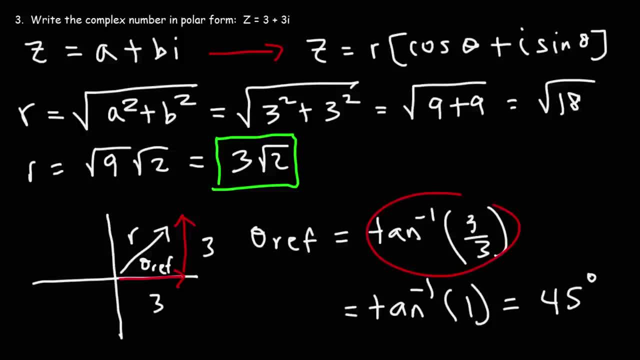 Now this formula gives you the reference angle. Now in quadrant 1 the reference angle is going to be the same as the angle that we want. But in other quadrants we need to adjust the angle relative to the positive x-axis, And I'm going to give you some examples on that. 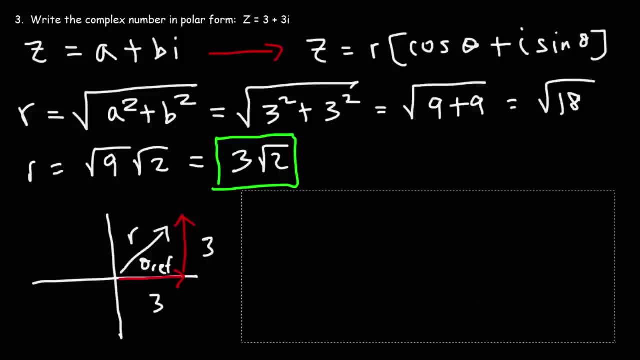 So now that we know theta, we can write our answer. So theta is 45 degrees. So to write the complex number in polar form using this formula, simply replace r and theta. So we're going to replace r with 3 square root 2.. 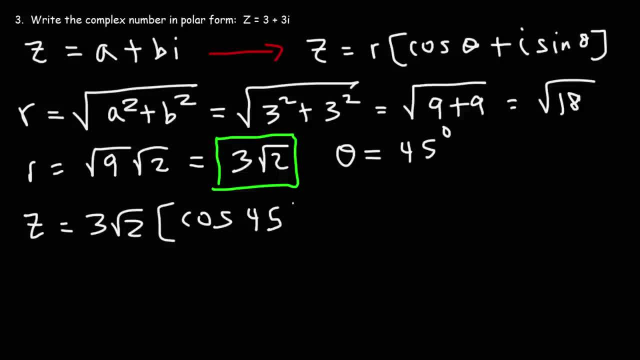 And we're going to replace theta with 45 degrees. Now, sometimes your final answer will be in radians as opposed to degrees, So we're going to convert it to radians as well. To do that, take your angle in degrees and multiply it by pi. 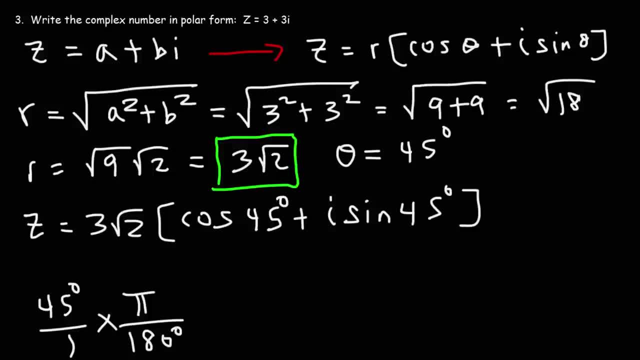 over 180.. 180 divided by 45 is 4.. So this turns out to be pi over 4.. Another way in which you can show your work is you can write it like this: You can break down 180 into 45 times 4.. 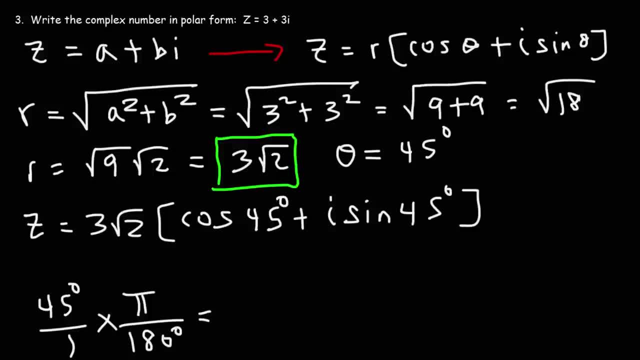 over 180. 180 divided by 45 is 4, So this turns out to be pi over 4. Another way in which you can show your work is you can write it like this: You can break down 180 into 45 times 4, And so: 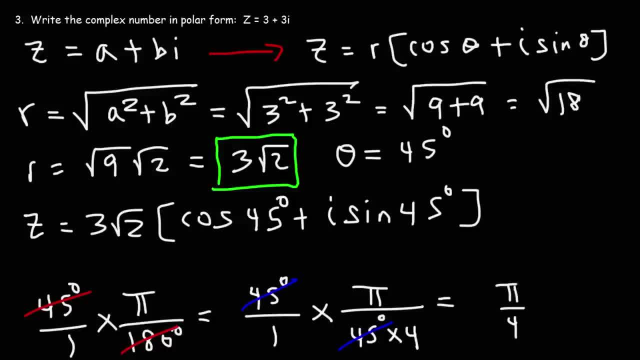 45 degrees will cancel giving you pi over 4. So we can write our final answer like this: So we can write our final answer like this: 3 square root 2 times cosine pi over 4 plus i sine pi over 4. So that's how we can convert. 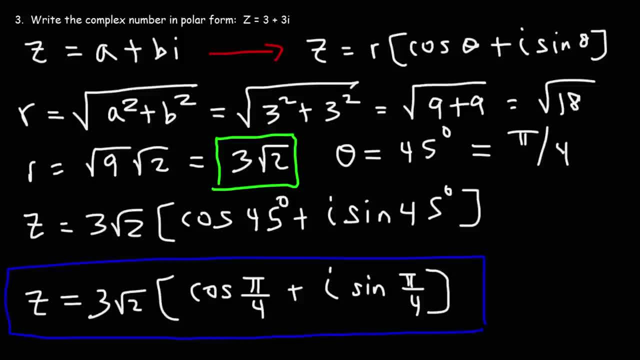 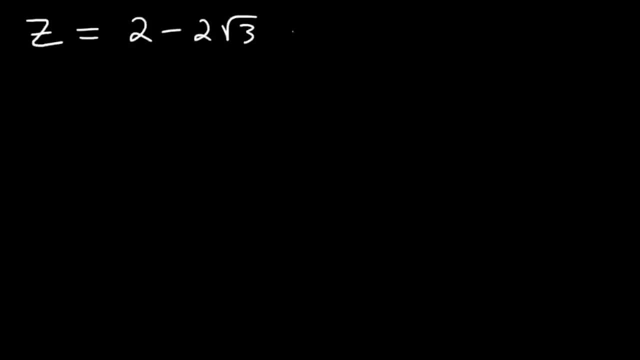 a complex number from rectangular form to polar form. Now let's work on some more examples. Let's say z is equal to 2 minus 2 root 3. i Go ahead and try this one. Find r and then find theta. Now you want to find the angle. 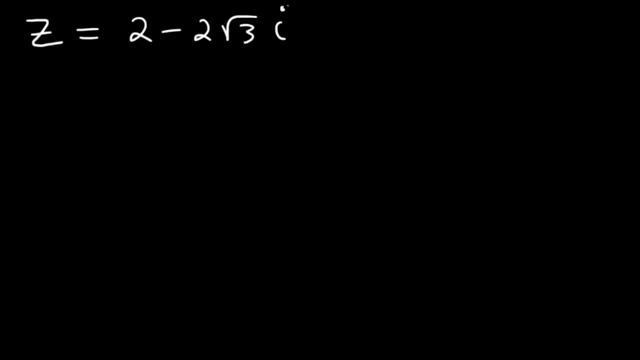 relative from the positive x-axis, Not just the reference angle. So let's start with r. r is going to be the square root of a squared. where a is 2 and b squared, b is going to be 2 root 3. Now, what is 2 root 3 squared? 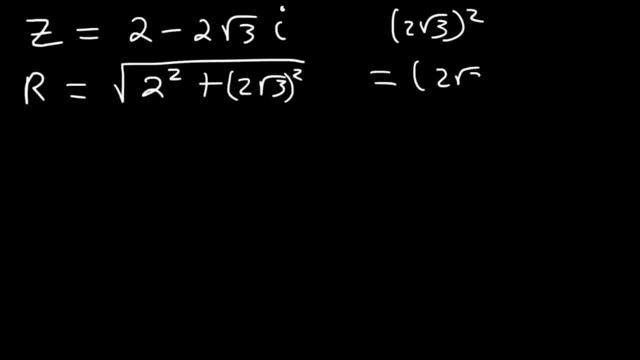 Now what is 2 root 3 squared? So that's basically 2 root 3 times 2, root 3 2 times 2 is 4 and root 3 times root 3 is the square root of 9, which is 3. 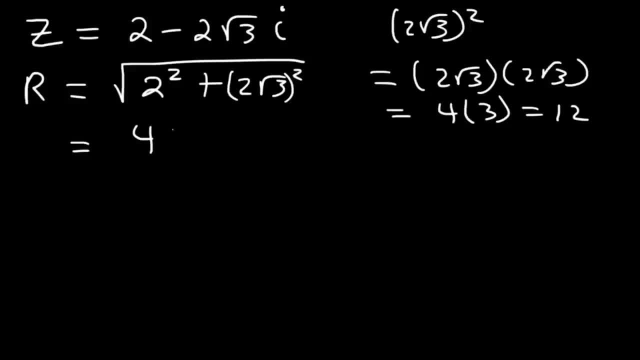 and 4 times 3 is 12, 2 squared is 4 and 2 root 3 squared is 12. 4 plus 12 is 16. So we get the square root of 16. So r is 4. So now that we have the value of r, 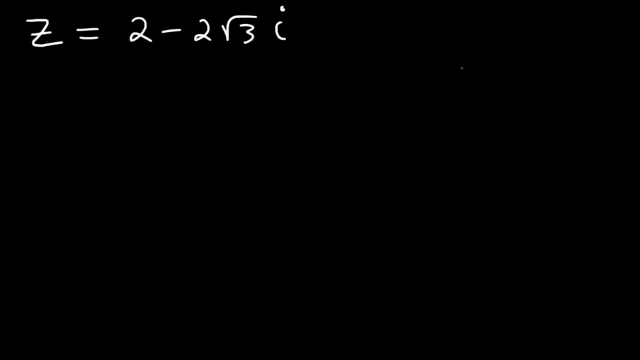 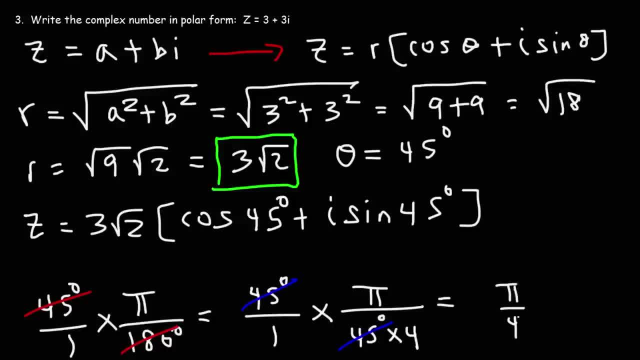 And so 45 degrees will cancel giving you pi over 4.. So we can write our final answer like this: 3 square root, 2 times cosine pi over 4, plus i sine pi over 4.. So that's how we can convert. 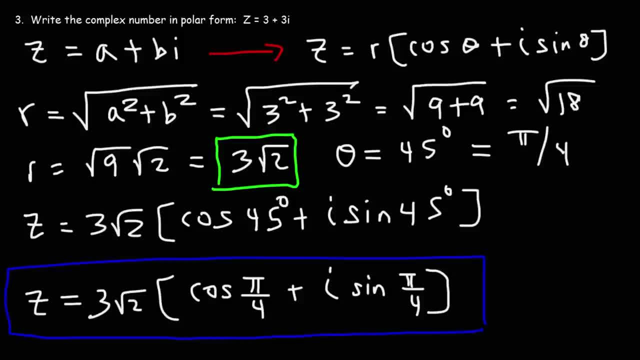 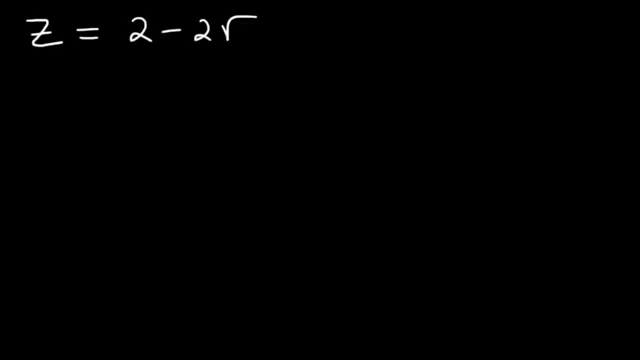 a complex number, from rectangular form to polar form. Now let's work on some more examples. Let's say z is equal to 2 root 3. i Go ahead and try this one. Find r and then find theta. Now you want to find the angle. 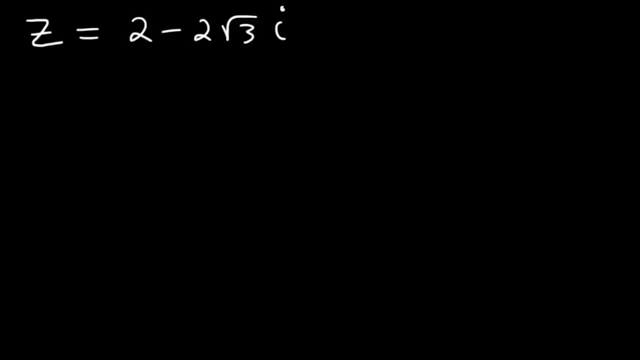 relative from the positive x axis, Not just the reference angle. So let's start with r. r is going to be the square root of a squared. where a is 2 and b squared, b is going to be 2 root 3.. Now what is? 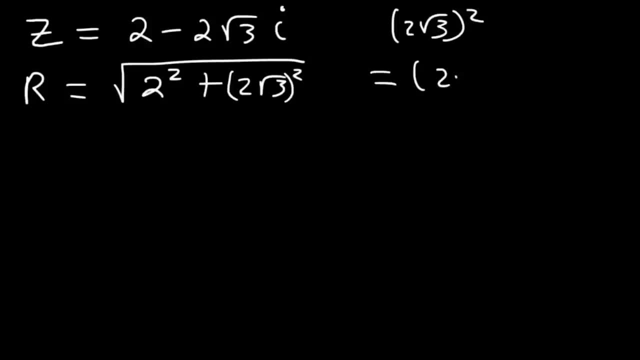 2 root 3 squared, So that's basically 2 root 3 times 2 root 3.. 2 times 2 is 4, and root 3 times root 3 is the square root of 9, which is 3.. 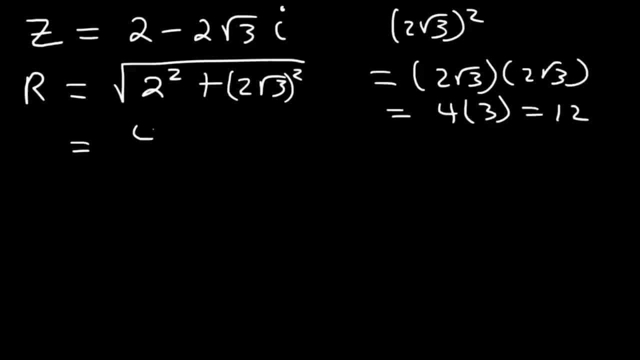 And 4 times 3 is 12.. 2 squared is 4 and 2 root 3 squared is 12.. 4 plus 12 is 16.. So we get the square root of 16, so r is 4.. 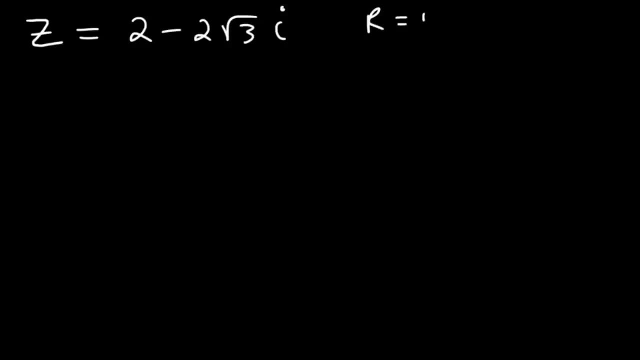 So, now that we have the value of r, let's find a reference angle. to begin with, To find a reference angle, which is the angle inside the triangle. when you use this equation, make sure that a and b are positive. So in this example, b, even though it's negative. 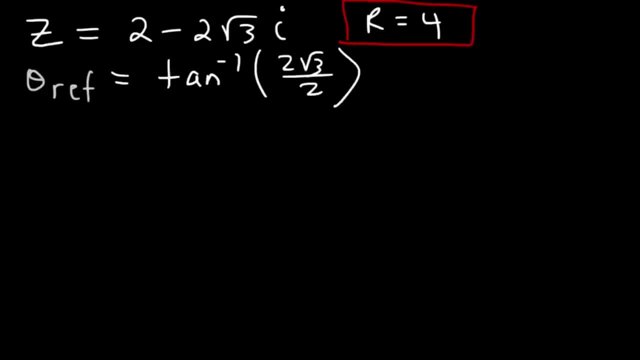 2 root 3, I'm going to use positive 2 root 3 in the equation, And a is 2.. So what we're looking for is the arc tangent of root 3.. If you type that in your calculator, make sure it's in degree mode. 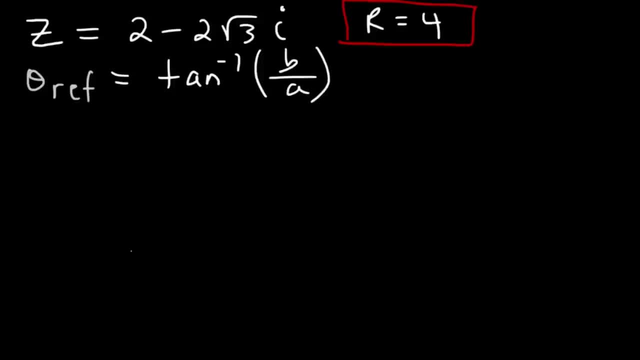 When you use this equation, make sure that a and b are positive. So in this example b, even though it's negative, 2 root 3, I'm going to use positive 2 root 3 in the equation and a is 2, So what we're looking for. 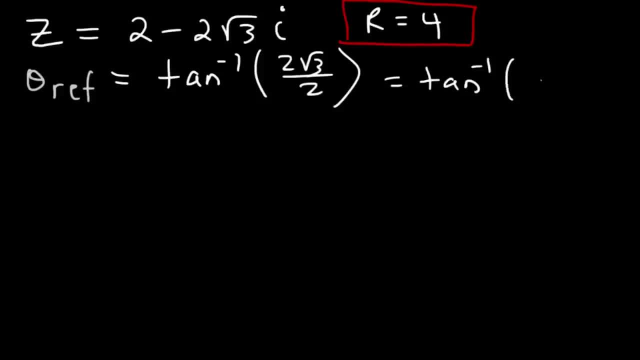 is the arc tangent of root 3 of root 3. If you type that in your calculator, make sure it's in degree mode. You should get 60 degrees. That's the reference angle. Now z is not in quadrant 1, So the final answer is not 60 degrees. 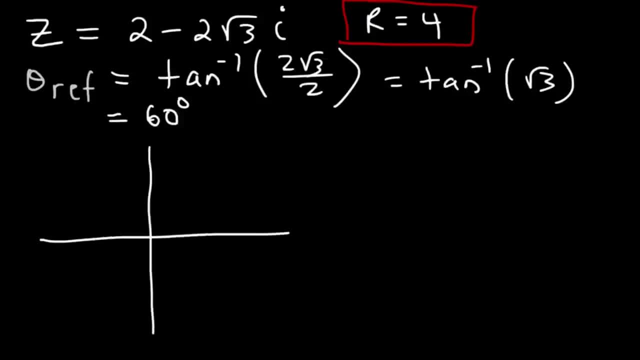 is not 60 degrees. Notice that a is positive, which is directed towards the right in the positive x axis, but b is negative. So therefore, r is in quadrant 4. r is in quadrant 4, So this is positive 2 and this is negative 2. root 3: 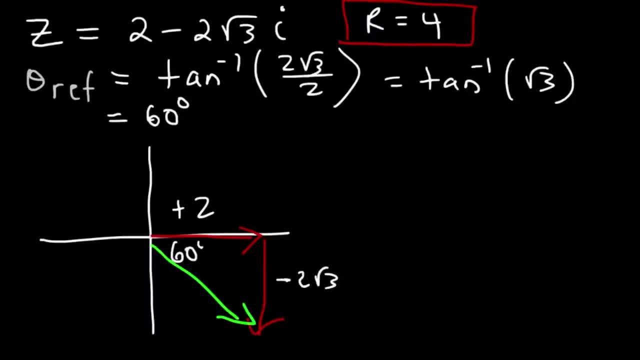 and this is negative 2 root 3. Now the reference angle is the angle inside the triangle, but we want the angle measured from the positive x axis, So that's 360 minus 60, which is 300. That's the angle that we want to report. 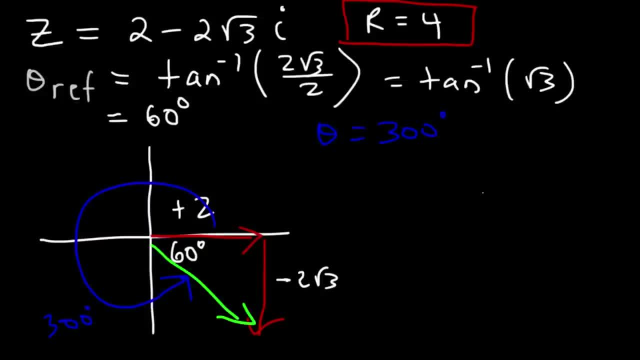 Now here's some notes that you may want to keep in mind. Let's say: if r is in quadrant 1, Define the angle as the reference angle. You don't need to change it. In quadrant 2, your angle has to be between 90 and 180. 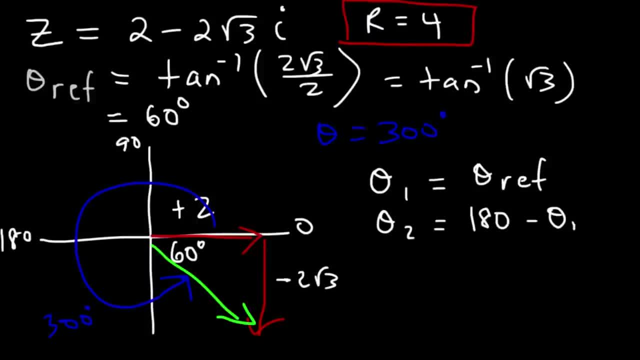 So the angle in quadrant 2 is 180 minus the reference angle. If r is in quadrant 2, the angle is going to be 180 plus the reference angle, And any time r is in quadrant 4, it's going to be 360 minus the reference angle. 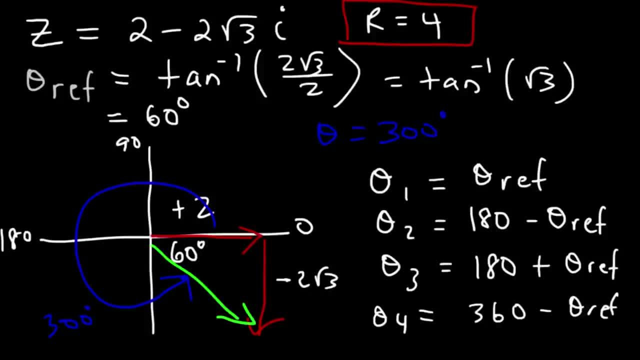 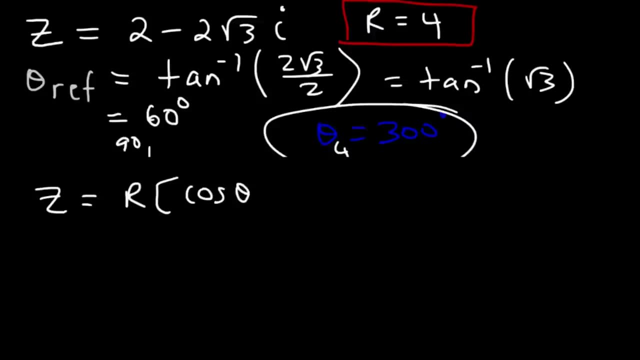 which is what we did- 360 minus 60- and that gave us this angle, which is 300. So now we can write our final answer in polar form. So, using the equation, z is equal to r cosine theta plus i sine theta z is going to be: 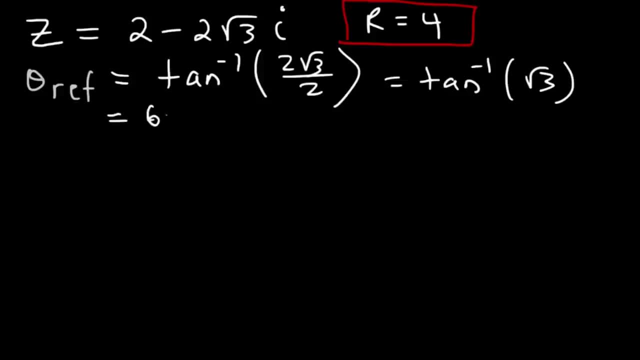 you should get 60 degrees. That's the reference angle. Now z is not in quadrant 1, so the final answer is not 60 degrees. Notice that a is positive, which is directed towards the right in the positive x-axis, But b is negative. 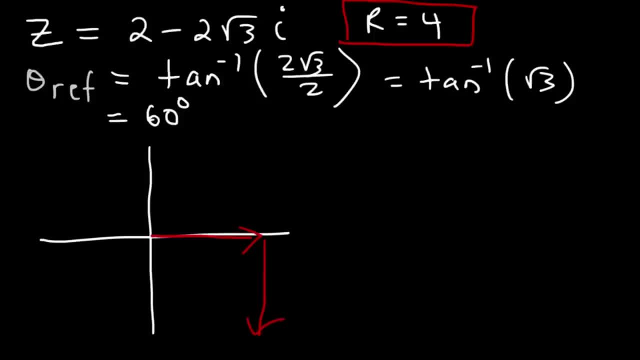 so therefore, r is in quadrant 4.. So this is positive 2 and this is negative 2 root 3.. Now the reference angle is the angle inside the triangle, That's 60. But we want the angle measured from the positive x-axis. 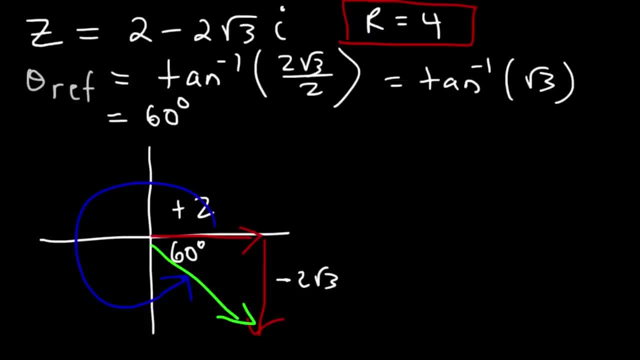 So that's 360 minus 60, which is 300.. That's the angle that we want to report. Now here's some notes that you may want to keep in mind. Let's say if r is in quadrant 1.. To find the angle is the same. 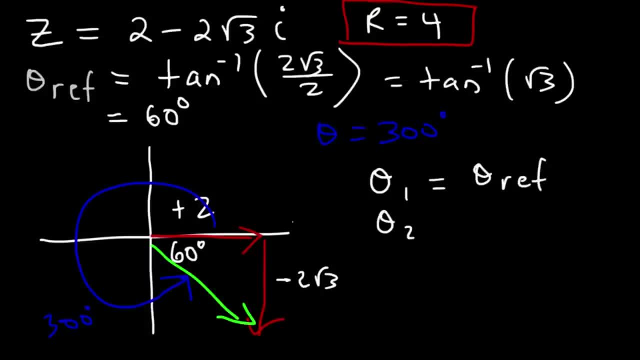 as the reference angle. You don't need to change it. In quadrant 2 your angle has to be between 90 and 180.. So the angle in quadrant 2 is 180 minus the reference angle If r is in quadrant 3. 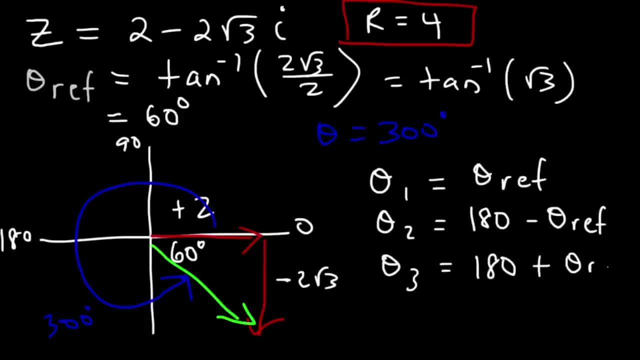 the angle is going to be 180 plus the reference angle And anytime r is in quadrant 4, it's going to be 360 minus the reference angle, Which is what we did- 360 minus 60- and that gave us this angle, which is 300. 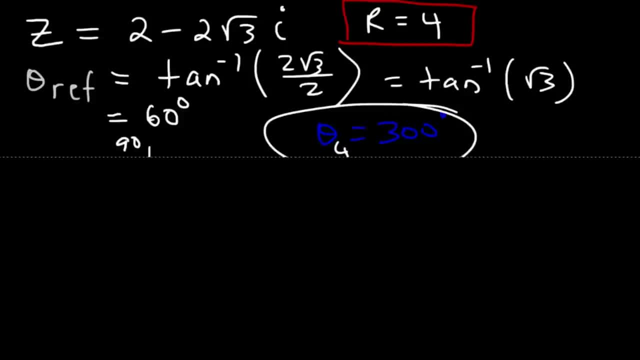 So now we can write our final answer in polar form. So, using the equation, z is equal to r cosine theta plus i sine theta. z is going to be 4 cosine 300 plus i sine 300. And if we want to write it in radians, 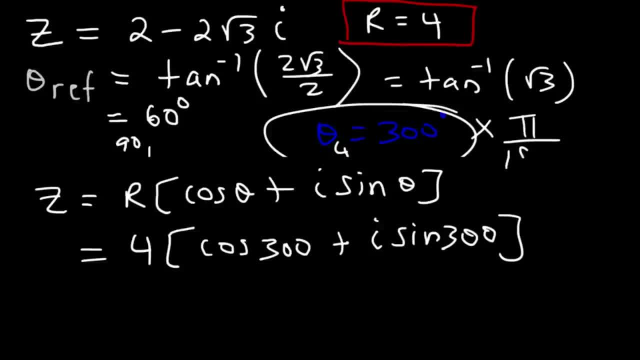 let's convert 300.. So let's multiply it by pi divided by 180.. So we can cancel with 0.. So we have 30 pi over 18.. 30 is basically 6 times 5.. 18 is 6 times 3.. 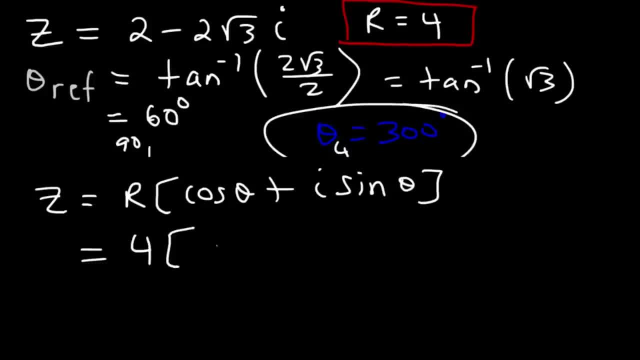 4, cosine 300 plus i sine 300 plus i sine 300 plus i sine 300. And if we want to write it in radians, let's convert 300. So let's multiply it by pi divided by 180, So we can cancel with 0. 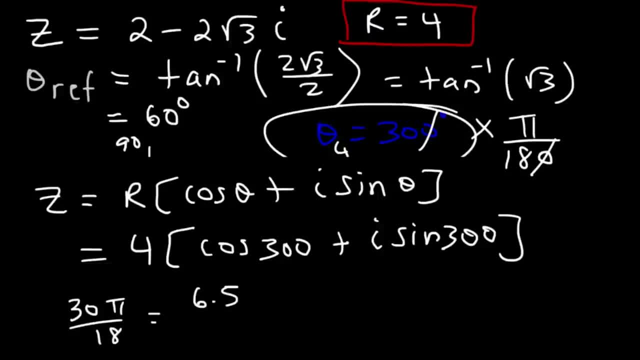 So we have 30 pi over 18. 30 is basically 6 times 5, 18 is 6 times 3, So we can get rid of 6. So therefore 300 degrees is 5 pi over 3. So this can be written as: 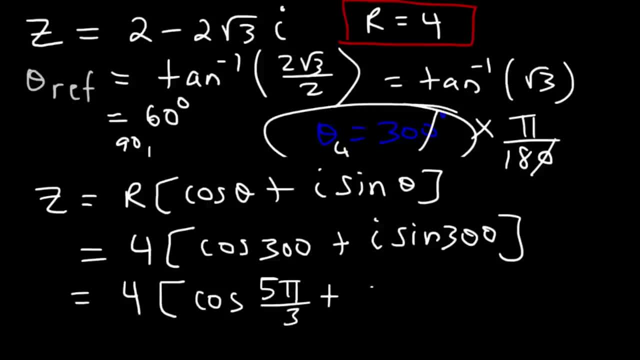 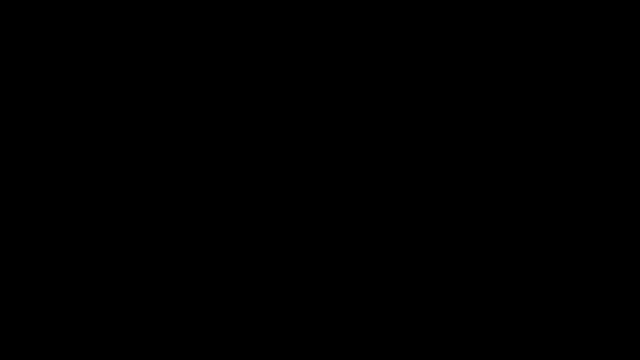 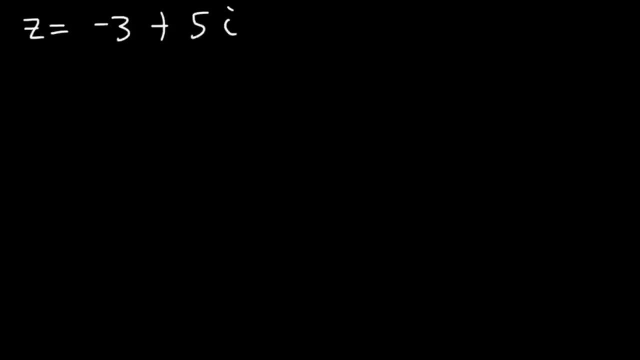 Let's say z is equal to negative 3 plus 5i. Go ahead and convert it into its polar form. Take a minute, pause the video and try this problem. So let's start by finding r. r is the square root of a squared plus b squared. 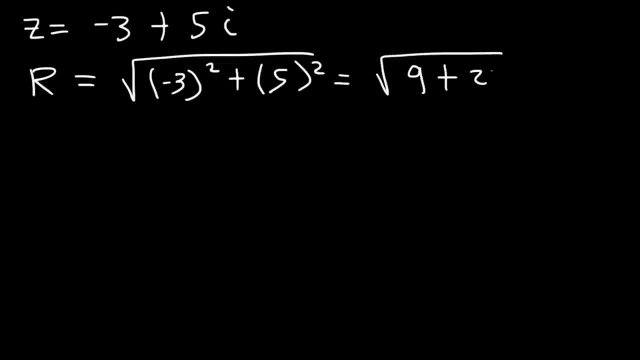 So negative: 3 squared is 9 plus 5 squared is 25. 9 plus 25 is 34, and we can't simplify root 34 because there's no perfect square that goes into 34. All you can do is break down 34 into 2 and 17. 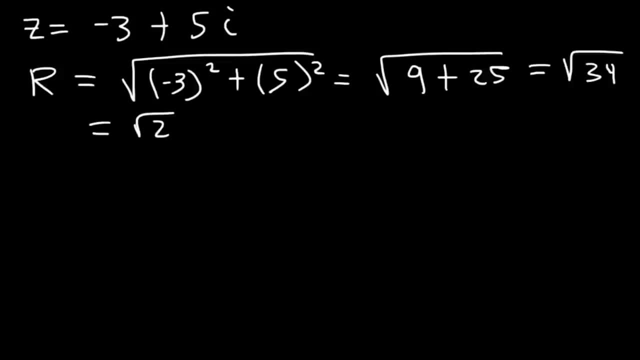 and both of these numbers are prime numbers. So now let's find the reference angle. So it's going to be arc tangent b over a, and we're just going to use the positive values of b and a. So arc tan 5 divided by 3, which is 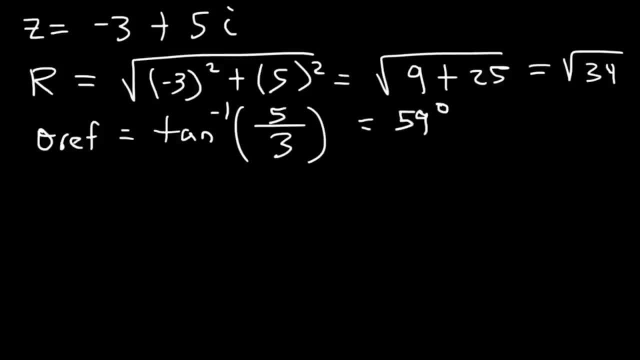 59 degrees. It's 59.03, but I'm going to round it to 59 degrees. Now let's find out what quadrant r is located in. So a is negative 3, which means we have to travel 3 units to the left, and b is positive 5. 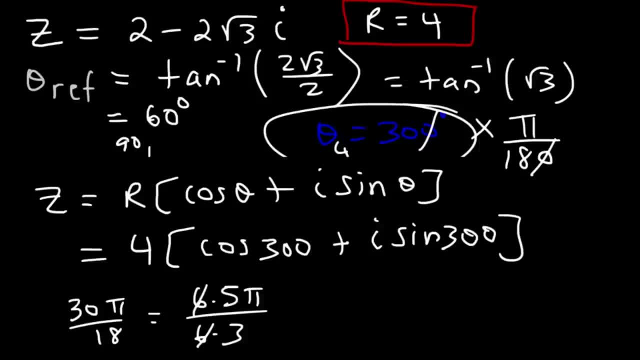 So we can get rid of the 6.. So therefore, 300 degrees is 5 pi over 3.. So this can be written as 4 cosine 5 pi over 3, plus i sine 5 pi over 3.. Here's another example. 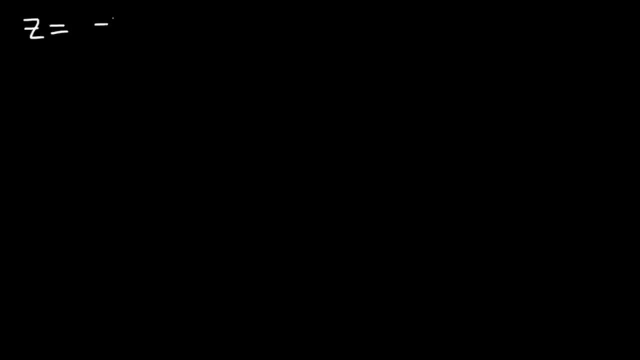 that you could try. Let's say z is equal to 3 plus 5. i Go ahead and convert it into its polar form. Take a minute, pause the video and try this problem. So let's start by finding r. r is the square root of. 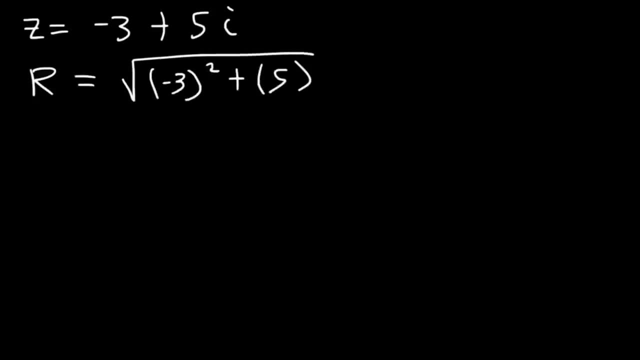 a squared plus b squared, So negative 3 squared is 9,, 5 squared is 25.. 9 plus 25 is 34.. And we can't simplify root 34, because there's no perfect square that goes into 34.. 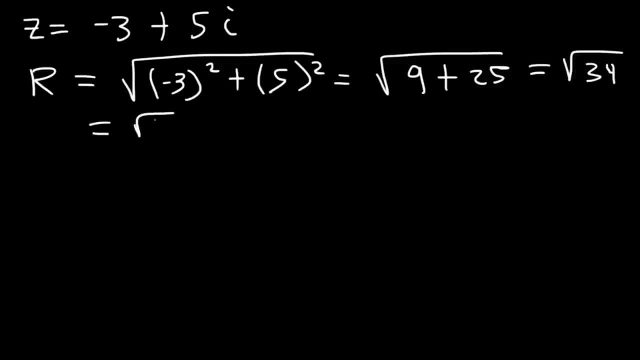 All you can do is break down 34 into 2 and 17.. And both of these numbers are prime numbers. So now let's find the reference angle. So it's going to be arc tangent b over a, And we're just going to use the positive values of b and a. 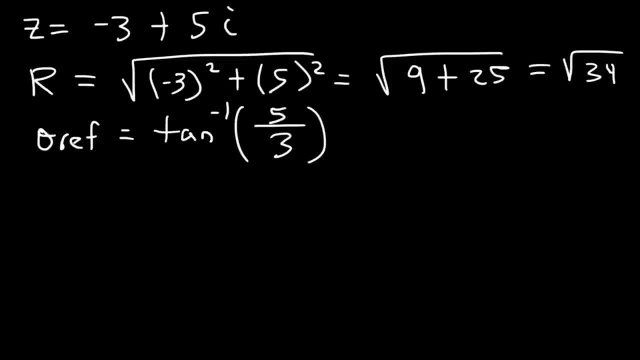 So arc tan 5 divided by 3., Which is 59 degrees. It's 59.03,, but I'm going to round it to 59 degrees. Now let's find out what quadrant r is located in. So a is negative 3.. That means we've got to travel 3 units to the left. 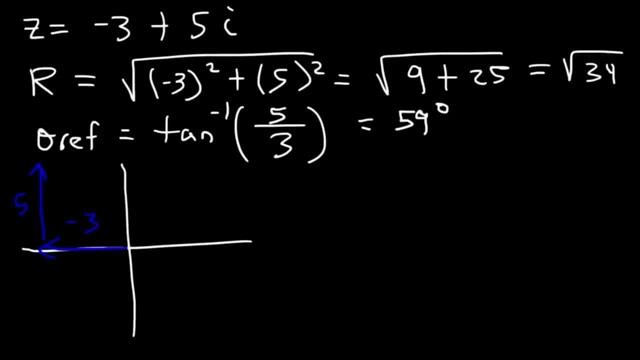 And b is positive 5.. So we've got to go up 5 units, which means r is in quadrant 2.. Any time you have r in quadrant 2, the angle is going to be 180 minus the reference angle, which is 59.. 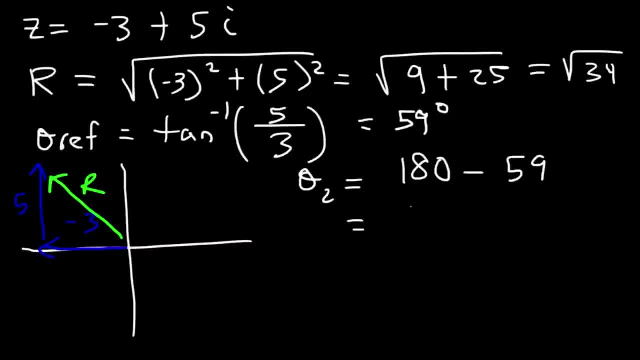 So 180 minus 59 is 121.. This is the angle that we want Relative to the positive x-axis, So that's 121.. The reference angle is inside the triangle, That's 59.. These two have to add up to 180.. 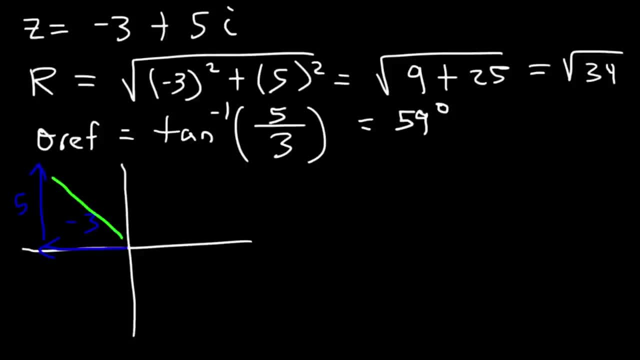 so we have to go up 5 units, which means r is in quadrant 2. Any time you have r in quadrant 2, the angle is going to be 180 minus the reference angle, which is 59. So 180 minus 59 is 121. 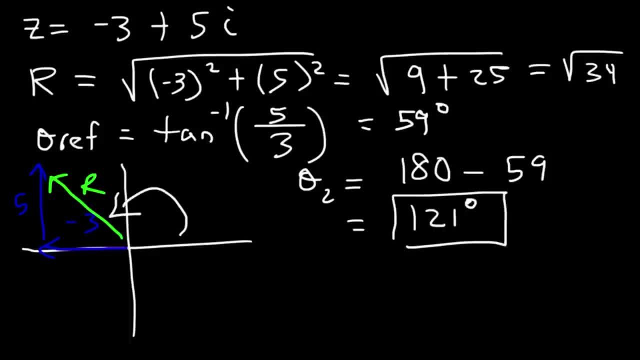 This is the angle that we want relative to the positive x-axis, So that's 121. The reference angle is inside the triangle, that's 59. These two have to add up to 180, which is a straight line. So now that we have the angle, 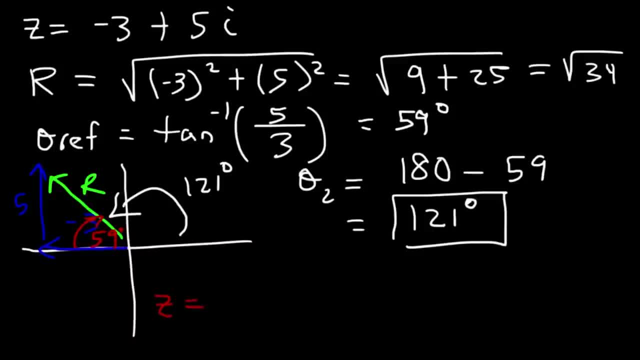 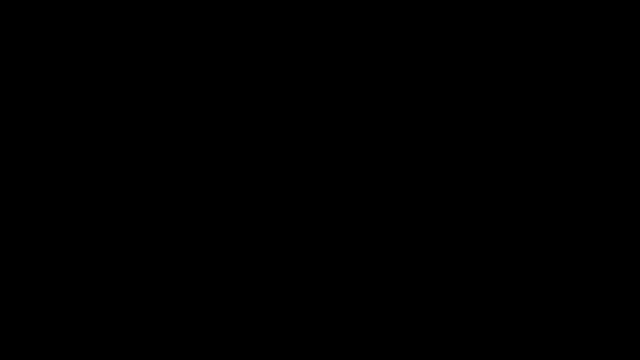 we can write our final answer in polar form. So z is equal to r, which is the square root of 34 times cosine of 121 plus i sine 121, and that's in degrees. So far we've considered examples of converting complex numbers in rectangular form to polar form. 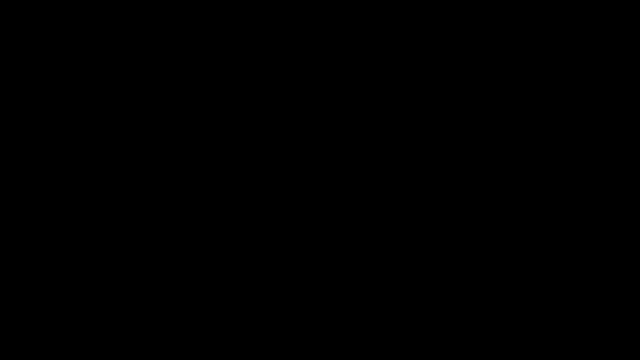 if we're given a and b? Now what if we're given a or b, but not both? What should we do? For example, let's say if z is equal to 3, How do you write that in polar form? Well, if z is equal to just one number, 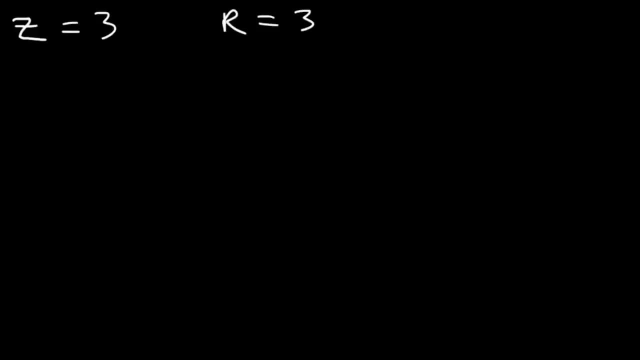 if you have a or b, only r is going to be equal to z. It's just going to be a or b by itself. So in this case r is 3. To prove it, when z is 3, it's going to be plus 0i. 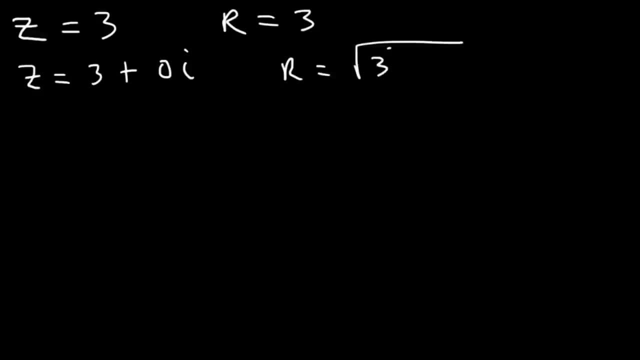 So to find r, it's going to be the square root of a squared plus b squared. 3 squared is 9 plus 0 squared, that's still going to be 9, and the square root of 9 is 3. So r is 3. 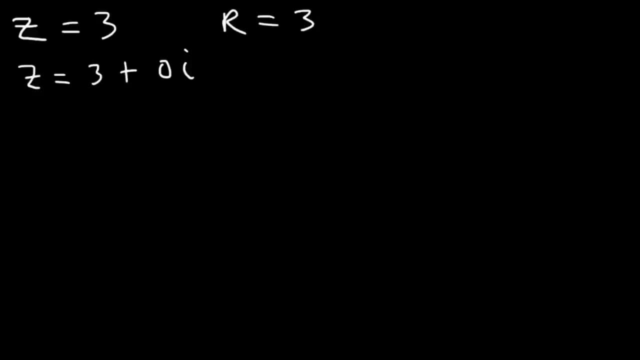 So if you're given a or b alone and the other one is 0, then z is equal to r under such circumstances. Now we need to find the angle, and it won't be wise to use the inverse tangent: y over x. you get arctan 0. 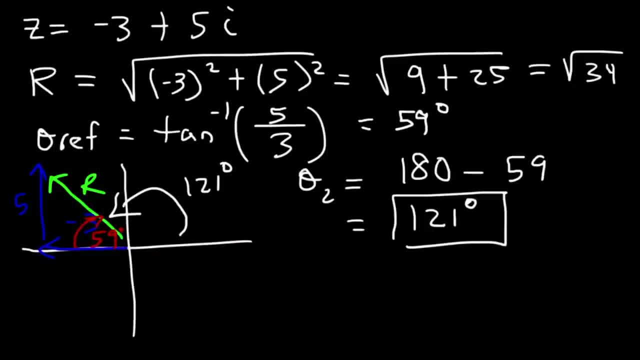 Which is a straight line. So now that we have the angle, we can write our final answer in polar form. b is equal to r, which is the square root of 34, times cosine of 121 plus i sine 121. And that's in degrees. 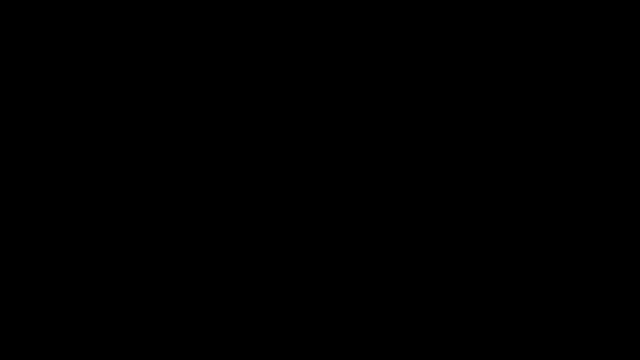 So far we've considered examples of converting complex numbers in rectangular form to polar form if we're given a and b. Now what if we're given a or b but not both? What should we do? For example, let's say if z 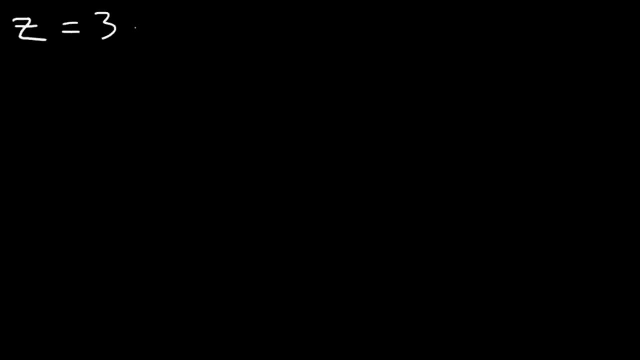 is equal to 3.. How do you write that in polar form? Well, if z is equal to just one number, if you have a or b, only r is going to be equal to z. It's just going to be a or b by itself. So in this case, r is 3.. 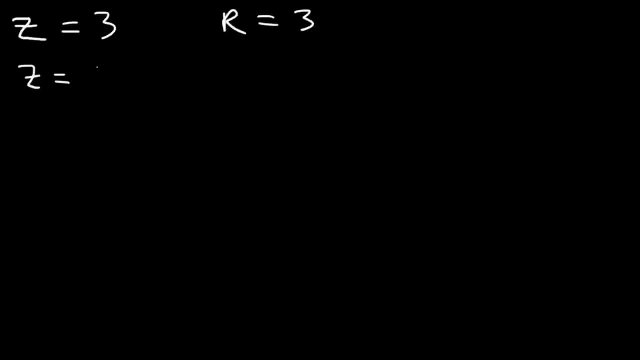 To prove it, when z is 3, it's the same as being 3 plus 0i. So to find r, it's going to be the square root of squared plus the b squared. 3 squared is 9 plus 0 squared, That's still going to be 9.. 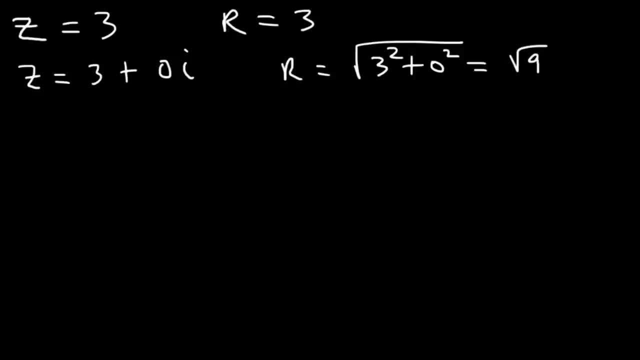 And the square root of 9 is 3.. So r is 3.. So if you're given a or b alone and the other one is 0, then z is equal to r under such circumstances. Now we need to find the angle. 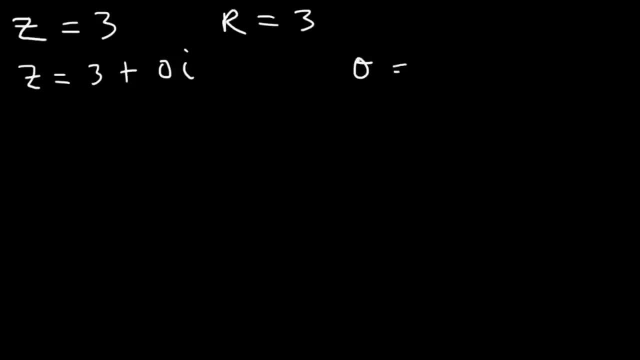 And it won't be wise to use the inverse tangent formula. If you type in inverse tangent, y over x, you get arctan 0. Which may give you the right answer. In this case it will, It's 0. But the easier 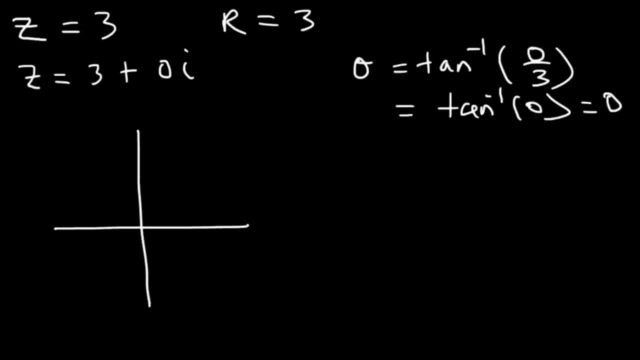 way to do it is to plot z. 3 plus 0i is on the x-axis, It's over here. So if you draw r, notice that r is 3 units long. That's why r equals 3.. And it's. 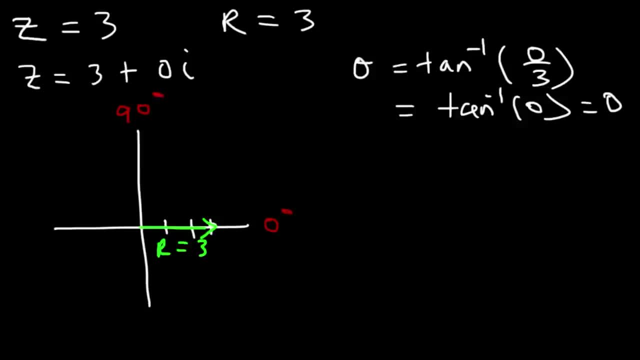 at an angle of 0 degrees. So if you have a or b and not both, the angle is either 0,, 90,, 180, or 270.. Because z is equal to positive 3,, the angle is 0 degrees. 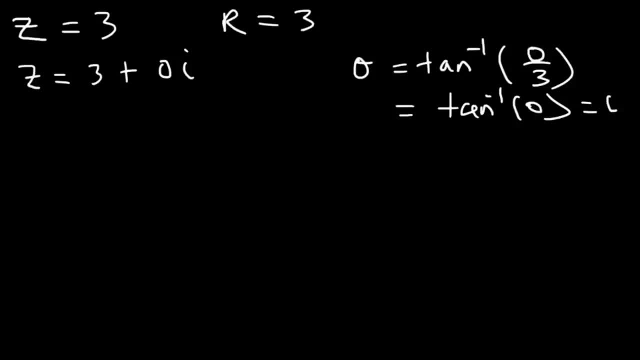 which may give you the right answer. in this case it will. it's 0, but the easy way to do it is to plot z: 3 plus 0i is on the x axis, it's over here. so if you draw r, notice that r is 3 units long. 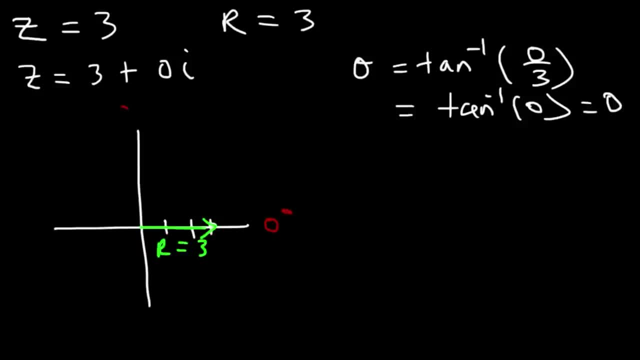 that's why r equals 3 and the angle is 0 degrees. so if you have a or b and not both, the angle is either going to be 0,, 90,, 180, or 270, because z is equal to positive 3. 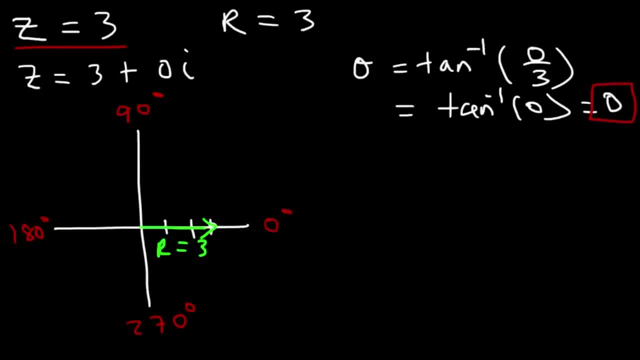 the angle is 0 degrees. so therefore we can say: z is equal to r, which is 3 times cosine of 0 degrees plus i sine of 0 degrees. so that's z in polar form. now what if z was equal to negative 4 r? 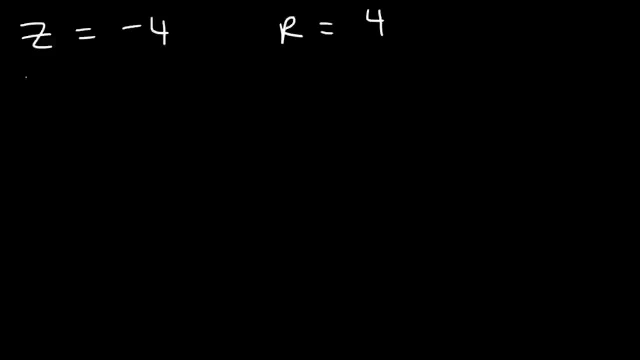 is always a positive value. that means r is equal to 4, so this is negative: 4 plus 0i. so r would be the square root of negative 4 squared plus 0 squared, which is the square root of 16, which is 4. 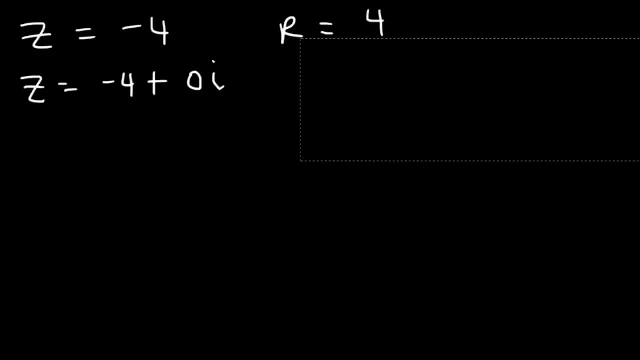 now if we try using the inverse tangent formula, if you type this in, you'll get 0 degrees, but the angle is not 0 because this time, if you plot it negative 4, 0i is on the negative x axis, it's 4 units to the left. 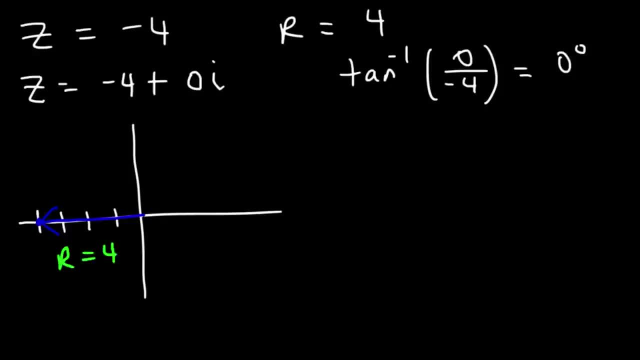 so r is 4, as you can see, but the angle is not 0, rather the angle is 180, which is on the negative x axis. so that's why this formula doesn't always work. if you have a or b, but not both, it's better to graph it. 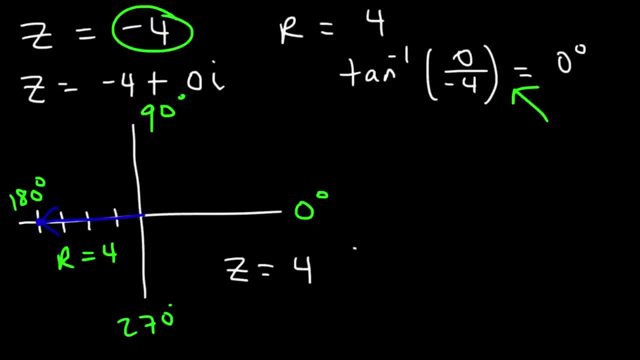 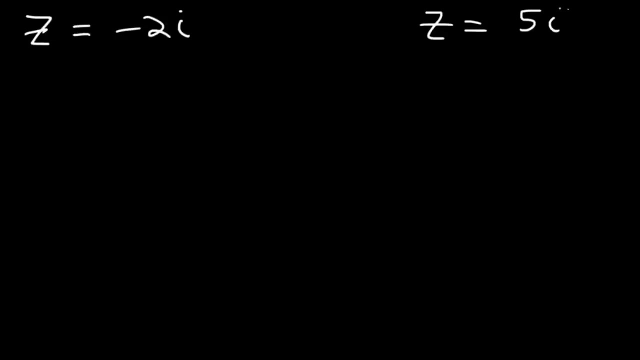 just to make sure. so the answer for this problem is 4 cosine of 180 degrees plus i sine 180 plus 1, and that's the answer. so let's try this. let's say that z is negative 2i and also that z is positive 5i. 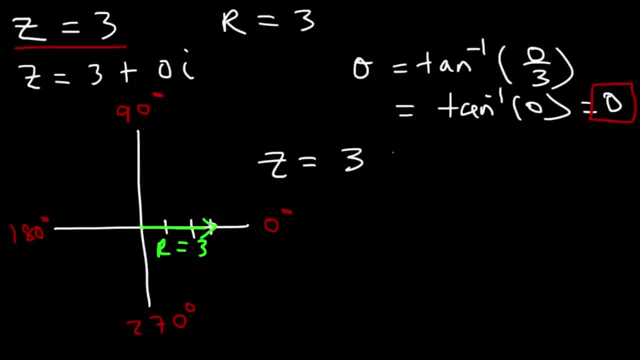 So therefore we could say: z is equal to r, which is 3, times cosine of 0 degrees, plus i sine of 0 degrees. So that's z in polar form. Now what if z was equal to negative 4?? 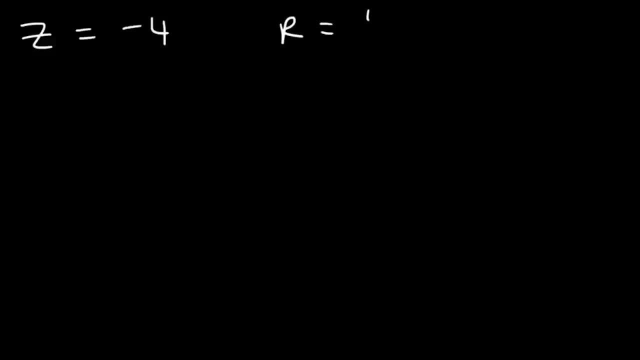 r is always a positive value. That means r is equal to 4.. So this is negative 4 plus 0i. So r would be the square root of negative 4 squared plus 0 squared, which is the square root of 16,. 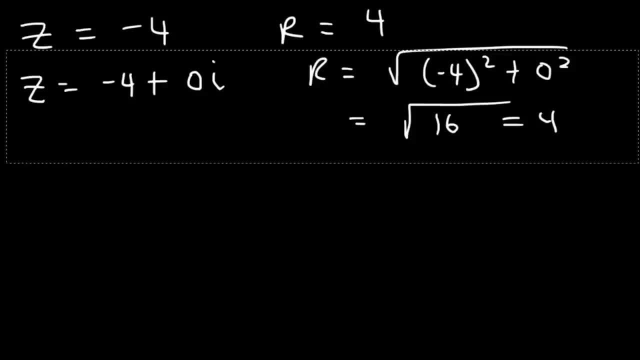 which is 4.. Now if we try using the inverse tangent formula, if you type this in, you'll get 0 degrees, But the angle is not 0. Because this time, if you plot it, negative 4, 0i is on. 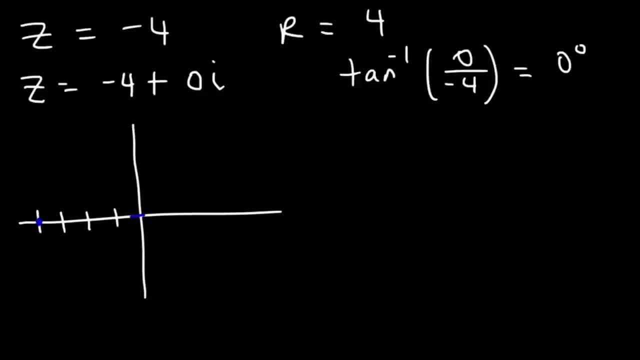 the negative x-axis, It's 4 units to the left. So r is 4, as you can see, But the angle is not 0. Rather, the angle is 180, which is on the negative x-axis. So that's why this. 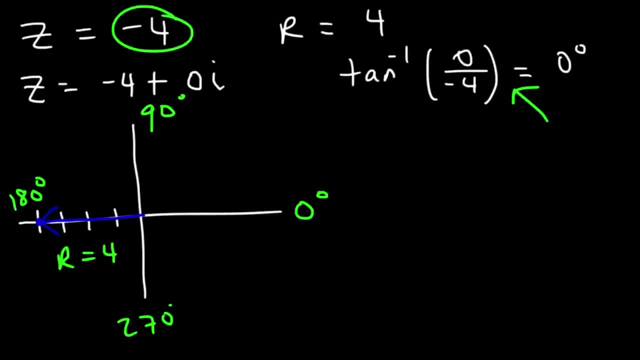 formula doesn't always work. if you have a or b but not both, It's better to graph it, just to make sure. So the answer for this problem is 4 cosine of 180 degrees plus i sine 180.. Try these two problems. Let's say that z is negative. 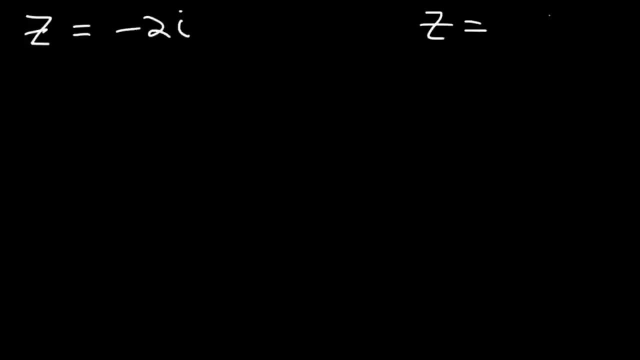 2i and also that z is positive 5i. Go ahead and try those two. So first we gotta find r. You can see that r is equal to 2.. Keep in mind z being negative. 2i is 0 minus 2i. 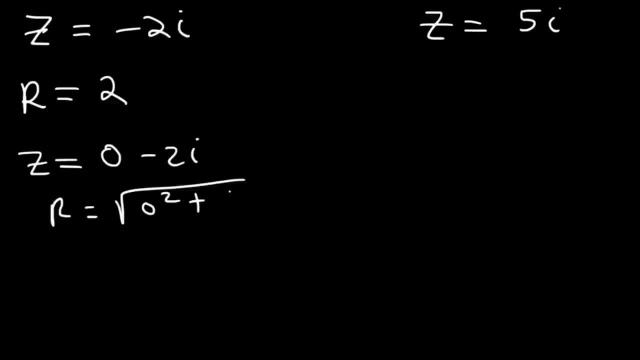 So r would be the square root of 0 squared, plus negative 2 squared, which is the square root of 4, which is 2.. So r is simply 2.. Now let's not use the inverse tangent formula. Instead, let's just plot. 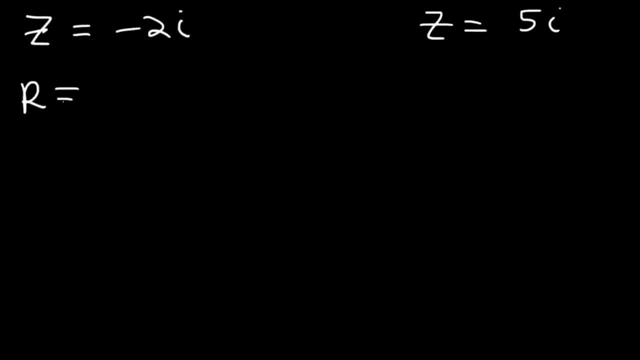 go ahead and try those two. so first we gotta find r. you can see that r is equal to 2. keep in mind z being negative, 2i is 0 minus 2i, so r would be the square root of 0 squared plus negative 2 squared, which is the square root of 4. 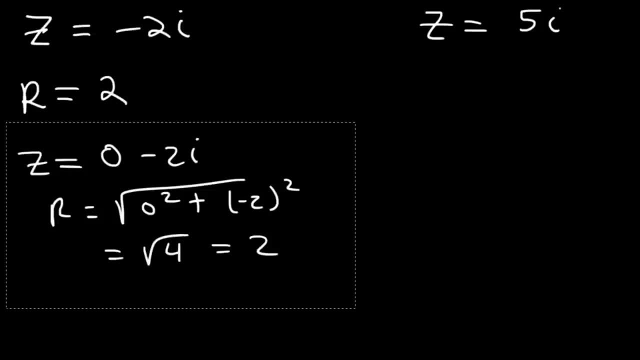 which is 2, so r is simply 2. now let's not use the inverse tangent formula. instead let's just plot negative 2i. negative 2i is on the negative y axis. so you can see: r is 2 units long and the angle. 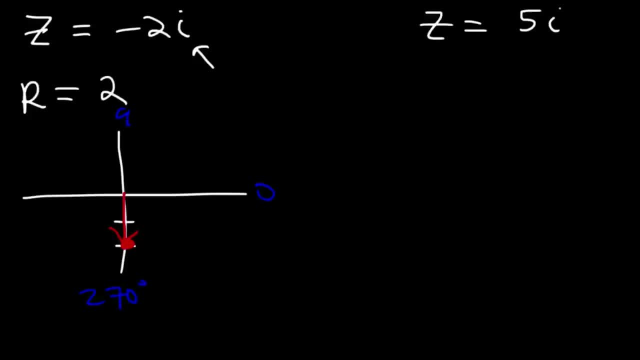 at this point is 270 degrees. so therefore z is equal to r, which is 2 times cosine of 270 plus i sine 270. now let's try the other one: z is equal to 5i, so clearly we can see that r is 5. 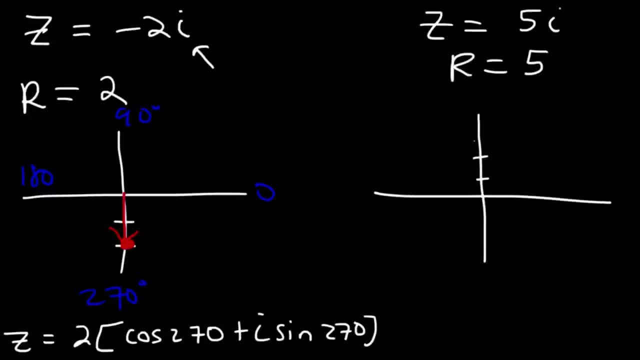 if we plot it, we just gotta travel 5 units in the y direction and we can see that the angle in a positive y axis is 90. so therefore z is going to be r, which is 5 times cosine of 90 plus i sine 90. 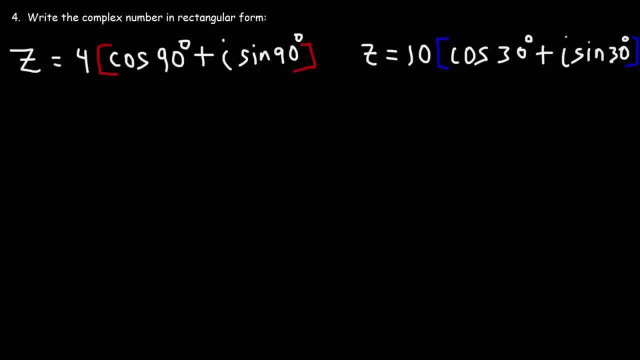 number 4. write the complex number in rectangular form. so let's start with the first example. all we need to do is basically plug in the numbers cosine of 90 degrees and remember to type that into your calculator. you'll get 0. sine of 90 is 1. 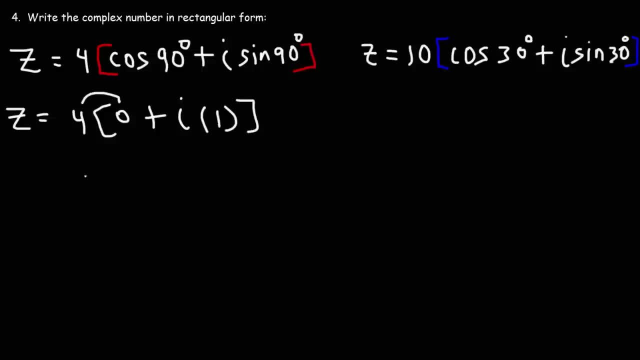 now all we need to do is distribute the 4. 4 times 0 is 0. 4 times 1i is simply 4i, so our final answer is: z is equal to 4i. for the next example, we're going to do the same thing. 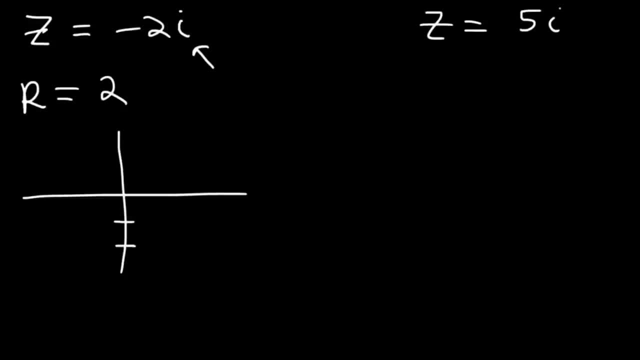 negative 2i. Negative 2i is on the negative y-axis. So you can see, r is 2 units long and the angle at this point is 270 degrees. So therefore, z is equal to r, which is 2,. 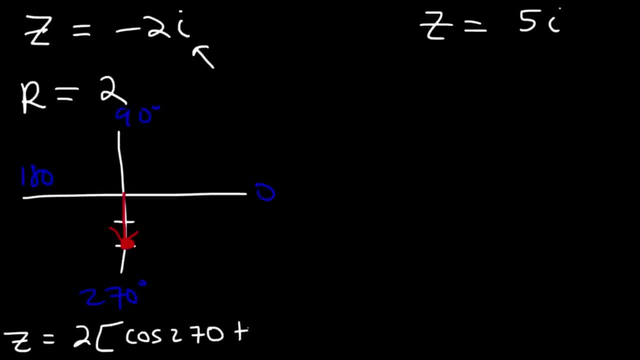 times cosine of 270, plus i sine 270.. Now let's try the other one. z is equal to 5i, So clearly we can see that r is 5.. If we plot it, we just gotta travel 5 units. 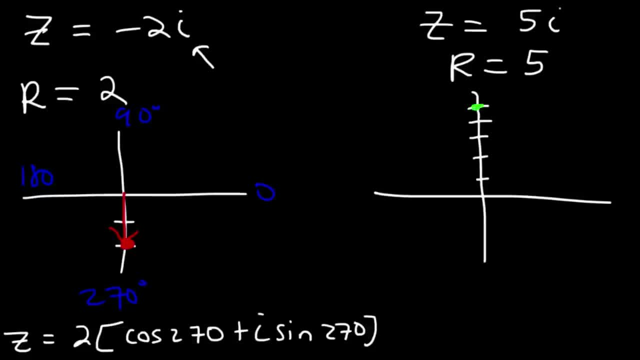 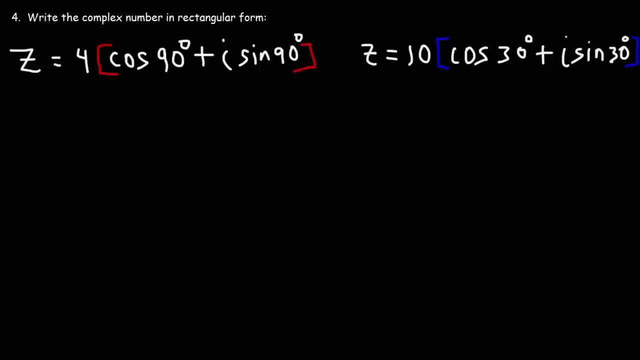 in the y-direction, And we can see that the angle in the positive y-axis is 90. So therefore, z is going to be r, which is 5, times cosine of 90, plus i sine 90. Number 4.. 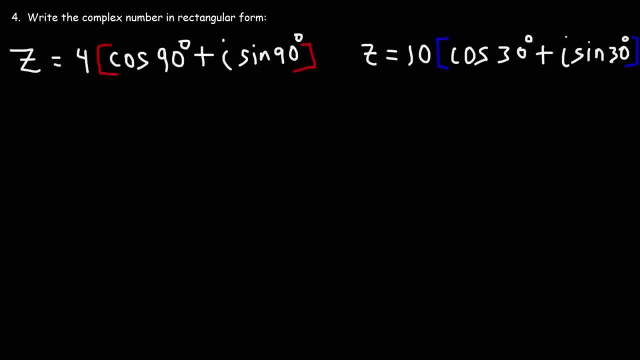 Write the complex number in rectangular form. So let's start with the first example. All we need to do is basically plug in the numbers Cosine of 90 degrees. if you were to type that into your calculator, you'll get 0.. 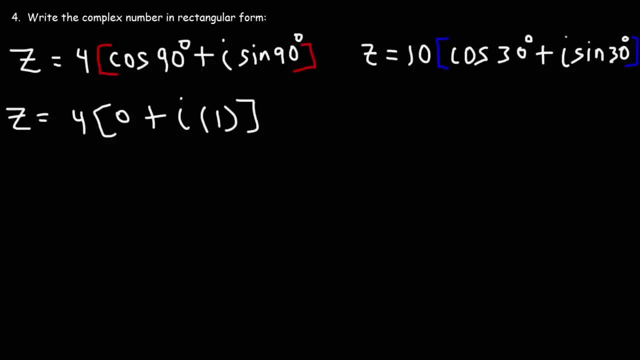 Sine of 90 is 1.. Now all we need to do is distribute the 4.. 4 times 0 is 0.. 4 times 1i is simply 4i, So our final answer is: z is equal to. 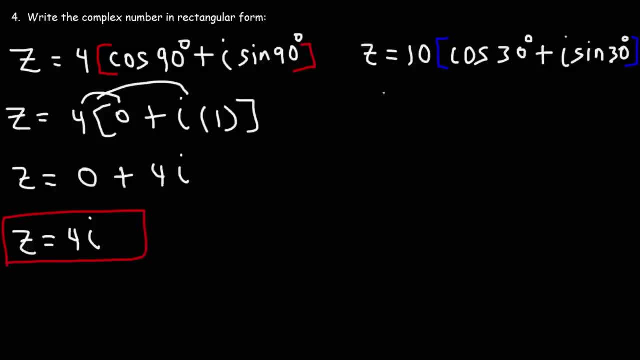 4i. For the next example, we're going to do the same thing. Cosine of 30 degrees. Cosine 30 is the square root of 3 over 2.. Sine 30 is 1 half. So now we've got to. 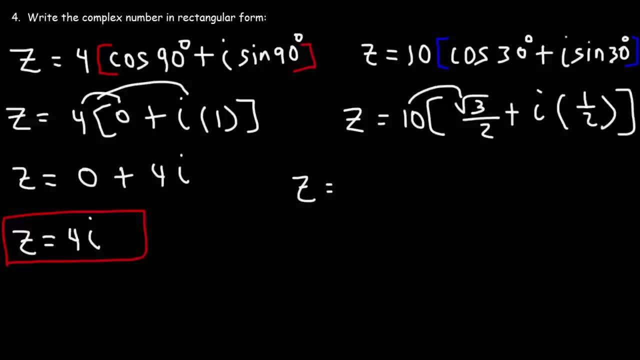 distribute the 10. So 10 times the square root of 3 over 2.. We know 10 over 2 is 5.. So this is going to be 5 square root 3.. Half of 10 is also 5.. 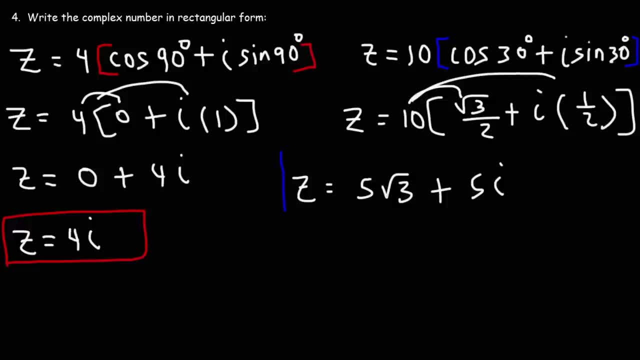 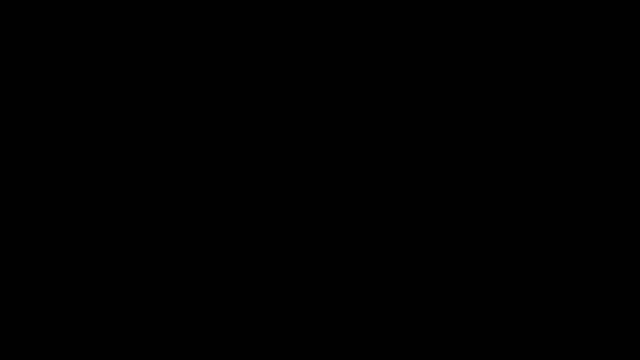 So this is going to be 5i, And so that's all we need to do in order to convert a complex number from polar form to rectangular form. Try this one. Let's say that z is equal to 20 cosine 4pi over 3. 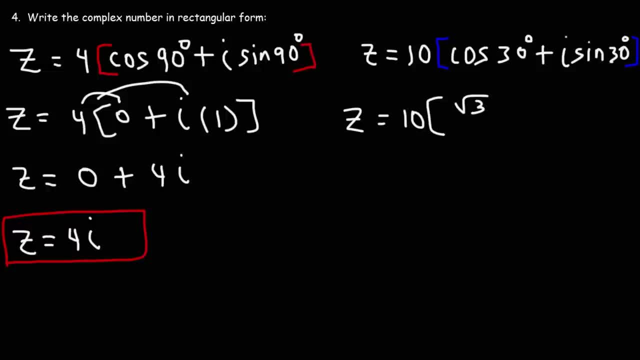 cosine of 30 degrees. cosine 30 is the square root of 30 over 2. sine 30 is 1 half. so now we gotta distribute the 10, so 10 times the square root of 3 over 2, we know 10 over 2 is 5. 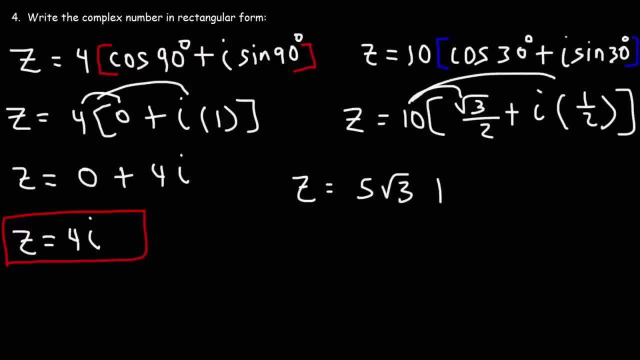 so this is going to be 5. square root 3, half of 10, is also 5, so this is going to be 5i, and so that's all we need to do in order to convert a complex number from polar form to rectangular form. 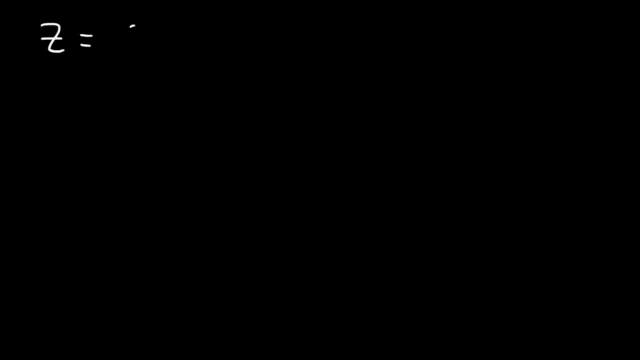 try this one. let's say that z is equal to 20 cosine 4pi over 3, plus i sine 4pi over 3. let's convert the angle from radians to degrees, so let's multiply by 180 over pi, so pi cancels. 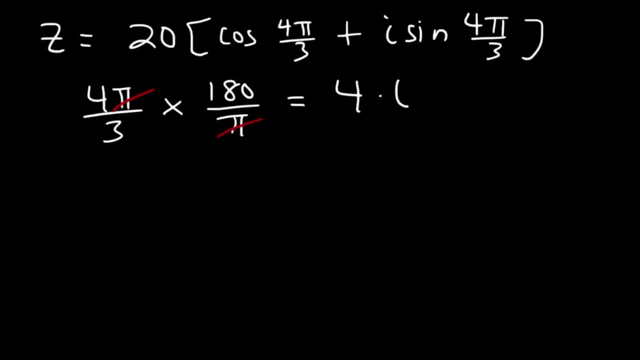 18 divided by 3 is 6. so 180 divided by 3 is 60. 4 times 60 is 240. cosine 240, that's the same as cosine 60. 60 is the reference angle of 240. if you do 240 minus 180, that's 60. 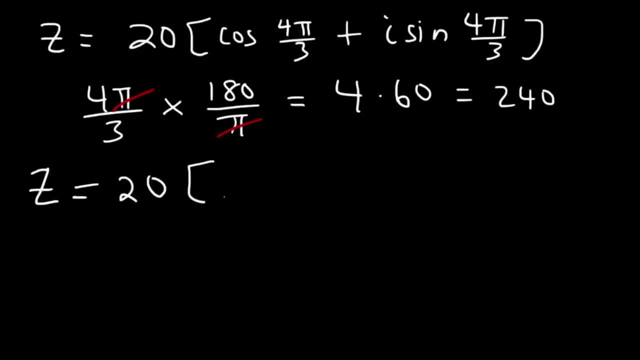 cosine 60 is 1 half, so cosine 240 is also 1 half. but 240 is in quadrant 3, so cosine 240 is negative 1 half. sine 240, which is similar to sine 60, sine 60 is root 3 over 2. 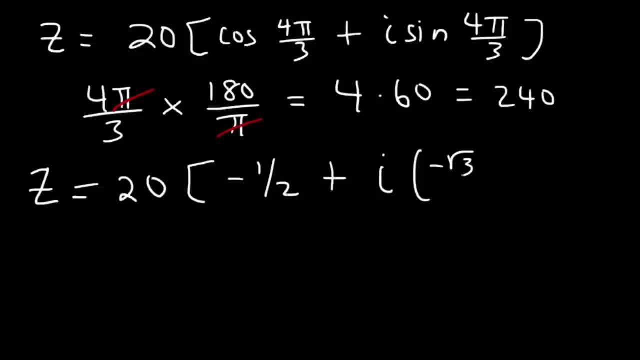 and sine 240. that's going to be negative root 3 over 2 because sine is negative. in quadrant 3, half of 20 is 10, so this is going to be negative 10 minus 10 root 3i. now for those of you out there who may need: 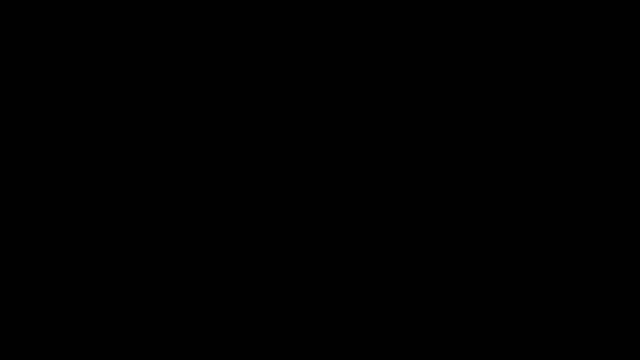 to evaluate cosine 240 or sine 240 without a calculator. here's what you can do. so first draw the angle 240- 240 is in quadrant 3, so this is 240 degrees- and turn it into a triangle- so this is 180, and if this is 240, 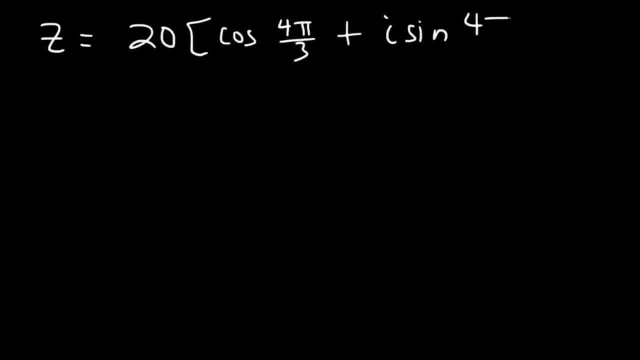 plus i sine 4pi over 3.. Let's convert the angle from radians to degrees. So let's multiply by 180 over pi. So pi cancels: 18 divided by 3 is 6.. So 180 divided by 3 is 60.. 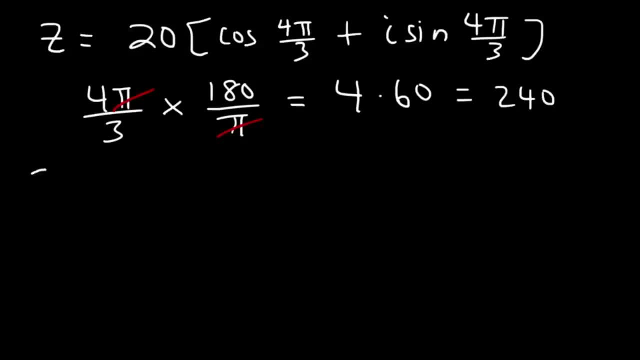 4 times 60 is 240.. Cosine 240, that's the same as cosine 60.. 60 is the reference angle of 240.. If you do 240 minus 180, that's 60.. Cosine 60 is 1 half, So cosine 240. 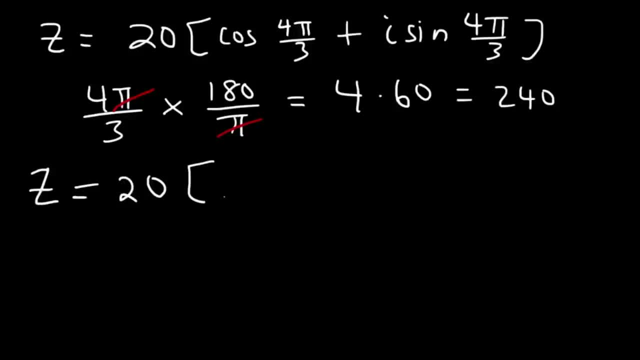 is also 1 half, But 240 is in quadrant 3, so cosine 240 is negative 1 half Sine 240, which is similar to sine 60. Sine 60 is root 3 over 2 and sine 240. 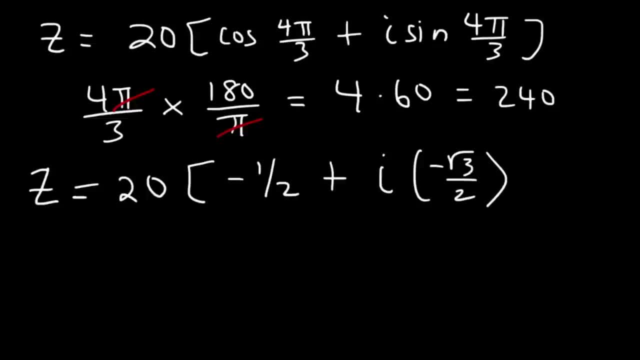 that's going to be negative. root 3 over 2. Because sine is negative in quadrant 3. Half of 20 is 10, so this is going to be negative: 10 minus 10. root 3i. Now for those of you out there: 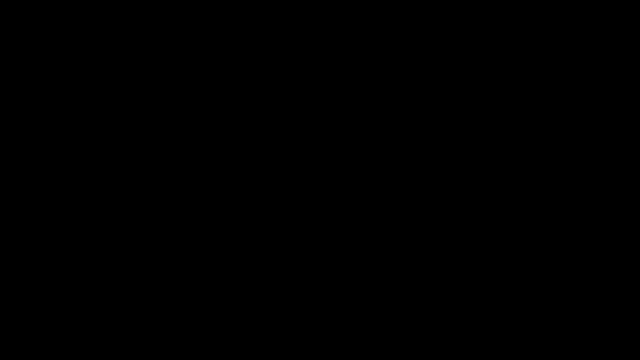 who may need to evaluate cosine 240 or sine 240 without a calculator. here's what you can do. So first draw the angle 240.. 240 is in quadrant 3.. So this is 240 degrees, And turn it into a triangle. 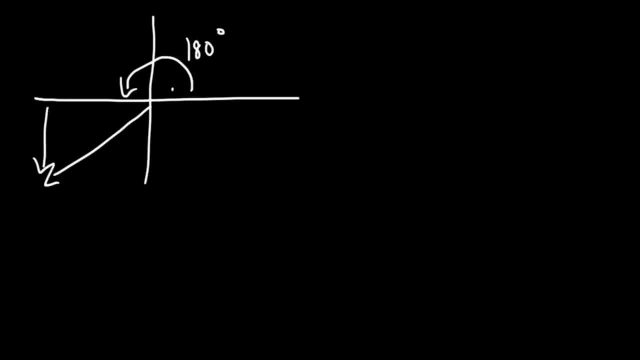 So this is 180.. And if this is 240, the difference must be 60.. So you need to realize that 60 is the reference angle To find the reference angle, and if your angle is in quadrant 3, it's going to be. 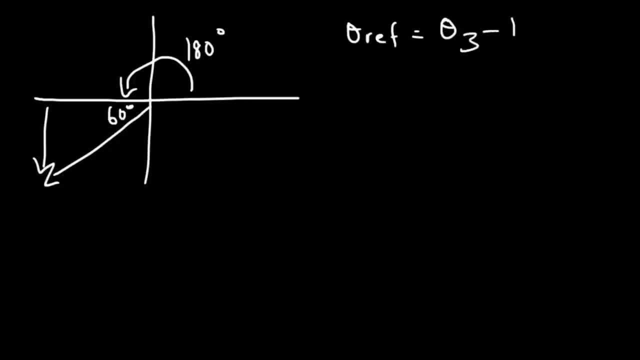 the angle in quadrant 3 minus 180.. To find it based on the angle in quadrant 2, it's 180 minus the angle in quadrant 2.. And if you have an angle in quadrant 4, it's going to be 360 minus the angle in quadrant 4.. 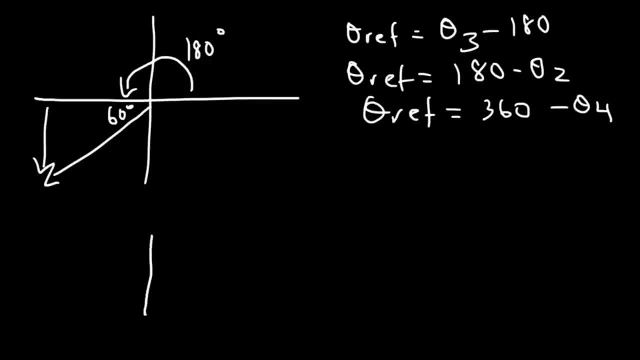 Now that we have the reference angle, we can solve it using the 30-60-90 reference triangle. Across the 30 is always going to be 1.. Across the 60 root 3 across the 92. So now we can evaluate. 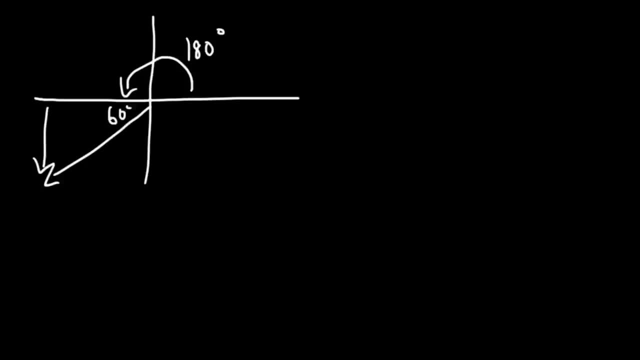 the difference must be 60, so you need to realize that 60 is the reference angle to find the reference angle, and if your angle is in quadrant 3, it's going to be the angle in quadrant 3 minus 180 to find it. and if your angle is in quadrant 2, 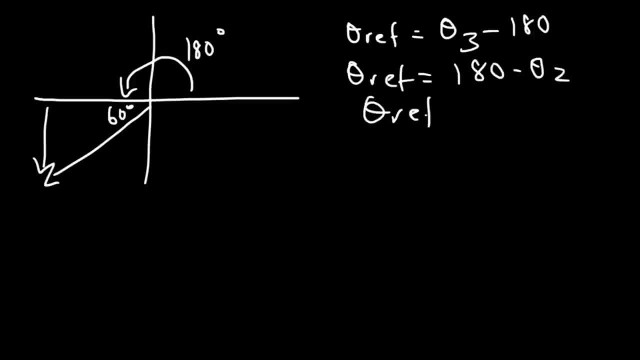 it's 180 minus the angle in quadrant 2, and if you have an angle in quadrant 4, it's going to be 360 minus the angle in quadrant 4. now that we have the reference angle, we can solve it using the 30, 60, 90. 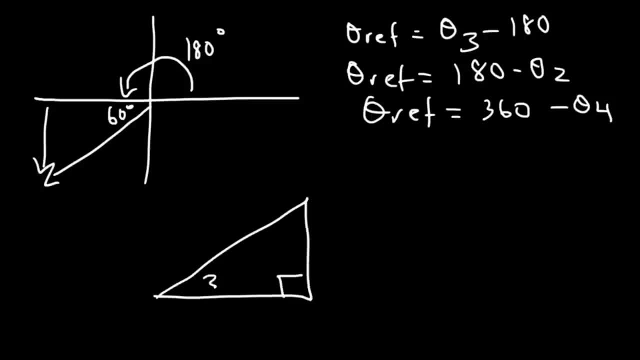 reference triangle across the 30 is always going to be 1 across the 60 root, 3 across the 92. so now we can evaluate sine of 60. sine based on circotoa is equal to the opposite side divided by the hypotenuse. 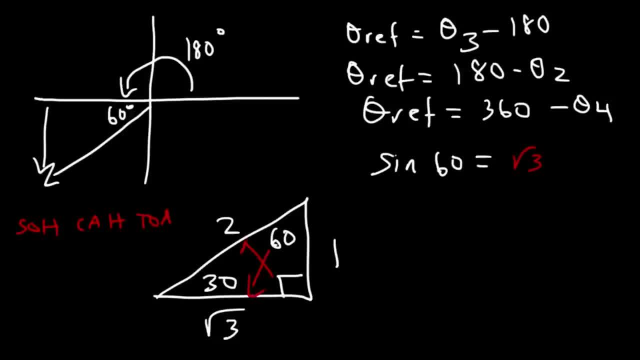 opposite to 60 is root 3. the hypotenuse is across the box, so that's going to be 2. so sine 60 is root 3 over 2. now sine 240 will also be root 3 over 2. you just got to determine if it's positive or negative. 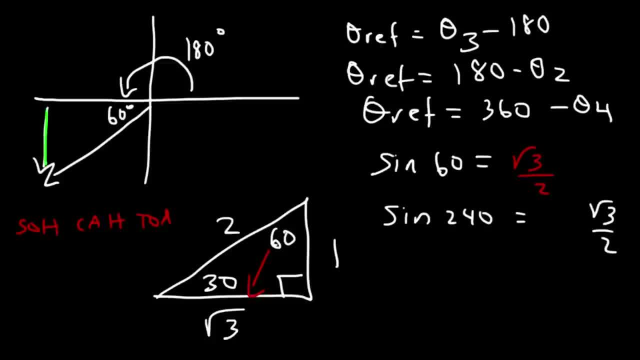 sine is associated with the y value and y is negative in quadrant 3, so this is going to be negative. root 3 over 2. cosine 240 is similar to cosine 60. cosine is adjacent over hypotenuse. adjacent to 60 is 1. 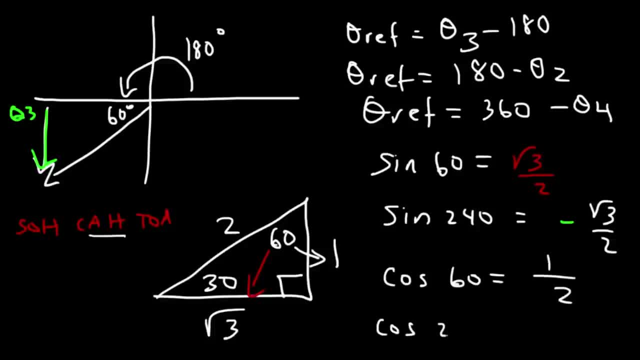 the hypotenuse is 2, so now we can find cosine 240 in quadrant 3. x is negative, so cosine 240 is negative. therefore it's negative 1 half. and so that's how you can find these values, based on the 30, 60, 90 triangle. 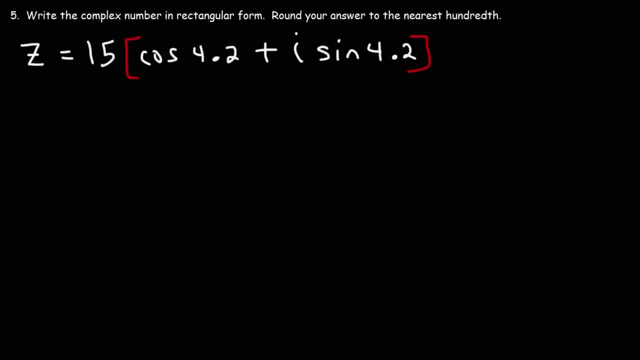 number 5. write the complex number in rectangular form. round your answer to the nearest hundredth. now, with this question we need to be a little bit careful, because the angle is not in degrees. this is not 4.2 degrees. if you don't see the degree symbol. 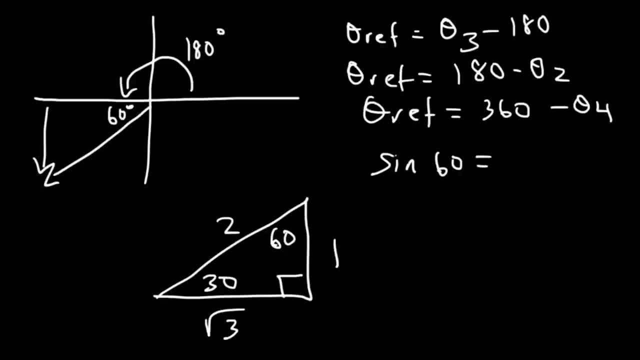 sine of 60. Sine based on SOHCAHTOA is equal to the opposite side divided by the hypotenuse. Opposite to 60 is root 3.. The hypotenuse is across the box, So that's going to be 2.. 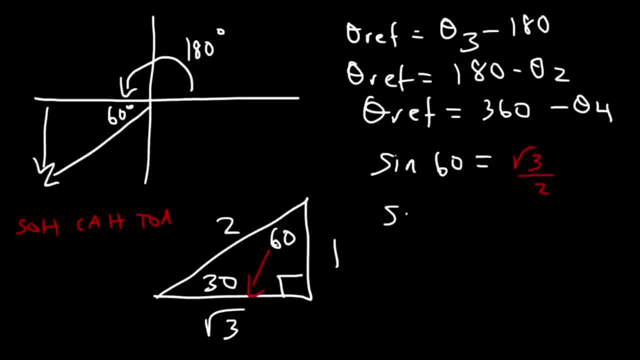 So sine 60 is root 3 over 2.. Now sine 240 will also be root 3 over 2.. You just got to determine if it's positive or negative. Sine is associated with the y value And y is negative. 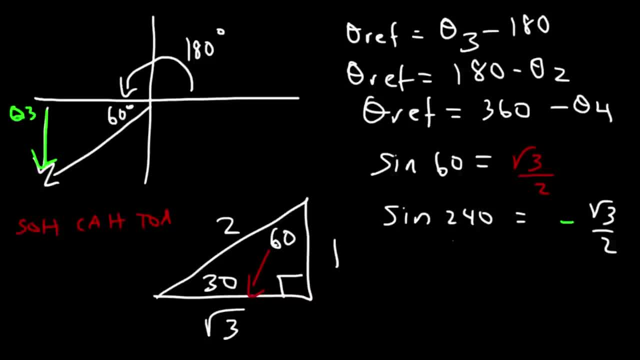 in quadrant 3.. So this is going to be negative. root 3 over 2.. Cosine 240 is similar to cosine 60. Cosine is adjacent over hypotenuse. Adjacent to 60 is 1.. The hypotenuse is 2.. 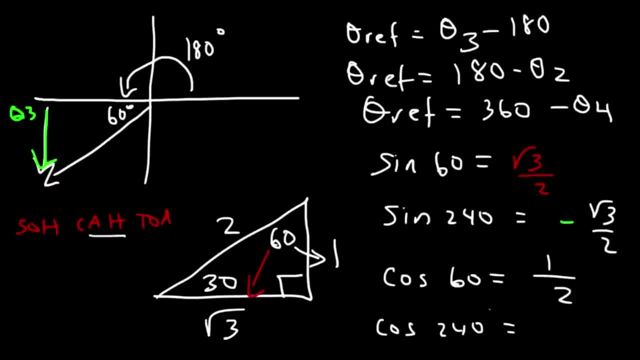 So now we can find cosine 240.. In quadrant 3, x is negative, So cosine 240 is negative. Therefore it's negative 1 half, And so that's how you can find these values based on the 30-60-90. 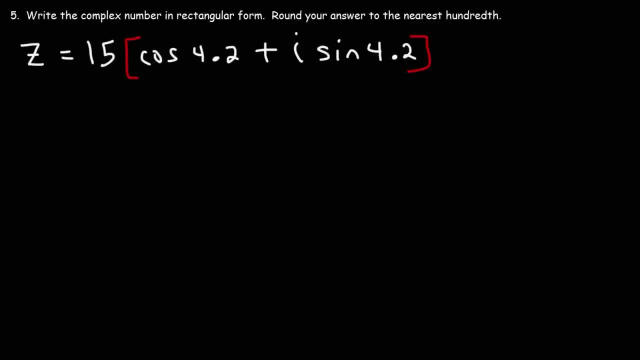 triangle Number 5.. Write the complex number in rectangular form. Round your answer to the nearest hundredth. Now, with this question we need to be a little bit careful, because the angle is not in degrees. This is not 4.2 degrees. 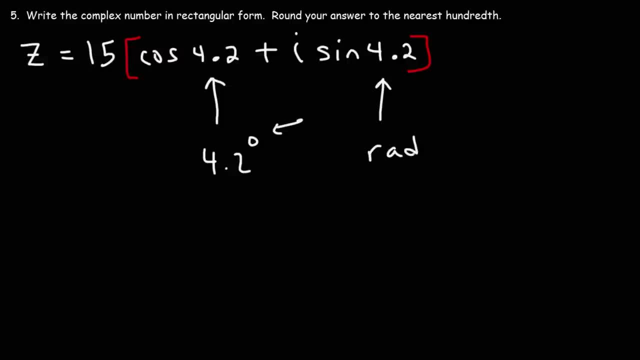 If you don't see the degree symbol, that means that the angle is in radians. So when you plug this into your calculator, make sure your calculator is in radian mode and not in degree mode. So before we plug in 4.2. 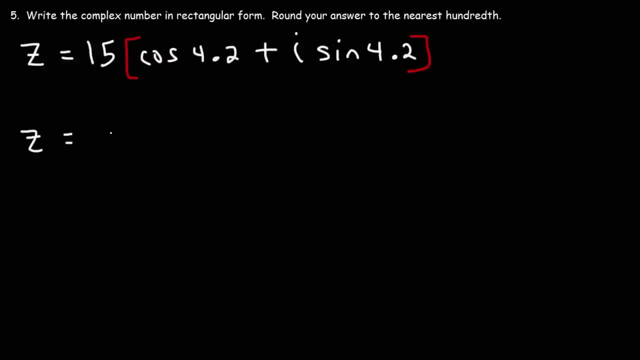 into cosine and sine. let's distribute the 15 first, So this is going to be 15 cosine 4.2 and then plus 15 sine, 4.2 times i Cosine 4.2, if your calculator is in radian mode, you should get. 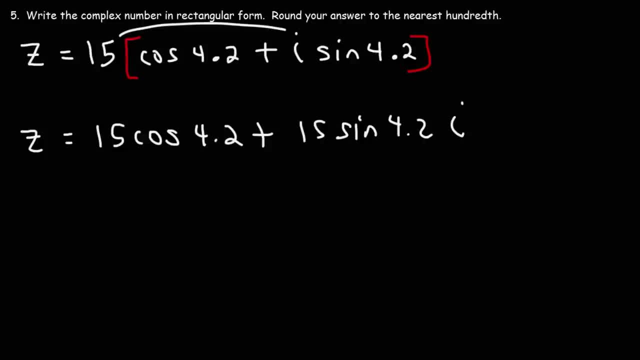 negative .49026.. We're going to take that black answer and multiply it by 15.. So you should get negative 7.3539 and so forth, But we're going to round that to the nearest hundredth. So that's going to be. 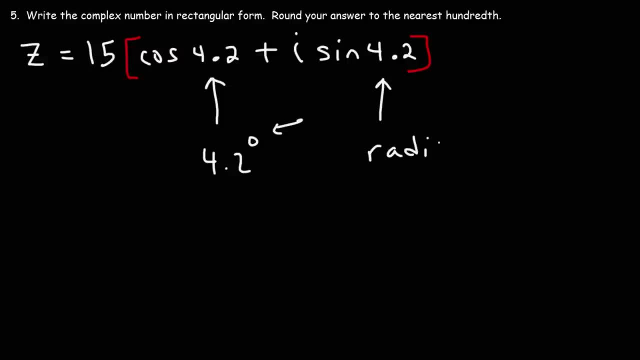 that means that the angle is in radians. so when you plug this into your calculator, make sure your calculator is in radian mode and not in degree mode. so before we plug in 4.2 into cosine and sine, let's distribute the 15 first. so this is going to be 15 cosine. 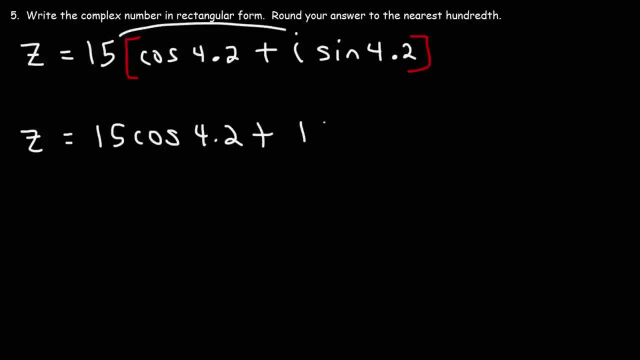 4.2 and then plus 15 sine 4.2 times, i cosine 4.2. if your calculator is in radian mode, you should get negative .49026. we're going to take that exact answer and multiply it by 15, so you should get negative. 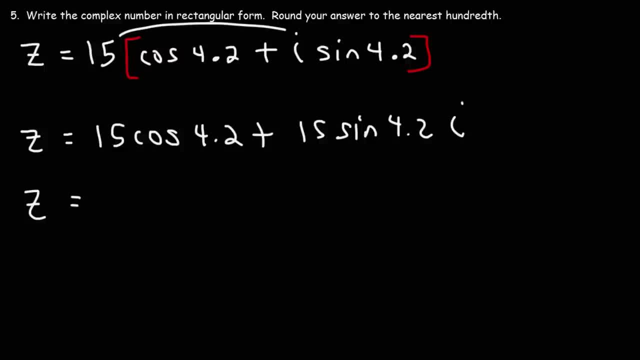 7.3539 and so forth. but we're going to round that to the nearest hundredth. so that's going to be negative 7.35 sine 4.2, that's negative .871575 if we multiply that by 15 and round it to the nearest hundredth. 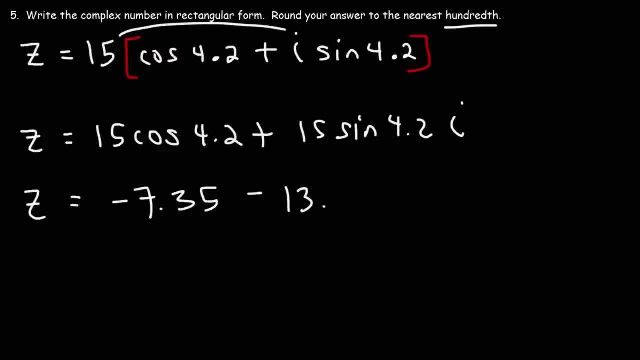 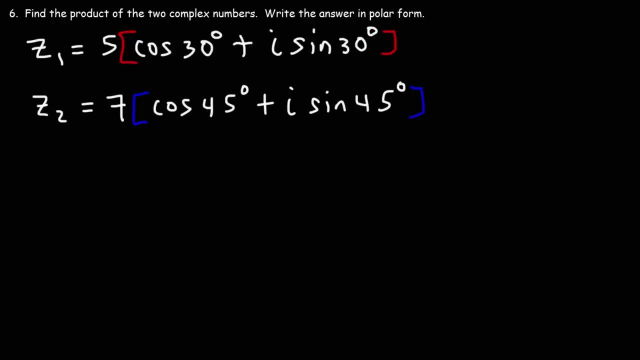 that's going to be negative 13.06. so that's the complex number in rectangular form, rounded to the nearest hundredth number: 6. find the product of the two complex numbers. write the answer in polar form. so, if you recall to find the product of two complex numbers, 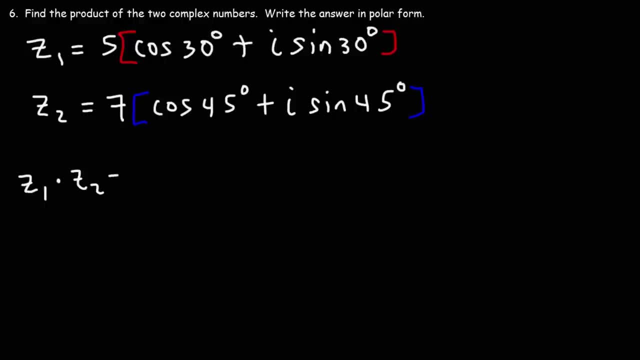 we could use this formula: it's r1 times r2, and then cosine theta1, and then cosine theta2 plus theta2, plus i sine theta1 plus theta2. so what we're going to do first is we're going to multiply r1 by r2. 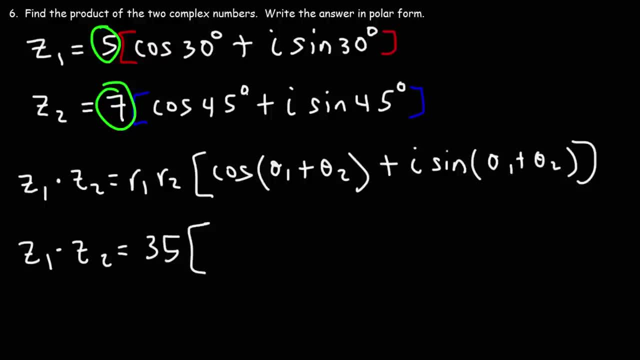 5 times 7 is 35. next, we're going to add up the angles: 30 plus 45 is 75. so this is going to be cosine 75 degrees plus i sine 75 degrees. so that's how you can find the two products. 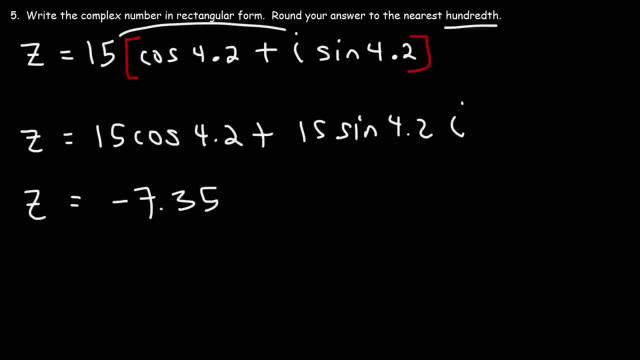 negative: 7.35.. Sine 4.2, that's negative .871575. and if we multiply that by 15 and round it to the nearest hundredth, that's going to be negative 13.07.. So that's the complex. 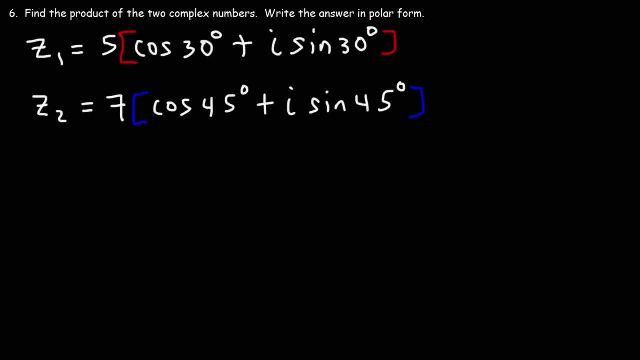 number in rectangular form, rounded to the nearest hundredth: Number. 6. Find the product of the two complex numbers. Write the answer in polar form. So if you recall to find the product of two complex numbers, we could use this formula. It's r1. 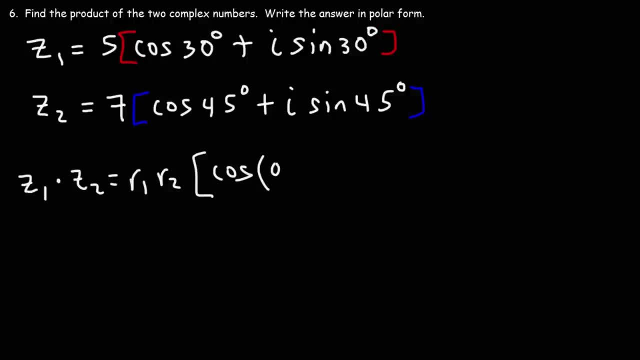 times r2, and then cosine theta1 plus theta2, plus i sine theta1 plus theta2.. So what we're going to do first is we're going to multiply r1 by r2.. 5 times 7 is 35.. Next we're going to add up the angles. 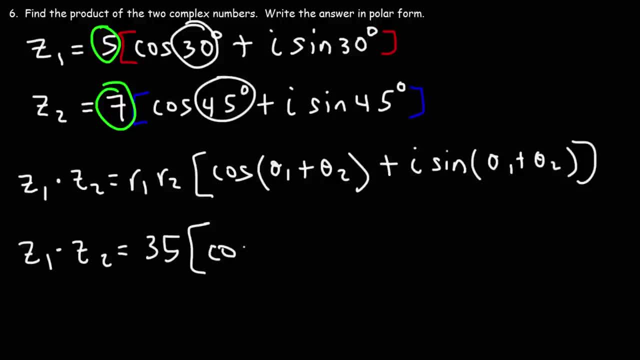 30 plus 45 is 75. So this is going to be cosine 75 degrees plus i sine 75 degrees. So that's how you could find the two products. I mean, that's how you could find the product of two complex numbers and 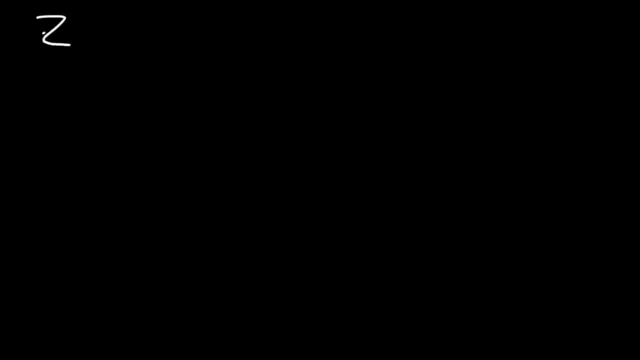 put it in polar form. Here's a practice problem that you could try. Let's say that z1 is 8 cosine 60 plus i sine 60.. And also that z2 is 5 cosine 100 plus i sine 100.. 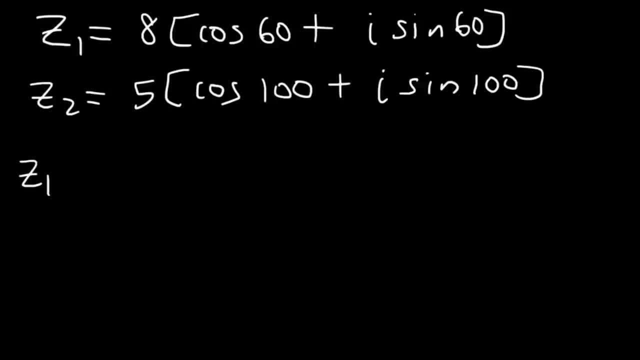 Go ahead and find the product of z1 and z2.. So feel free to pause the video and work on it. So first let's multiply 8 times 5. So that's going to be 40.. Next let's add: 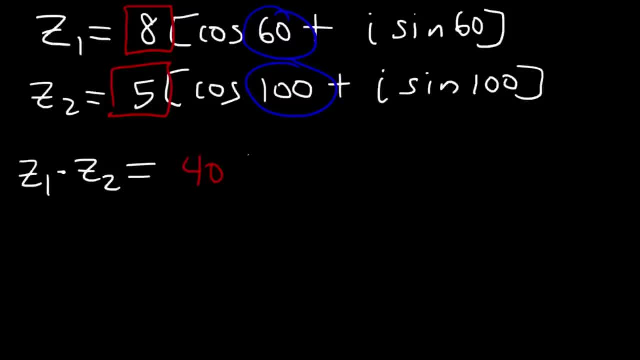 60 plus 100, which is going to be 160.. So the answer is 40 cosine 160 plus i sine 160.. Now sometimes you might have to work out this problem with an angle in radians as opposed to degrees. So let's say: 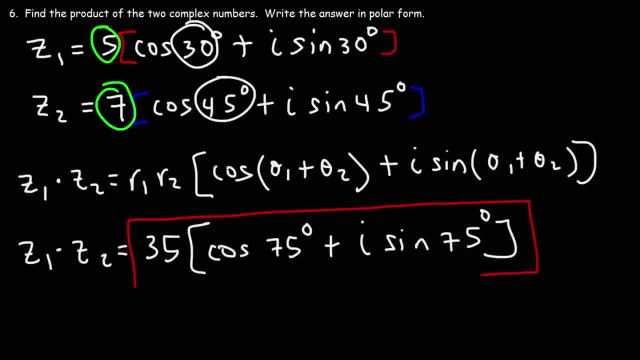 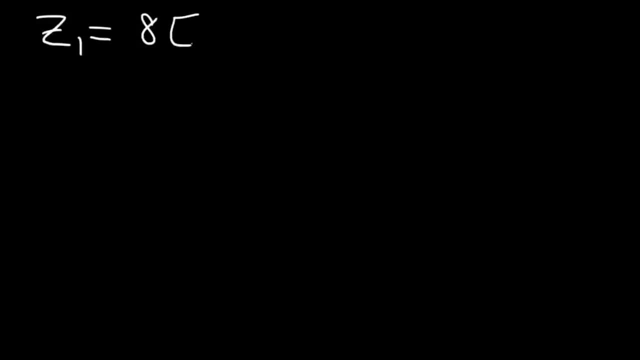 I mean, that's how you can find the product of two complex numbers and put it in polar form. here's a practice problem that you can try. let's say that z1 is 8 cosine 60 plus i sine 60, and also that z2. 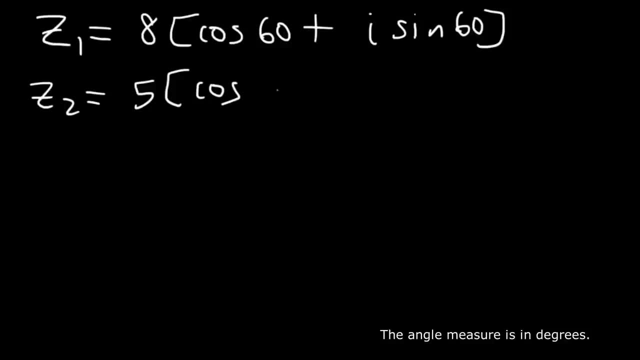 is 5, cosine 100 plus i sine 100. go ahead and find the product of z1 and z2. so feel free to pause the video and work on it. so first let's multiply 8 times 5, so that's going to be 40. 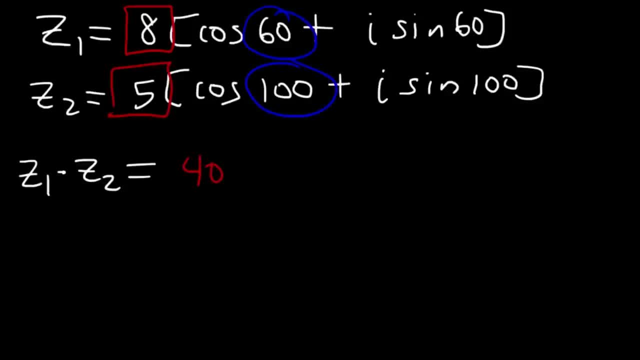 next, let's add 60 plus 100, which is going to be 160. so the answer is 40 cosine 160 plus i sine 160. now sometimes you might have to work out this problem with an angle in radians as opposed to degrees. so let's say that. 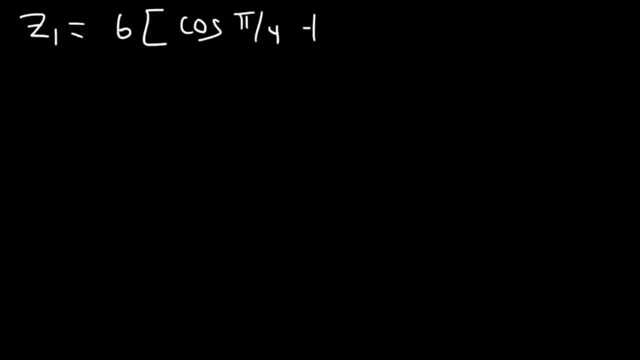 c1 is 6 cosine pi over 4 plus i sine pi over 4, and that z2 is 3 cosine pi over 3 plus i sine pi over 3. so r1 times r2, 6 times 3, that's going to be 18. 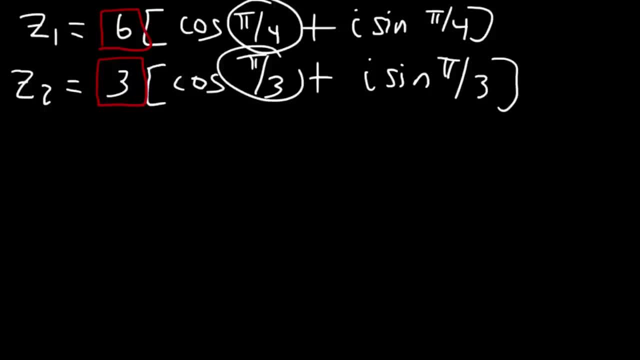 so let's not worry about that. for now. let's add pi over 4 plus pi over 3, so what we need to do is get common denominators. so let's multiply this fraction by 3 over 3 and the other one by 4 over 4. 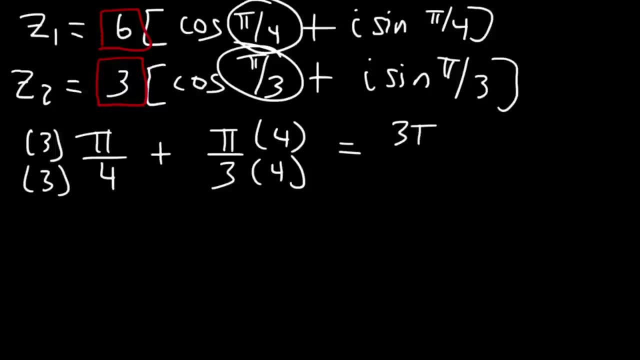 so this becomes 3 pi over 12 plus 4 pi over 3 plus 4 pi over 12. so the sum of the two angles is 7 pi over 12. so therefore the product of z1 and z2 is going to be 6 times 3. 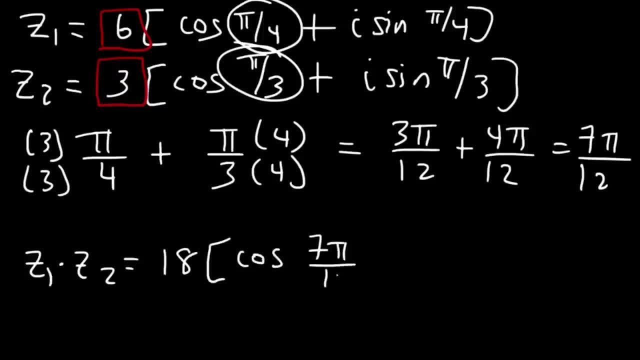 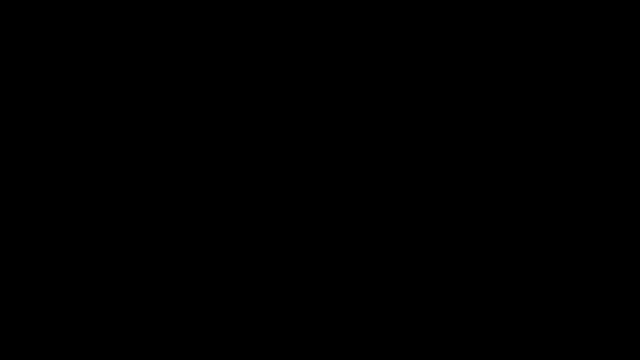 which is 18, and then cosine 7 pi over 12 plus i sine 7 pi over 12. now let's say that z1 is equal to z2 and z2 is 5 plus 12i. so what is the product of z1 and z2? 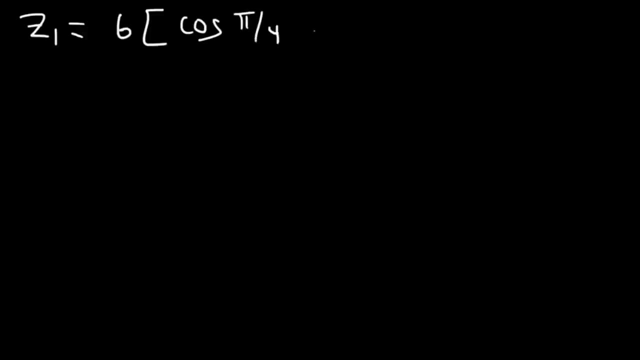 that c1 is 6 cosine pi over 4 plus i sine pi over 4.. And that z2 is 3 cosine pi over 3 plus i sine pi over 3.. So r1 times r2.. 6 times 3, that's going to be 18.. 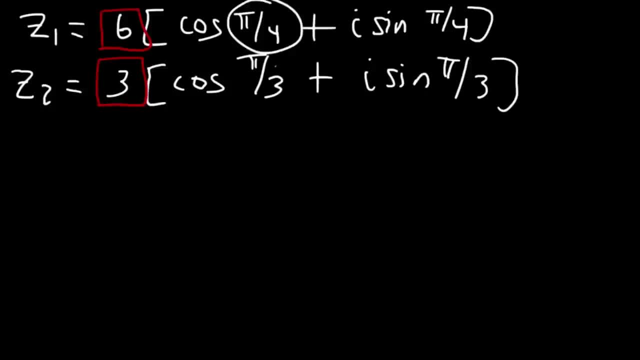 So let's not worry about that for now. Let's multiply. rather, let's add pi over 4 plus pi over 3.. So what we need to do is get common denominators. Let's multiply this fraction by 3 over 3. 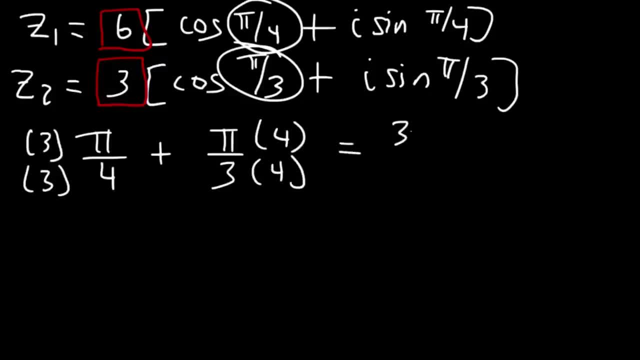 and the other one by 4 over 4.. So this becomes 3 pi over 12 plus 4 pi over 12.. So the sum of the two angles is 7 pi over 12.. So therefore, the product of z1 and z2. 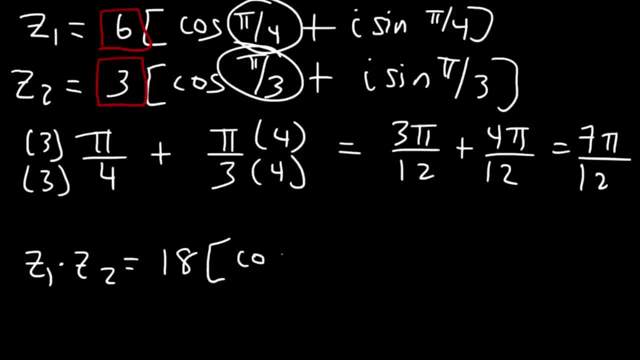 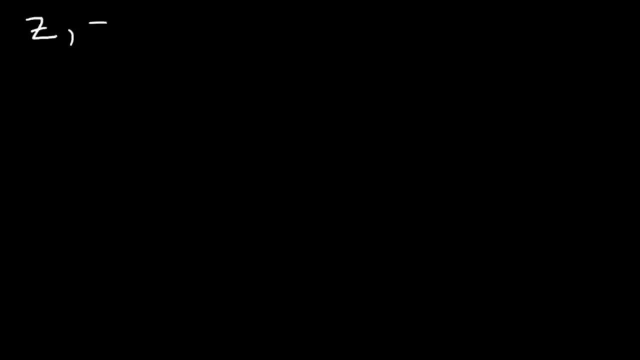 is going to be 6 times 3, which is 18.. And then cosine 7 pi over 12 plus i, sine 7 pi over 12.. Now let's say that z1 is equal to 3 minus 4, i and. 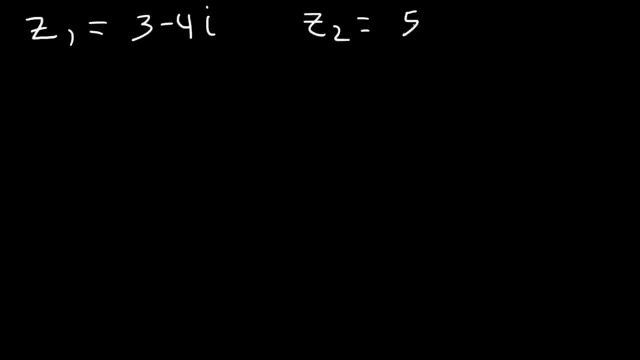 z2 is 5 plus 12 i. So what is the product of z1 and z2 in polar form? Now we can multiply z1 and z2 first and then convert it to polar form, or we could convert z1 and z2 into its polar. 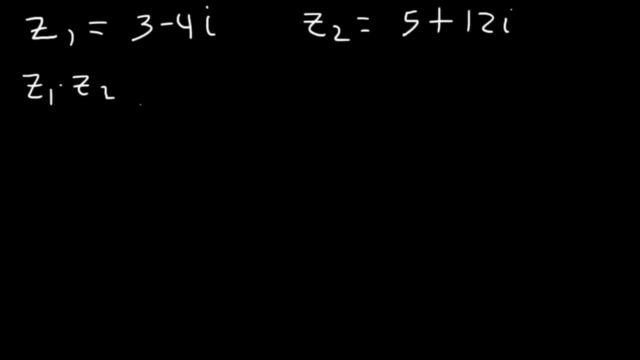 form and then multiply. For the sake of your understanding, let's do it both ways. Let's multiply the two the way it is right now. So 3 minus 4, i times 5 plus 12, i 3 times 5, is 15. 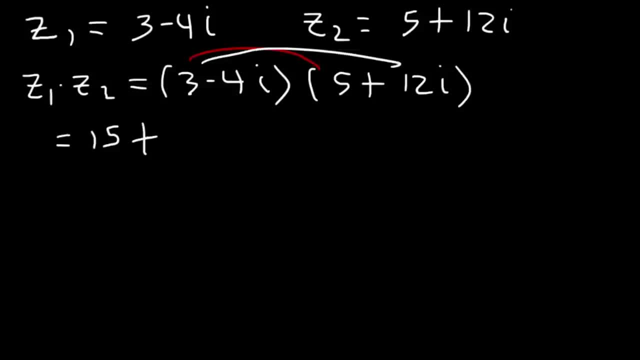 and 3 times 12 i, that's going to be 36 i. Negative 4 i times 5 is negative 20 i and negative 4 i times 12 i is negative 48 i squared. Now let's go ahead and combine like terms. 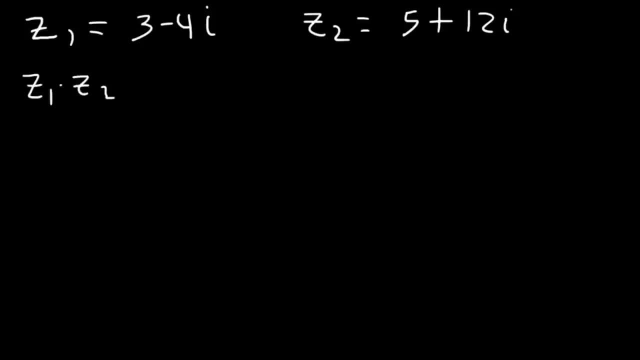 in polar form. now we can multiply z1 and z2 first and then convert it to polar form, or we could convert z1 and z2 into its polar form and then multiply. for the sake of your understanding, let's do it both ways. let's multiply the two the way it is right now. 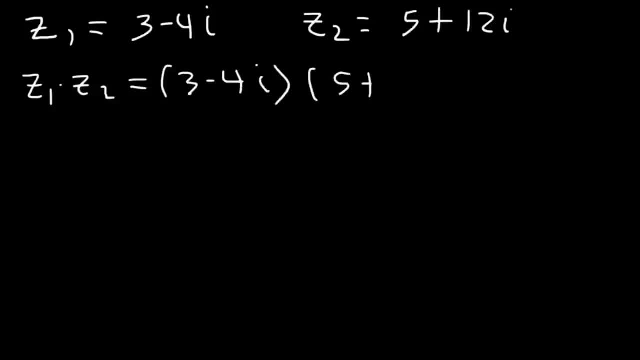 so 3 minus 4i times 5 plus 12i. 3 times 5 is 15 and 3 times 12i, that's going to be 36i. negative 4i times 5 is negative 20i and negative 4i times 12i. 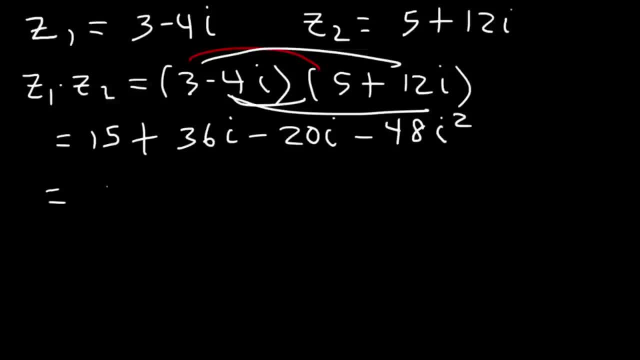 is negative 48i squared. now let's go ahead and combine like terms: 36i minus 20i is equal to positive 16i and i squared is negative 1, so negative 48i squared is positive 48, and then we can add 15. 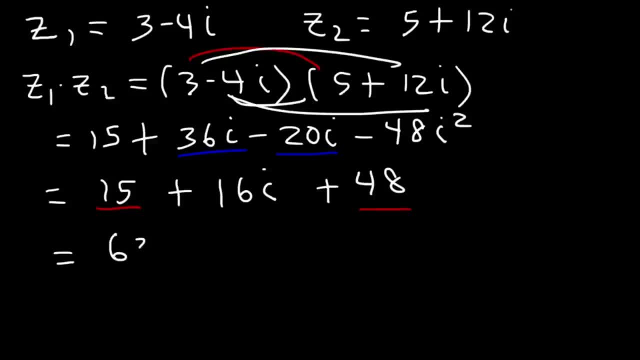 and 48. so therefore we have 63 plus 16i. so that's the product of z1 and z2 in rectangular form. now let's take that answer and convert it to polar form. now let's go ahead and find r. so r is going to be. 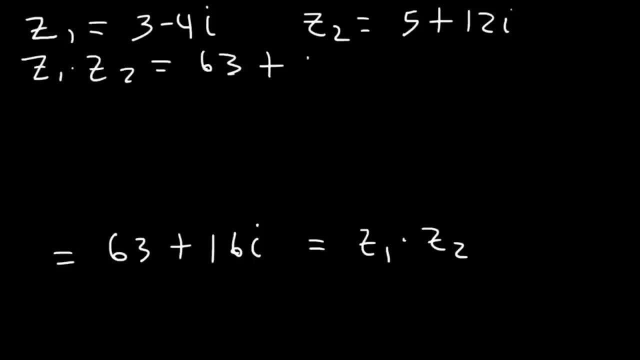 the square root of 63 squared plus 16 squared. so if you type this in, 63 squared is 3,969 plus 16 squared, which is 2. so if you type this in, 63 squared is 3,969 plus 16 squared. 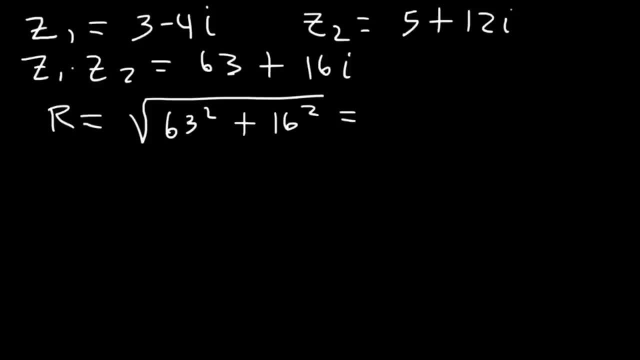 which is 2, which is 256. that adds up to 4,225. the square root of 42,25 is 65, so that's r. so now let's find the reference angle. so that's going to be arctangent b over a. 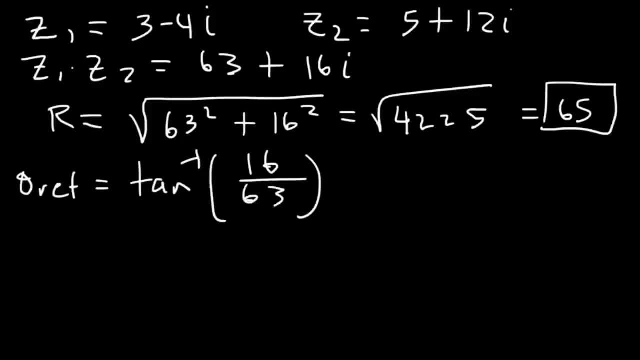 or 16 divided by 63. arctan of 16 over 63, that's 14.25 degrees. now a and b are both positive. therefore r is in quadrant 1, which means we need an angle between 0 and 90 and we have it, so we don't have to. 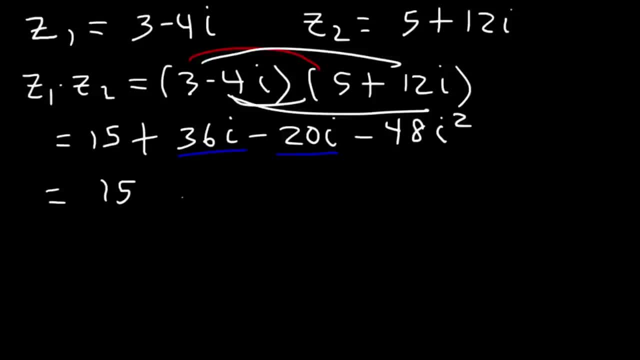 36 i minus 20. i is equal to positive 16 i And i squared is negative 1, so negative 48, i squared is positive 48.. And then we can add 15 and 48.. So therefore we have 63 plus 16 i. 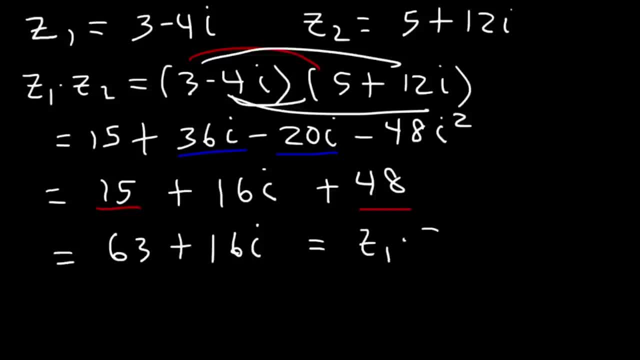 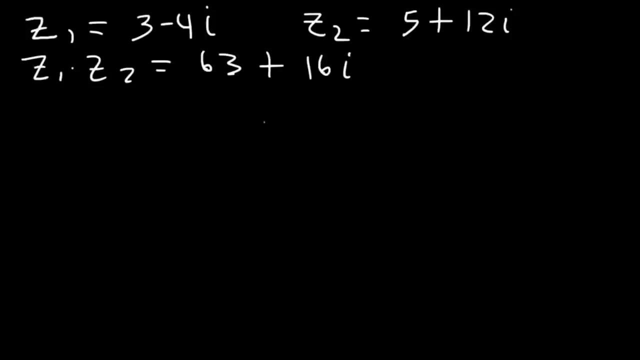 So that's the product of z1 and z2 in rectangular form. Now let's take that answer and convert it to polar form. Now let's go ahead and find r. So r is going to be the square root of 63 squared. 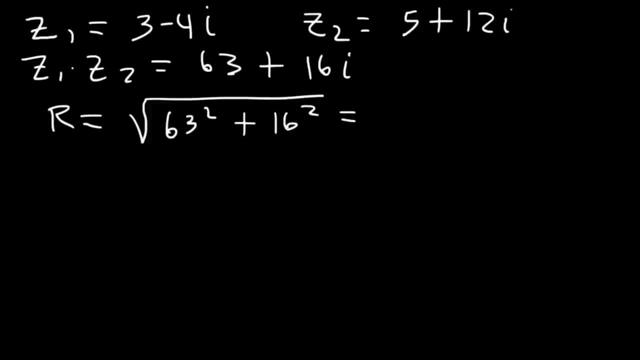 plus 16 squared. So if you type this in, 63 squared is 3,969 plus 16 squared, which is 256.. That adds up to 4,225.. The square root of 42,25 is 65.. So that's r. 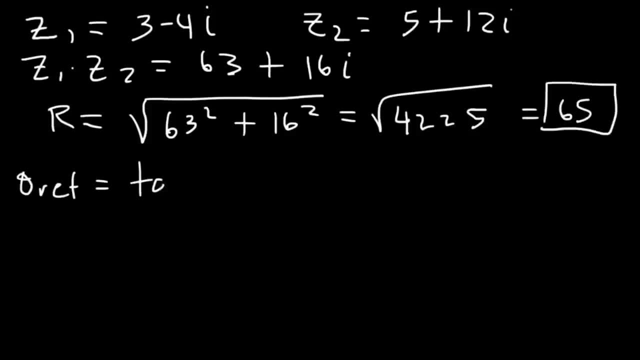 So now let's find a reference angle. So that's going to be arctangent b over a, or 16 divided by 63.. Arctan of 16 over 63, that's 16.25 degrees. Now a and b are both positive. 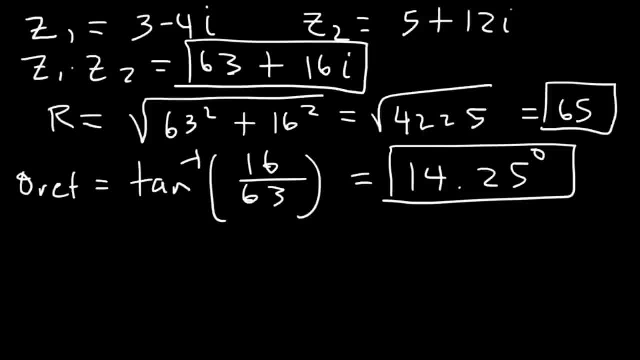 Therefore, r is in quadrant 1. Which means we need an angle between 0 and 90. And we have it, so we don't have to modify this angle. So therefore, z1 and z2 is going to be r, which is 65. 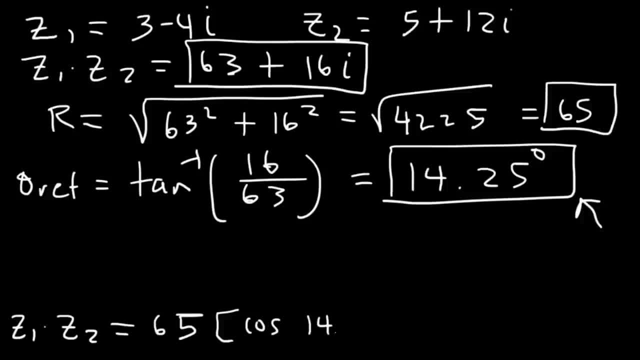 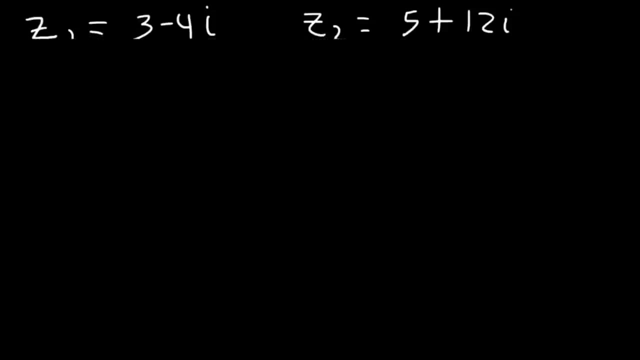 times cosine of 14.25 degrees plus i sine of 14.25 degrees. So remember this answer because we're going to get the same answer using another technique. So now let's convert z1 and z2 into its polar form individually. 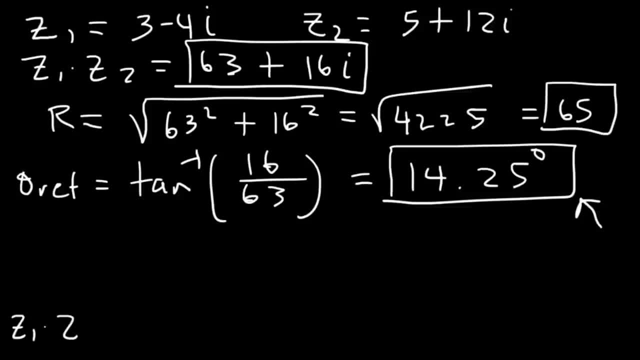 modify this angle. so therefore z1 and z2 is going to be r, which is 65 times cosine of 14.25 degrees plus i sine 14.25 degrees. so remember this answer, because we're going to get the same answer using another technique. 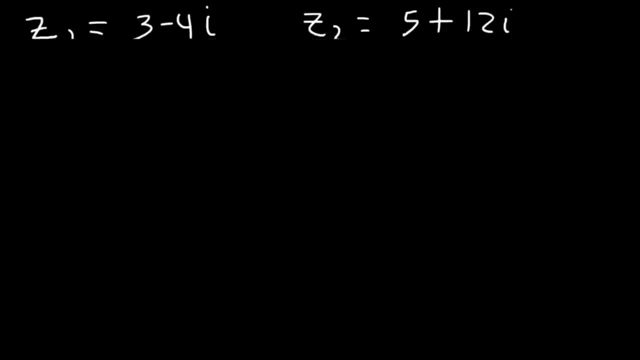 so now let's convert z1 and z2 into its polar form individually. so first let's find r. so r is going to be the square root of 3 squared plus negative 4 squared, that's 9 plus 16, which is 25, and the square root of 25 is 5. 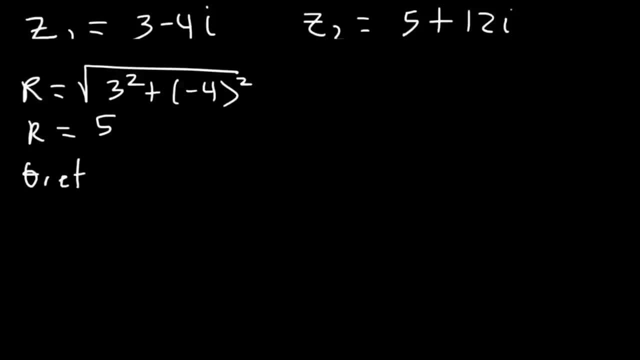 next, let's find a reference angle, so it's going to be arctan y over x. but let's use positive 4 and positive 3, so this is going to be 53.13 if we plot it. x is well, a is 3. 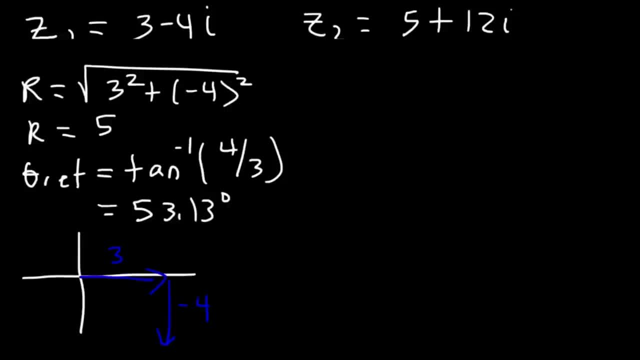 and b is negative 4. so therefore r is in quadrant 4 with a reference angle of 53.13. so to find the actual angle, it's going to be 360 minus the reference angle. so 360 minus 53.13 that's 306.87. 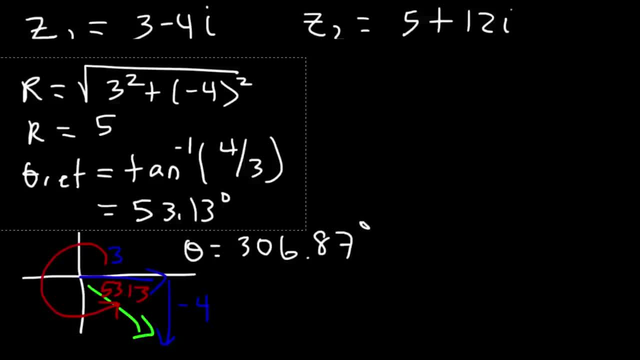 now let's express z1 in polar form. so keep in mind: r is 5 for z1, so it's going to be 5 cosine 306.87 plus i sine 306.87. now let's do the same for z2. so first, 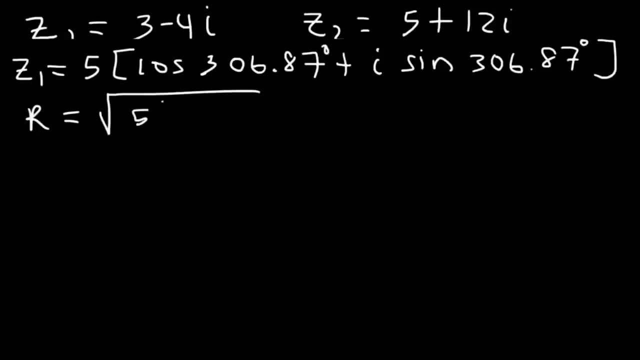 let's find r. r is going to be the square root of 5 squared plus 12 squared. 5 squared is 25, 12 squared is 144, and these two add up to 169, and the square root of 169 is 13. so that's r. 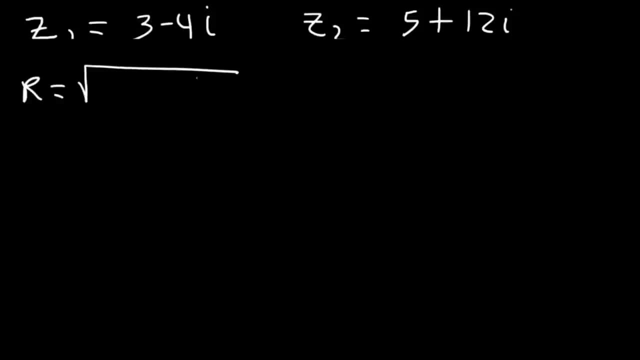 So first let's find r. So r is going to be the square root of 3 squared plus negative 4 squared plus 16, which is 25.. And the square root of 25 is 5.. Next, let's find a reference angle. 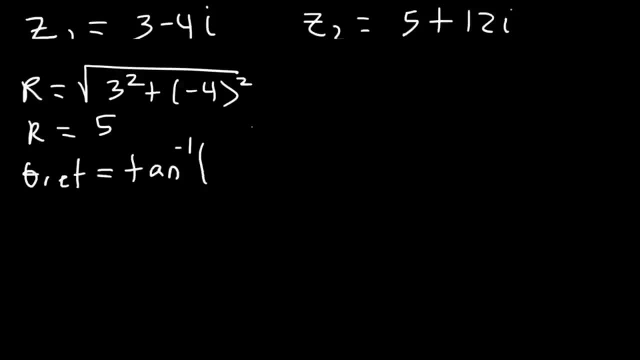 So it's going to be arctangent y over x, But let's use positive 4 and positive 3.. So this is going to be 53.13.. If we plot it, x is 3, and b is negative 4.. 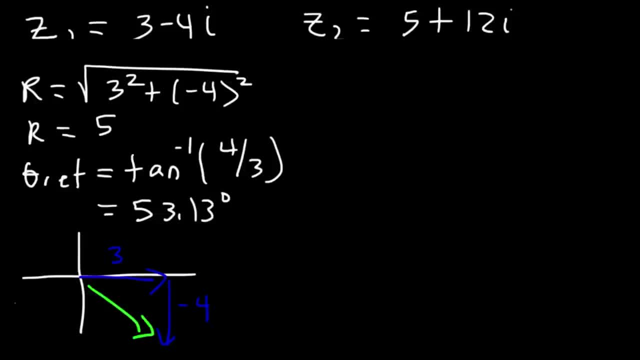 So therefore, r is in quadrant 4.. With a reference angle of 53.13.. So to find the actual angle, it's going to be 360 minus the reference angle. So 360 minus 53.13, that's 306.87.. 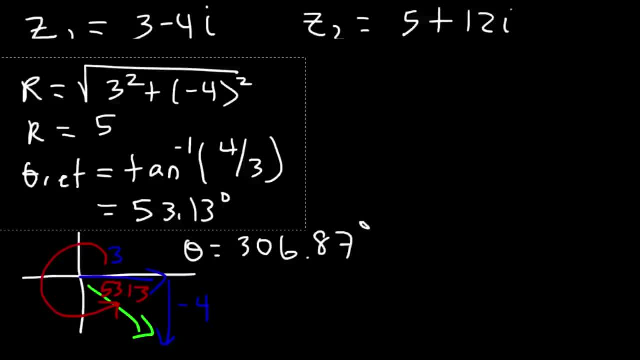 Now let's express z, z1 in polar form. So keep in mind: r is 5 for z1.. So it's going to be 5 cosine 306.87 plus i sine 306.87.. Now let's do the same for z2.. 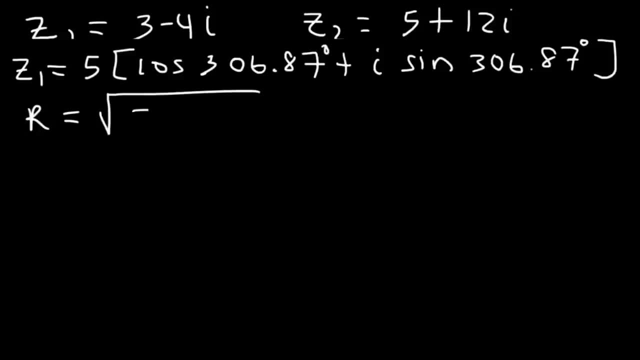 So first let's find r. r is going to be the square root of 5 squared, plus 12 squared. 5 squared is 25.. 12 squared is 144.. And these two add up to 169. And the square root of 169 is 13.. 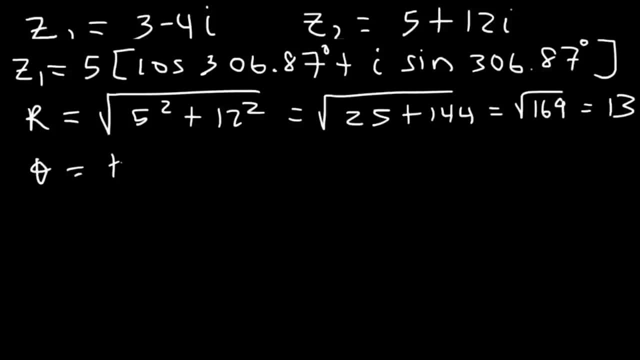 So that's r. So now let's find the angle. So this is going to be the inverse tangent of 12 over 5. And that's equal to 67.38 degrees. Now a and b are both positive, so therefore, 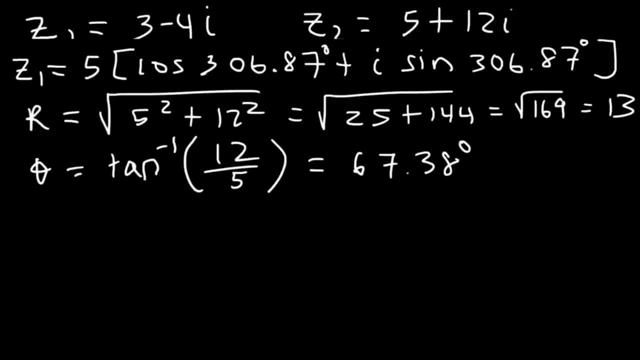 the reference angle is the same as the actual angle that we need. If they're both positive, r is going to be in quadrant 1. And we have an angle that's in quadrant 1. So we don't have to change it. 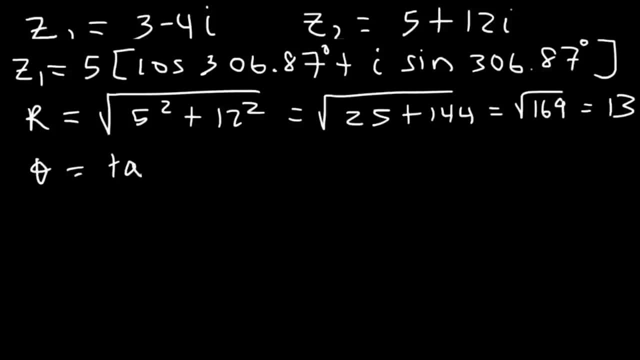 so now let's find the angle. so this is going to be the inverse tangent of 12 over 5, and that's equal to 67.38 degrees. now a and b are both positive, so therefore the reference angle is the same as the actual angle that we need. 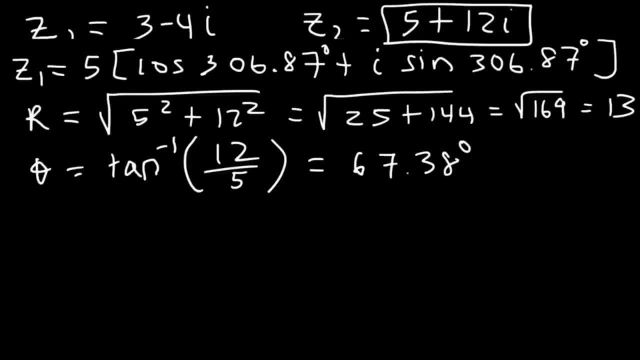 if they're both positive, r is going to be in quadrant 1 and we have an angle that's in quadrant 1, so we don't have to change it. so now we can express z2 as 13 cosine 67.38 plus i sine. 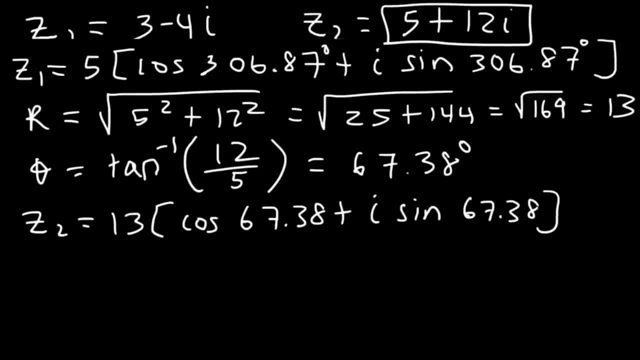 67.38. so now we can find a product of z1 and z2. so first, z1 times z2, we got to multiply r1 and r2. so 5 times 13 is 65. next we need to add the two angles. so let's add. 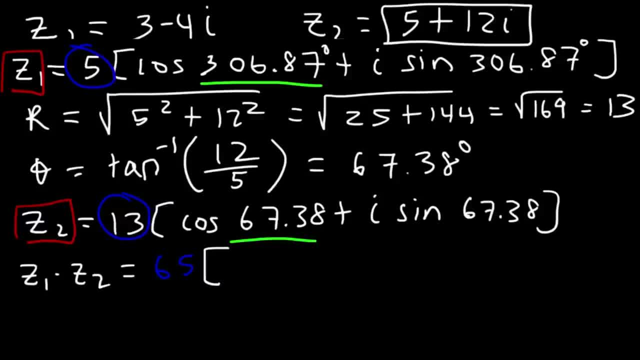 306.87 plus 67.38. now, if you add those two angles, you're going to get 374.25, which is greater than 360. so let's find the angle between 0 and 360. to do that, subtract it by 360. 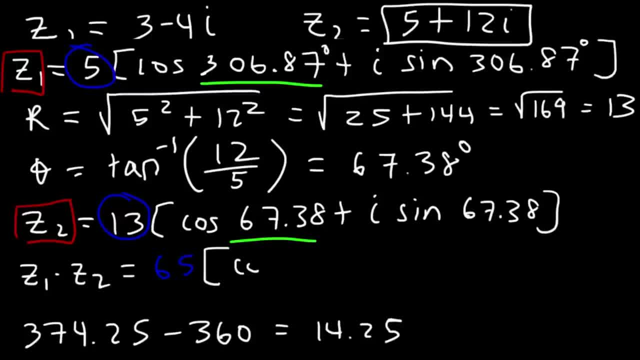 and this will give you 14.25. so now we have the same answer: 65 cosine 14.25, plus i sine 14.25. personally, i believe that the first method is a lot easier than the second, but now you know how to do it both ways. 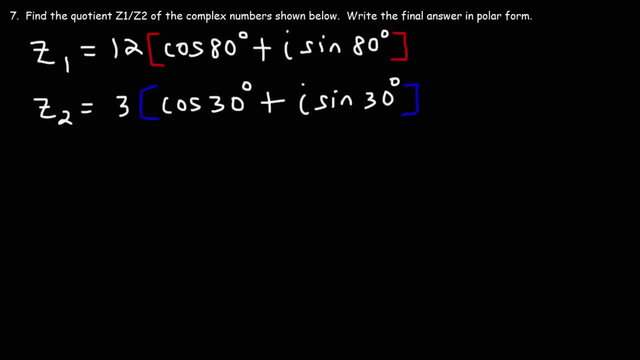 number 7 find the quotient z1 over z2 of the complex numbers shown below. so first let's write the formula: z1 over z2 is going to be r1 over r2 times cosine of theta1 minus theta2 plus i sine theta1 minus theta2. 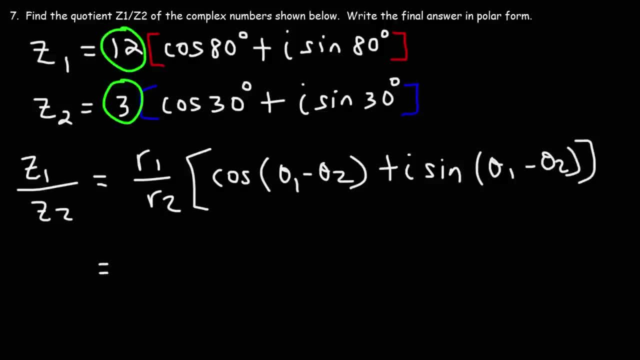 so the first thing we're going to do is divide the r values- r1 over r2, so that's going to be 12 divided by 3. and then we're going to subtract the two angles, theta1 minus theta2, so that's going to be: 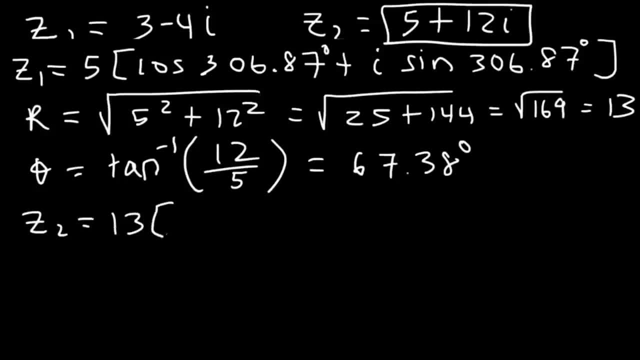 So now we can express z2 as 13 cosine 67.38 plus i sine 67.38.. So now we can find a product of z1 and z2.. So first z1 times z2, we got to multiply r1 and r2.. 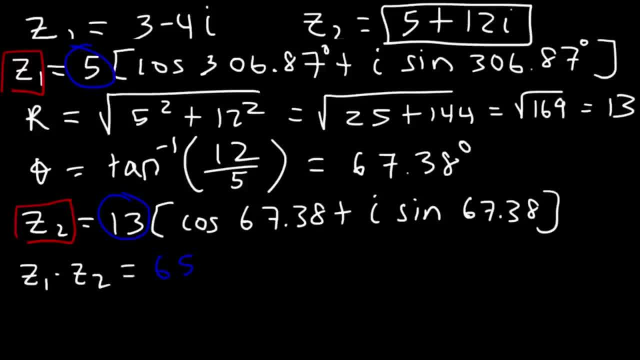 So 5 times 13 is 65.. Next we need to add the two angles. So let's add 306.87 plus 67.38. Now if you add those two angles, you're going to get 374.25. 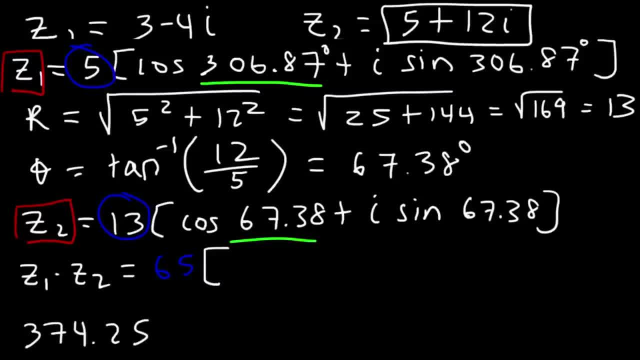 which is greater than 360. So let's find the coterminal angle between 0 and 360.. To do that, subtract it by 360. And this will give you 14.25.. So now we have the same answer. 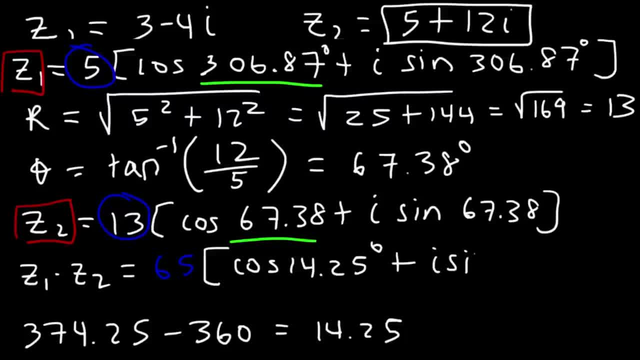 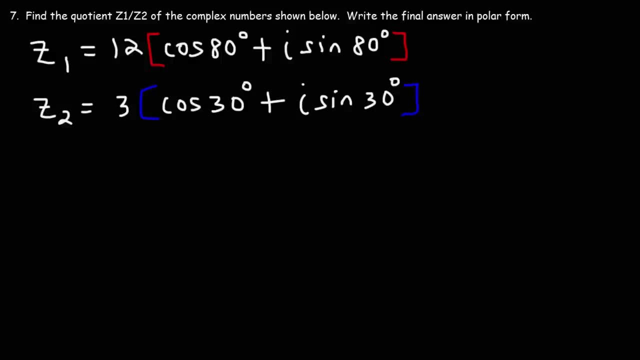 65 cosine 14.25, plus i sine 14.25. Personally, I believe that the first method is a lot easier than the second, But now you know how to do it both ways. Number 7. Find the quotient z1 over z2 of the complex numbers. 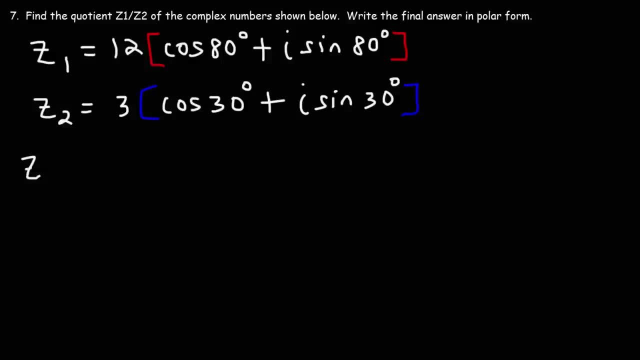 shown below. So first let's write the formula: z1 over z2 is going to be r1 over r2 times cosine of theta1 minus theta2 plus i sine theta1 minus theta2. So the first thing we're going to do is divide the r values. 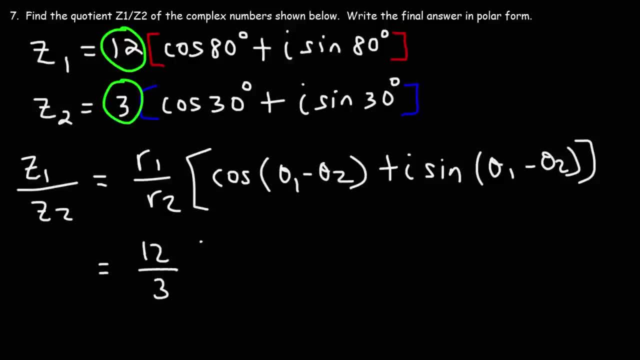 r1 over r2.. So that's going to be 12 divided by 3.. And then we're going to subtract the two angles, theta1 minus theta2.. So that's going to be 80 degrees minus 30 degrees, And then we can write our 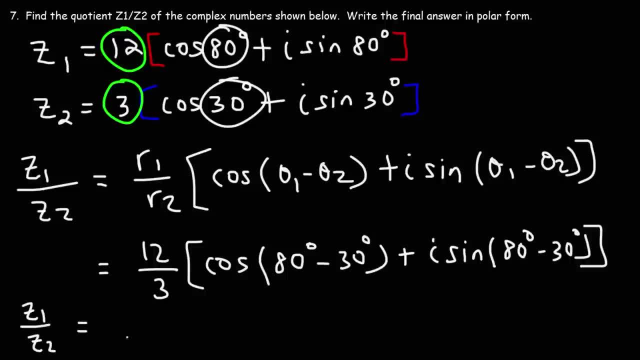 final answer. So the quotient z1 over z2 is going to be 12 divided by 3, which is 4.. And then times cosine, 80 degrees minus 30 degrees, That's going to be 50 degrees. So it's going to be cosine 50. 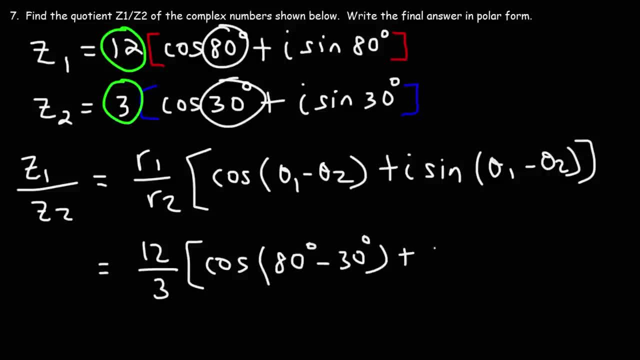 80 degrees minus 30 degrees, and then we can write our final answer. so the quotient z1 over z2 is going to be 12 divided by 3, which is 4, and then times cosine 80 degrees minus 30 degrees, that's going to be 50 degrees. 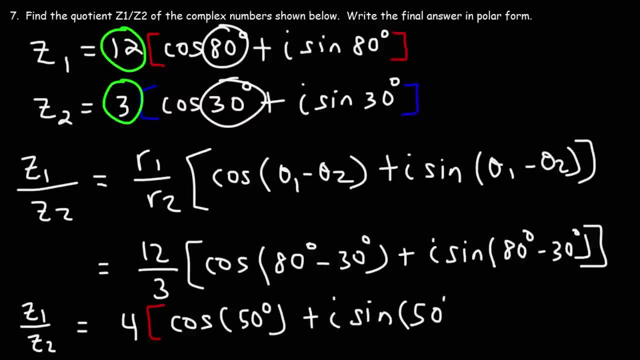 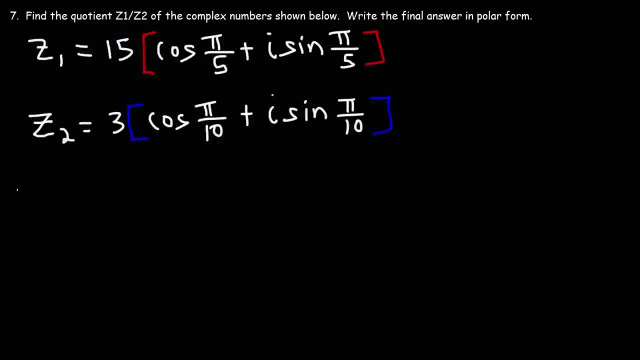 so it's going to be cosine 50 plus i sine 50 degrees, and that's our answer for this problem. now let's try an example where the angle is in radians and not degrees: z1 over z2. so let's begin by dividing the r values first. 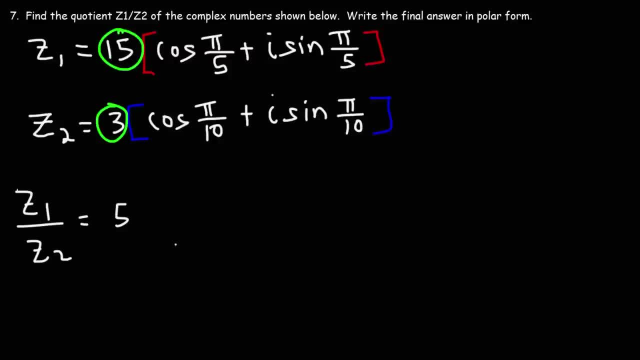 so r1 over r2, 15 divided by 3 minus 5, and then it's going to be cosine theta1 minus theta2. so let's subtract those two angles, so that's pi over 5 minus pi over 10. so we need to get common denominators first. 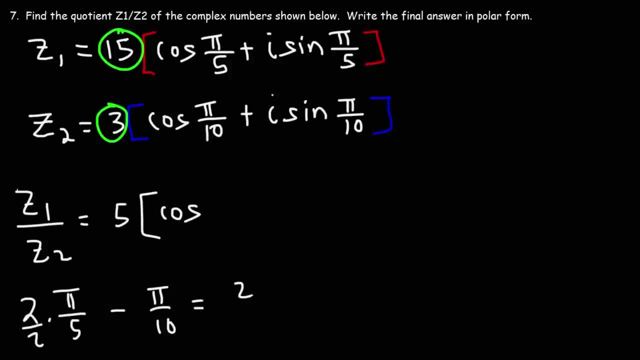 let's multiply this one by 2 over 2, so this becomes 2 pi over 10, minus pi over 10, which is the same as 1 pi over 10. 2 pi minus 1 pi is 1 pi, so the difference is pi over 10. 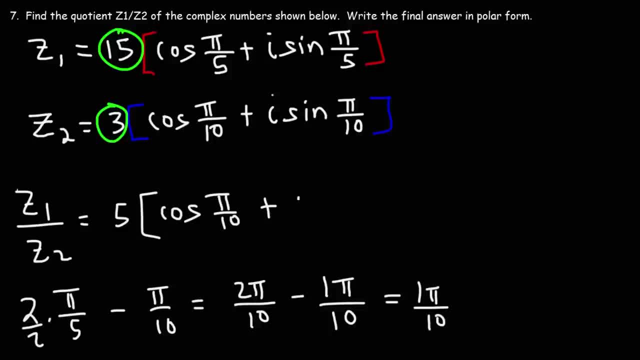 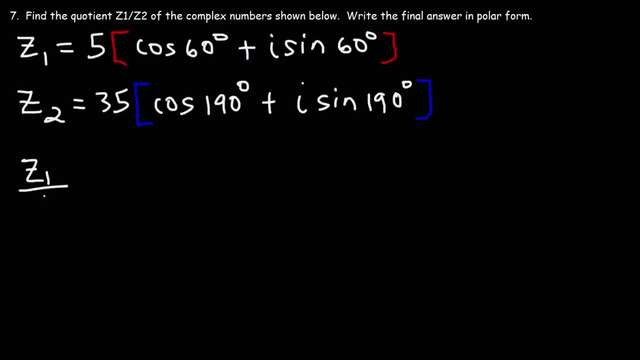 so this is going to be 5 cosine pi over 10, plus i sine pi over 10. so that's the quotient of z1 and z2 in this problem. now let's try this example. so once again we're going to find the quotient r1 over r2. 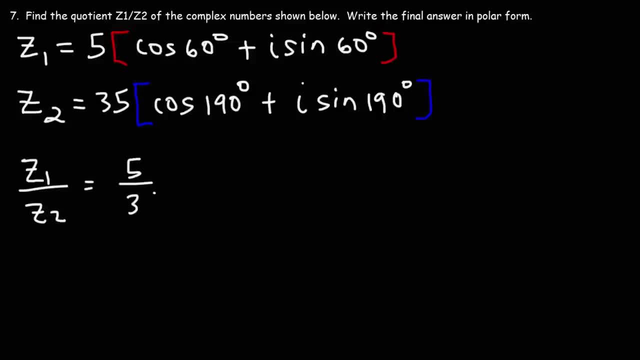 that's going to be 5 over 37. I mean not 37, but 5 over 35. and then cosine: we're going to take angle 1 and subtract it by angle 2. 60 minus 190, that's going to be negative 130. 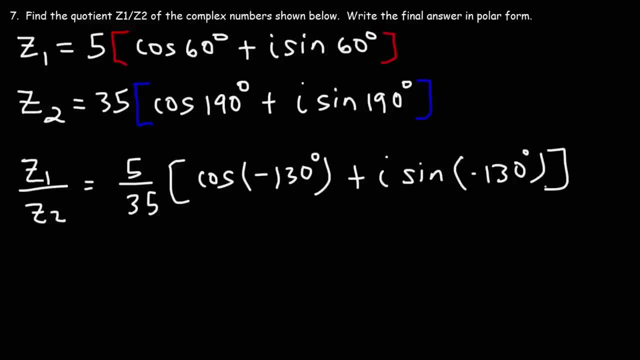 so what do we do with a negative angle? well, before we get into that, let's simplify: 5 over 35. 35 is 5 times 7, 5 is 5 times 1. so if we cancel a 5, it's going to become 1 over 7. 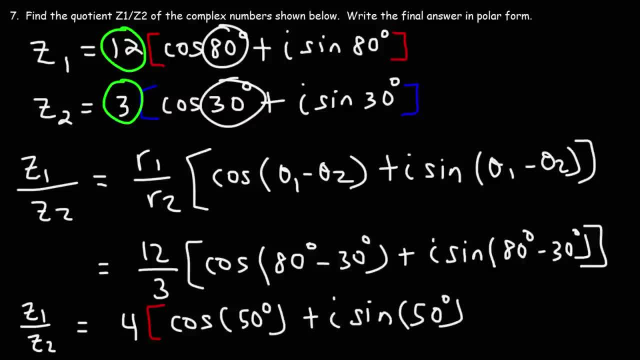 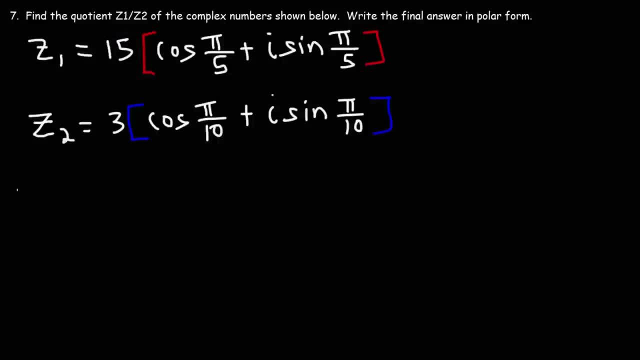 plus i sine 50 degrees, And that's our answer for this problem. Now let's try an example where the angle is in radians and not degrees, z1 over z2.. So let's begin by dividing the r values first, So r1 over r2.. 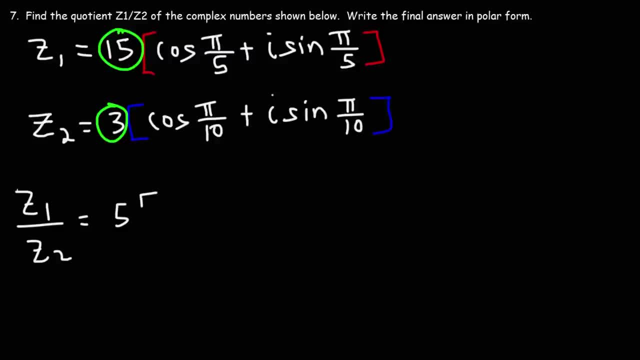 15 divided by 3.. That's going to be 5.. And then it's going to be cosine theta1 minus theta2.. So let's subtract those two angles, So that's pi over 5 minus pi over 10.. So we need to get common. 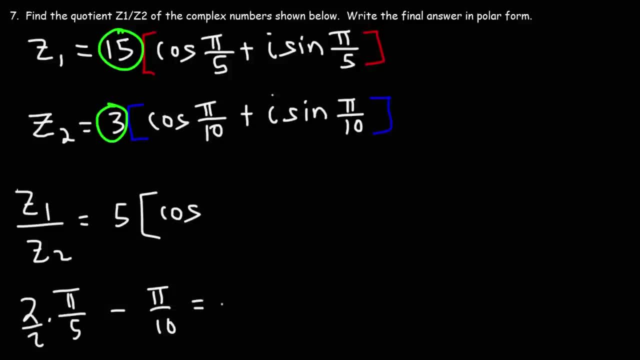 denominators. first Let's multiply this one by 2 over 2.. So this becomes 2 pi over 10 minus pi over 10, which is the same as 1 pi over 10.. 2 pi minus 1 pi is 1 pi. 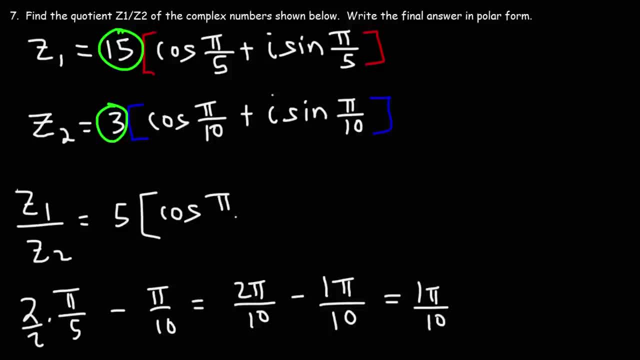 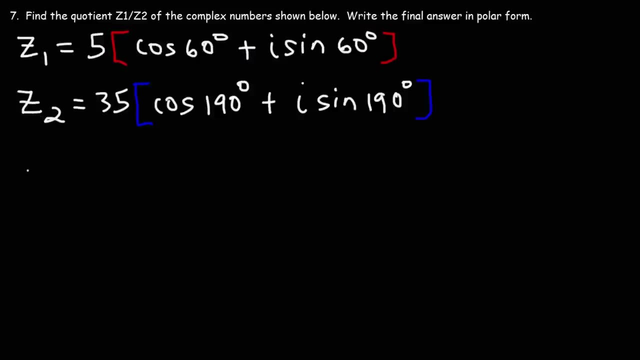 So the difference is pi over 10.. So this is going to be 5 cosine pi over 10, plus i sine pi over 10.. So that's the quotient of z1 and z2 in this problem. Now let's try this example. 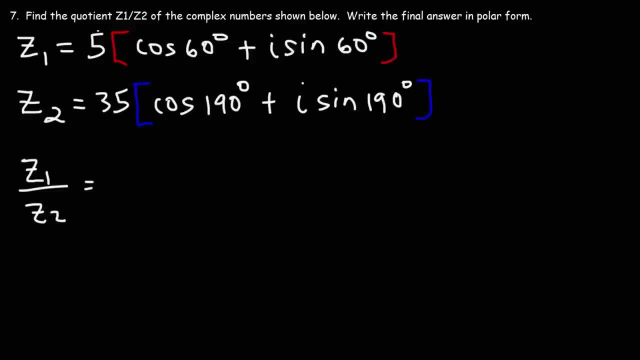 So once again, we're going to find the quotient r1 over r2.. That's going to be 5 over 36.. I mean not 37, but 5 over 35.. And then cosine: we're going to take angle 1 and subtract it by angle 2.. 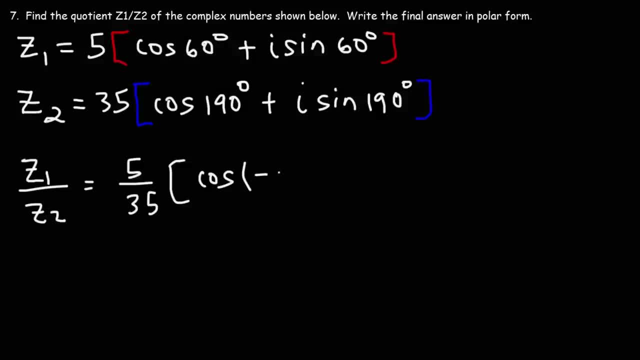 60 minus 190, that's going to be negative 130.. So what do we do with a negative angle? Well, before we get into that, let's simplify 5 over 35.. 35 is 5 times 7.. 5 is 5 times 1.. 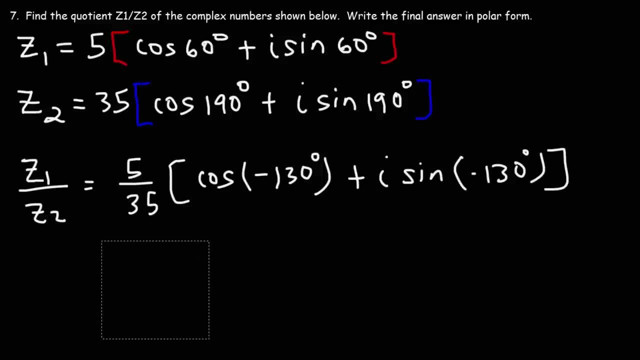 So if we cancel a 5, that's going to become 1 over 7.. Now what should we do with this negative angle? If you get a negative angle, what you want to do is find the positive coterminal angle of that angle. 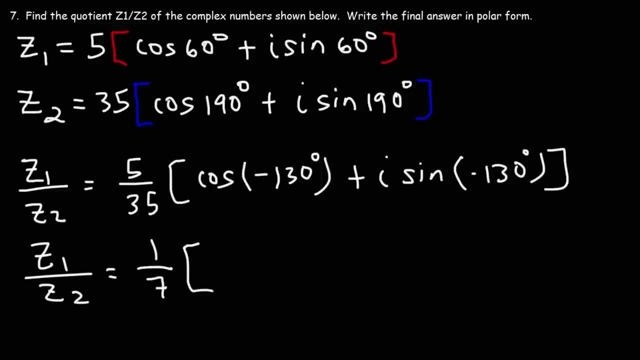 now what should we do with this negative angle? if you get a negative angle, what you want to do is find the positive coterminal angle of that angle. so to get a coterminal angle, simply add 360 to negative 130, so the coterminal angle will be. 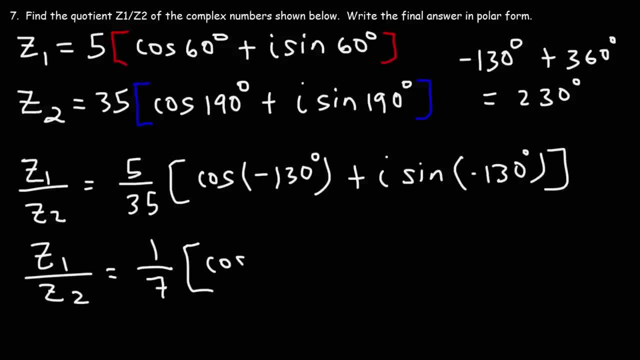 230. so this is going to be cosine 230 plus i sine 230 degrees, and here's how you know if you need to do this. I didn't put it in this problem, but when you look at your homework problem in the directions you might see something like: 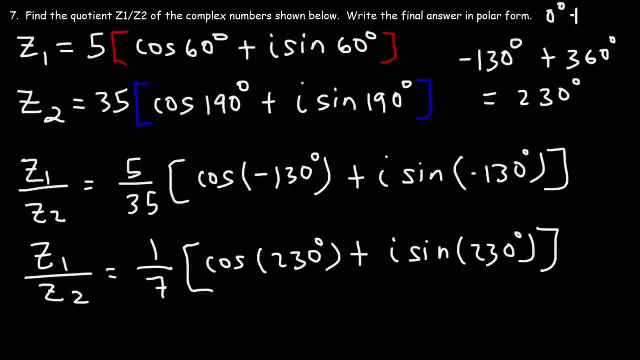 write your answer using an angle between 0 and 360 degrees, or it can be between 0 and 2 pi. typically it should be within this range. but if you leave your answer like this, it would be correct if this direction wasn't stated. but if it is stated, then 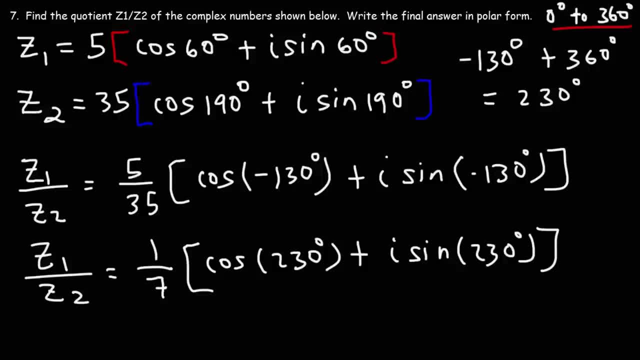 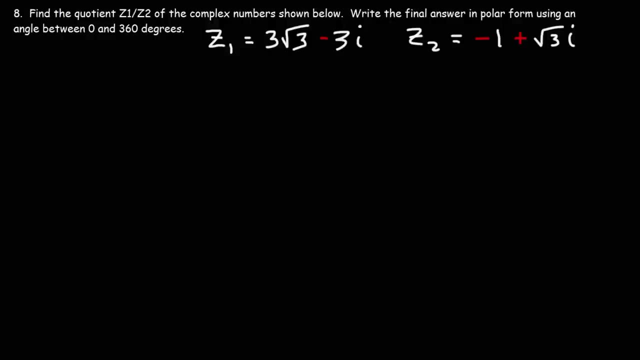 you gotta find a coterminal angle between 0 and 360, so just make sure you're aware of that. therefore, this is the final answer for this problem, number 8. so we need to find a quotient, z1 over z2, but we're given z. 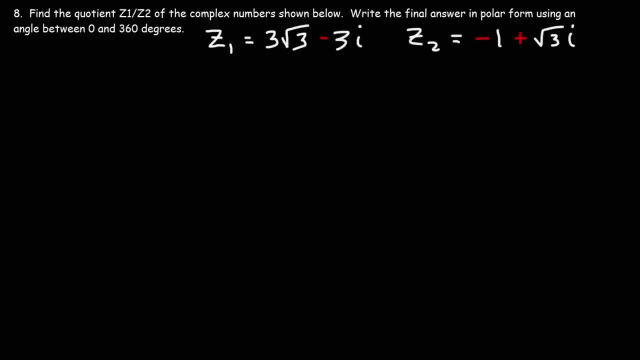 in its rectangular form. so there's two ways we could do this. we could divide z1 and z2 right now, simplify the expression and then convert it to polar form. or we could convert z1 and z2 individually in polar form and then divide it, which will give us the final answer in polar form. 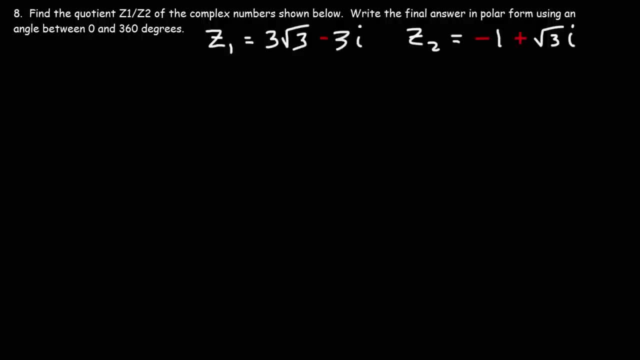 for the sake of learning, let's do it both ways. so let's divide z1 by z2 in rectangular form first. so this is going to be 3 square root 3 minus 3i, divided by negative 1 plus root 3i. so to simplify this expression, 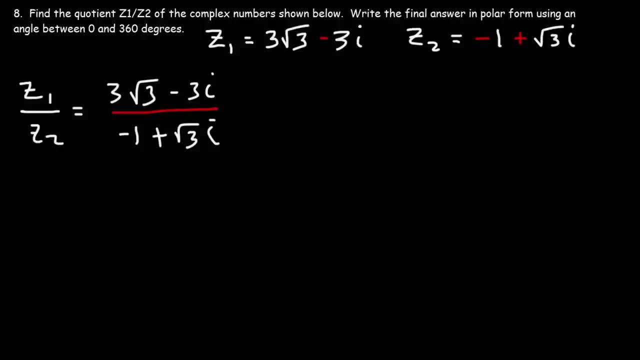 what we need to do is multiply the bottom and the top by the conjugate of the denominator. the conjugate is going to be everything that we see here, but we're going to change the positive sign to a negative sign. so now let's FOIL. this is going to be. 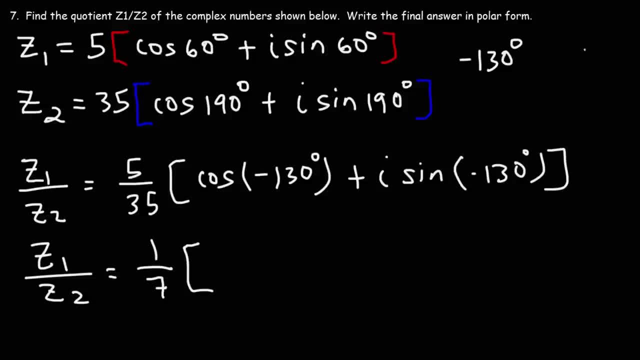 So to get a coterminal angle, simply add 360.. To negative 130.. So the coterminal angle will be 230.. So this is going to be cosine 230 plus i sine 230 degrees. And here's how you know. 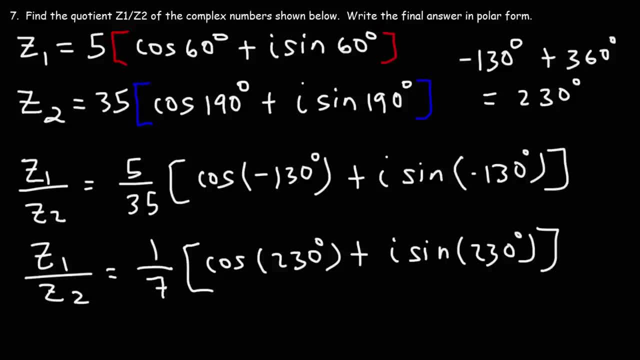 if you need to do this. I didn't put it in this problem, but when you look at your homework problem in the directions you might see something like: write your answer using an angle between 0 and 360 degrees, Or it could be between 0 and 2 pi. 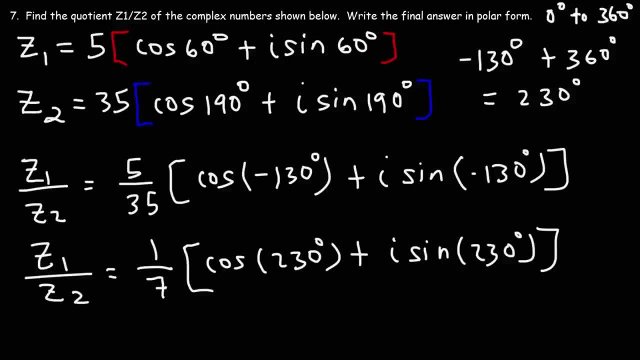 Typically it should be within this range. but if you leave your answer like this, it would be correct if this direction wasn't stated. But if it is stated, then you gotta find a coterminal angle between 0 and 360.. So just make sure you're. 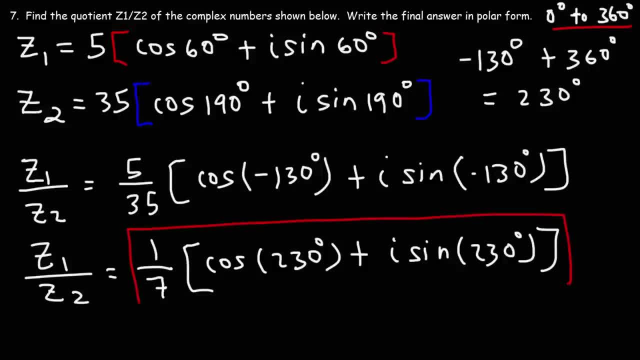 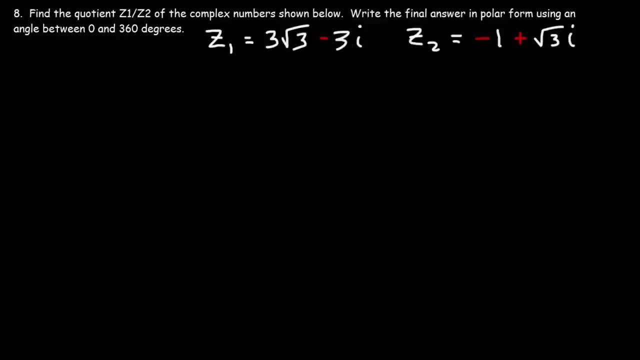 aware of that. Therefore, this is the final answer for this problem, Number 8.. So we need to find the quotient z1 over z2, but we're given z in its rectangular form. So there's two ways we could do this. We could divide z1 and z2 right now. 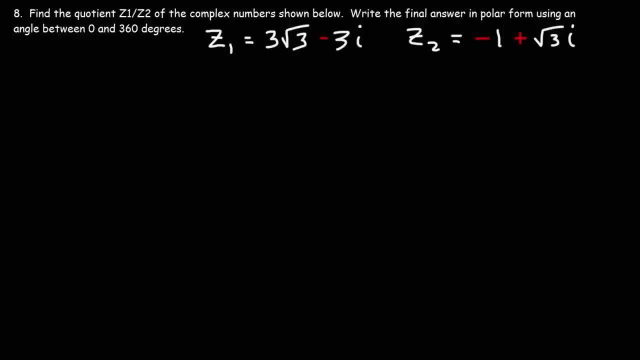 simplify the expression and then convert it to polar form. Or we could convert z1 and z2 individually in polar form and then divide it, which will give us the final answer in polar form. For the sake of learning, let's do it both ways. 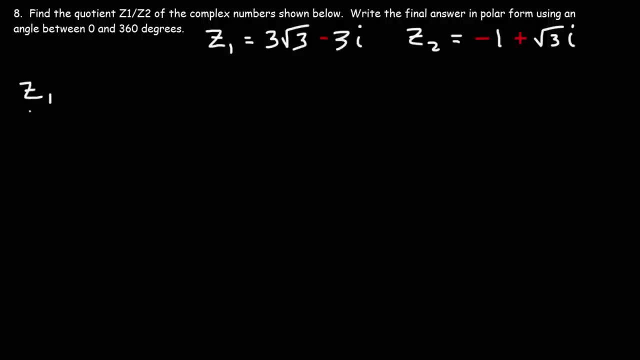 So let's divide z1 by z2 in rectangular form first. So this is going to be 3 square root 3 minus 3i, divided by negative 1 plus root 3i. So to simplify this expression, what we need to do is multiply the bottom. 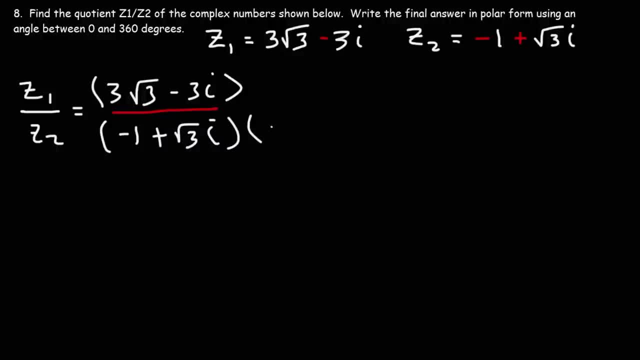 and the top by the conjugate of the denominator. The conjugate is going to be everything that we see here, but we're going to change the positive sign to a negative sign. So now let's FOIL. This is going to be negative. 3, root 3. 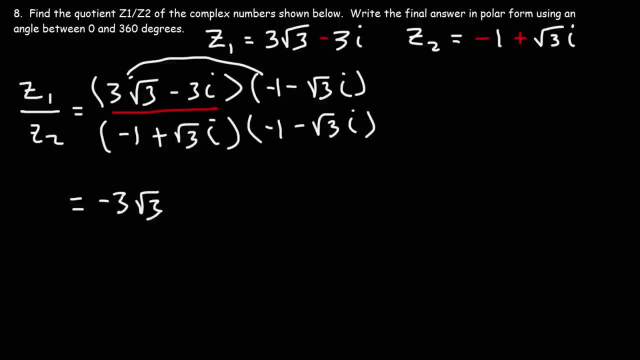 negative 3 root 3, and then that's going to be minus 3, the square root of 3 times the square root of 3, that's another 3, and then times i, and then here we're going to have positive 3i, the two negative signs. 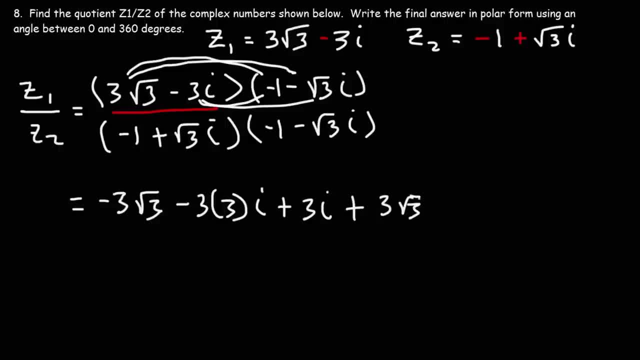 will cancel. so it's going to be positive 3 root 3. i times i, which is i squared on the bottom. we're going to have negative 1 times negative 1, which is 1, this term, which is positive root 3i. that's going to cancel with negative root 3i. 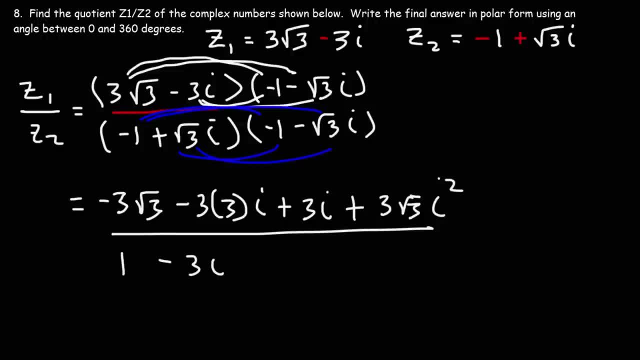 the last term will be negative 3 times i squared. so now let's see what we can do to simplify. so here we have negative 9i plus 3i and i squared is negative 1. so this becomes negative root 3. square root 3. 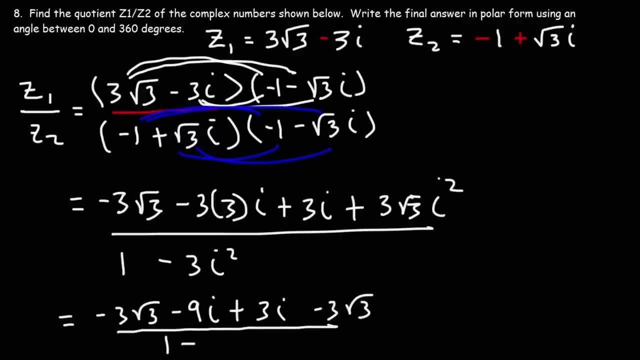 on the bottom we have 1 minus i squared is negative 1, so negative 3 times that that becomes positive 3. now we can combine these two terms, so that's going to be negative 6, square root 3 and then negative 9i plus 3i. 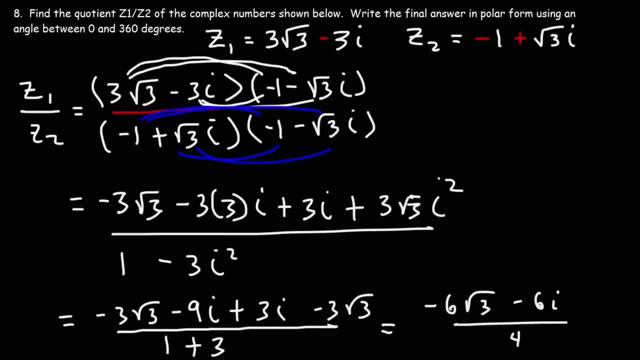 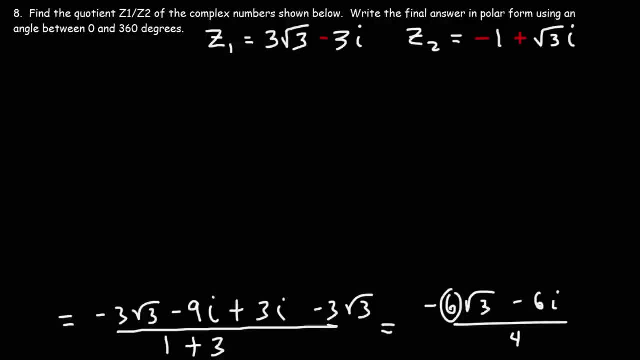 that's negative 6i. now we can divide these three numbers by 2, so z1 over z2 is going to be negative 3 square root, 3 over 2 minus 3 over 2i. so at the same time we could break this. 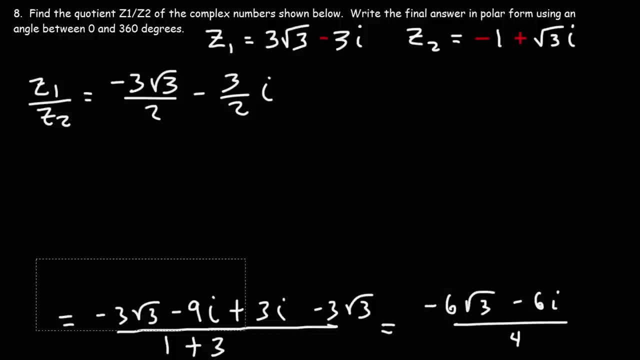 fraction into two smaller fractions. so now we have the ratio of z1 and z2 in a plus bi format, so we can go ahead and convert it into its polar form. so r is going to be the square root of negative 3, square root 3 over 2. 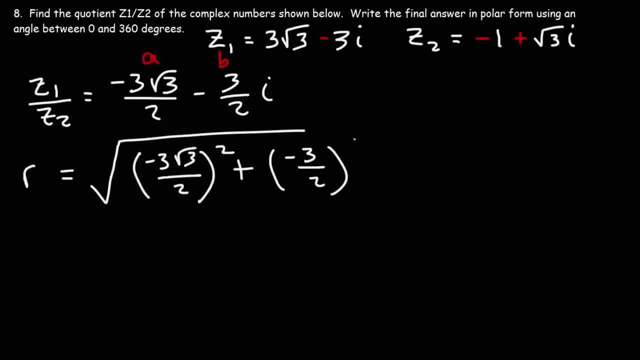 squared plus negative 3 over 2 squared, negative 3 squared, that's going to be 9, the square root of 3 squared, that's the square root of 9, which is 3 divided by 2 squared, which is 4 negative 3 over 2 squared. 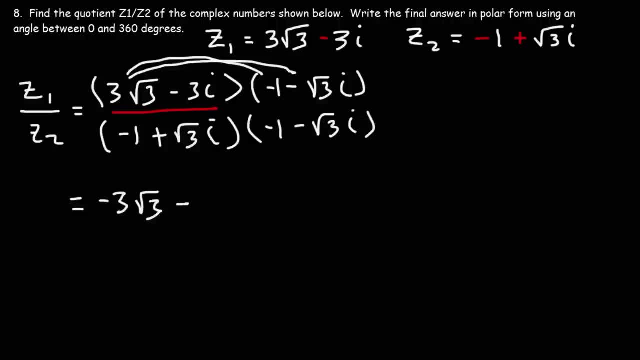 and then that's going to be minus 3, the square root of 3 times the square root of 3, that's another 3, and then times i, and then here we're going to have positive 3i. the two negative signs will cancel, so it's going to be positive 3 root 3. 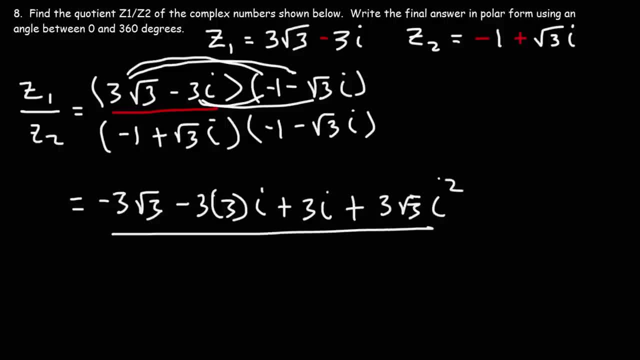 i times i, which is i squared On the bottom, we're going to have negative 1 times negative 1, which is 1. This term, which is positive root 3i, that's going to cancel with negative root 3i, The last term will be. 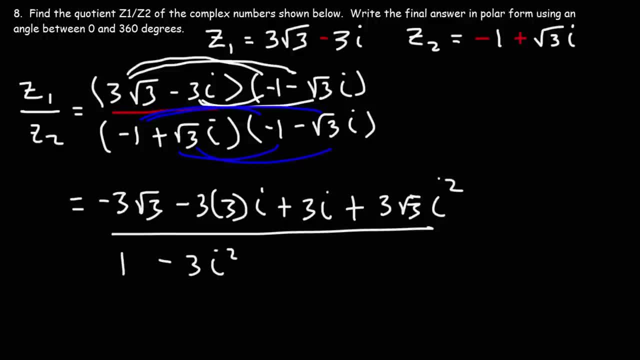 negative 3 times i squared. So now let's see what we can do to simplify. So here we have negative 9i plus 3i and i squared is negative 1. so this becomes negative root 3, square root 3. On the bottom we have: 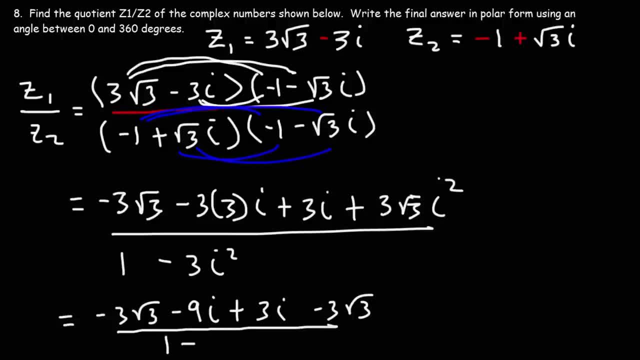 1 minus i squared is negative 1, so negative 3 times that that becomes positive 3. Now we can combine these two terms, so that's going to be negative 6, square root 3, and then negative 9i plus 3i, that's negative 6i. 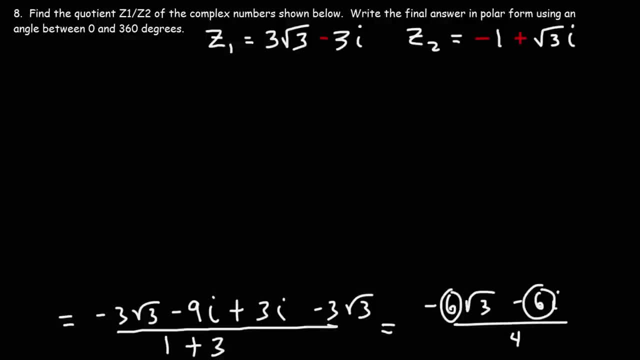 Now we can divide these three numbers by 2, So z1 over z2 is going to be negative. 3 square root, 3 over 2 minus 3 over 2i. So at the same time we can break this fraction into two smaller fractions. 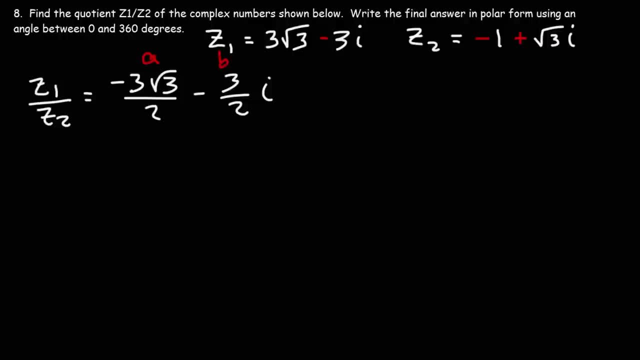 So now we have the ratio of z1 and z2 in a plus bi format, So we can go ahead and convert it into its polar form. So r is going to be the square root of negative 3, square root 3 over 2 squared plus. 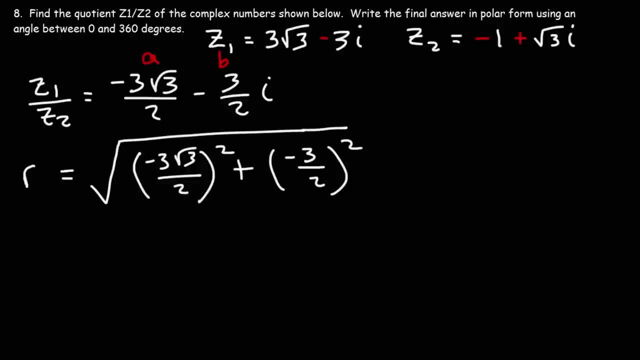 negative: 3 over 2 squared. negative 3 squared, that's going to be 9, the square root of 3 squared, that's the square root of 9, which is 3 divided by 2 squared, which is 4. negative 3 over 2 squared. 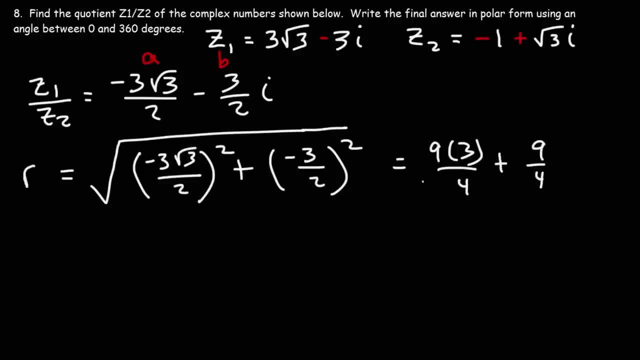 that's going to be 9 over 4. 9 times 3 is 27, so we have 27 over 4 plus 9 over 4. 27 plus 9 is 36, and 36 divided by 4 is 9 and the square root of 9 is 3. 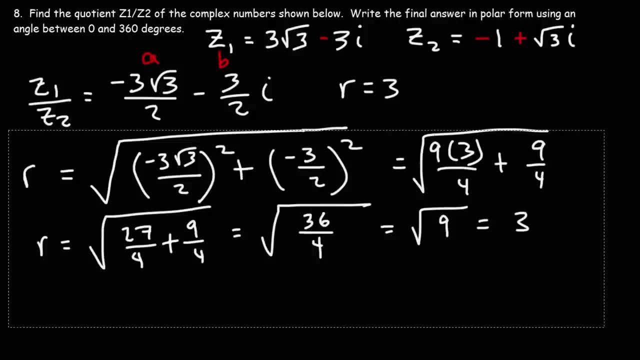 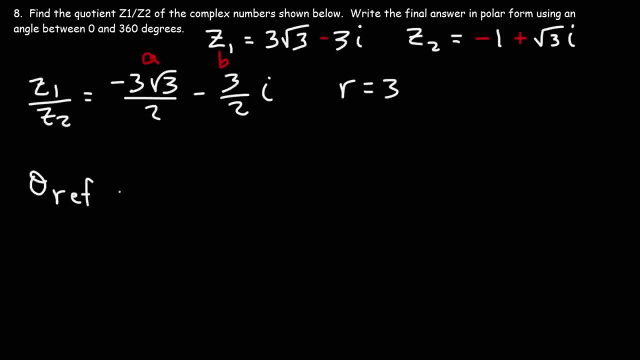 so we get that r is equal to 3. Now the next thing that we need to find is the angle, theta, but we're going to find the reference angle first. so this is going to be arc tangent: b over a, b is negative, 3 over 2. 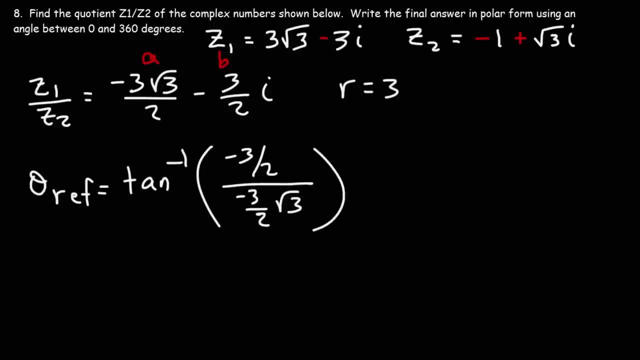 a is negative 3 over 2, but times the square root of 3, so we could cancel negative 3 over 2. this gives us the arc tangent of 1 divided by the square root of 3, and we can rationalize this if we want to. 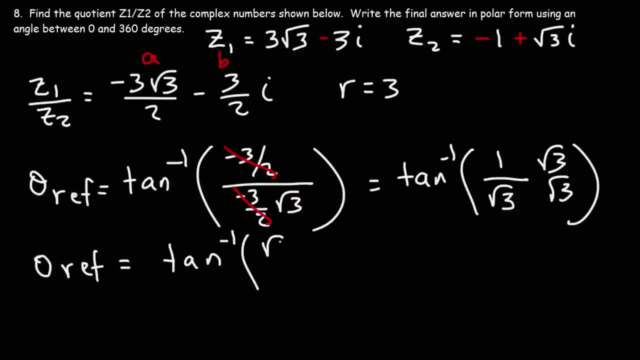 so this is arc tangent square root 3 over 3 and this is equal to 30 degrees and you can plug it in your calculator. tangent of 30 degrees is first. we have to make sure it's in degree mode. tan 30 is .57735. 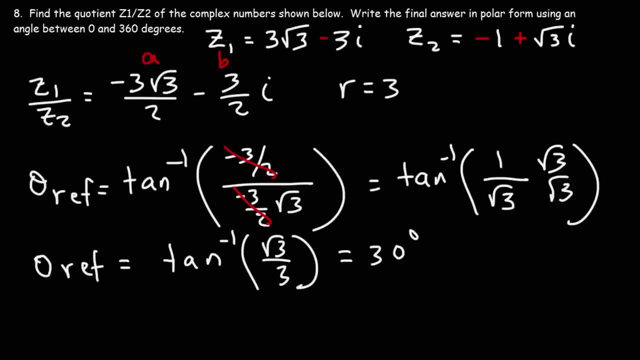 which is the square root of 3 over 3, so it helps to know the 30- 60, 90 triangle to figure this out. now, even though the reference angle is 30, that may not be the final angle that we're looking for, so we need to adjust it. 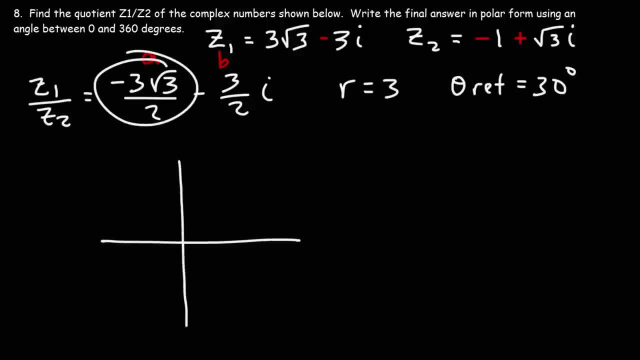 a is negative and b is negative, so the real angle that we're looking for is in quadrant 3, so this is the reference angle 30, that's the angle inside the triangle. we want the angle measured from the positive x-axis, so it's 180 plus 30. 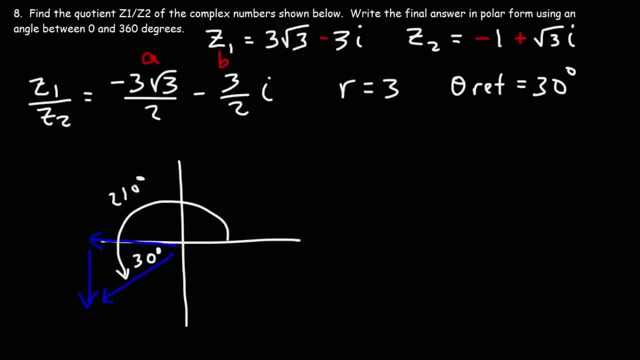 so that will give us a combined angle of 210. so now that we have r and theta, we can write our final answer. z1 over z2 is going to be r, which is 3 times cosine of the angle, that's cosine 210 plus i sine. 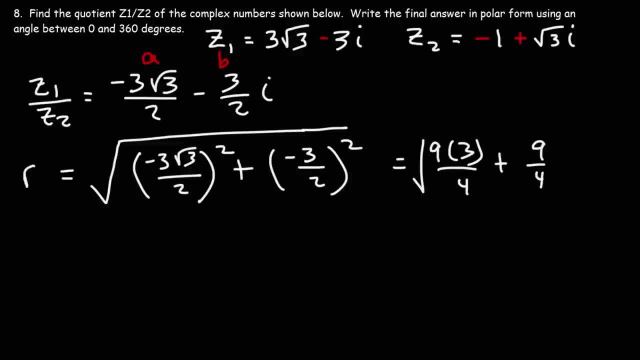 that's going to be 9 over 4. 9 times 3 is 27, so we have 27 over 4 plus 9 over 4. 27 plus 9 is 36, and 36 divided by 4 is 9 and the square root of 9 is 3. 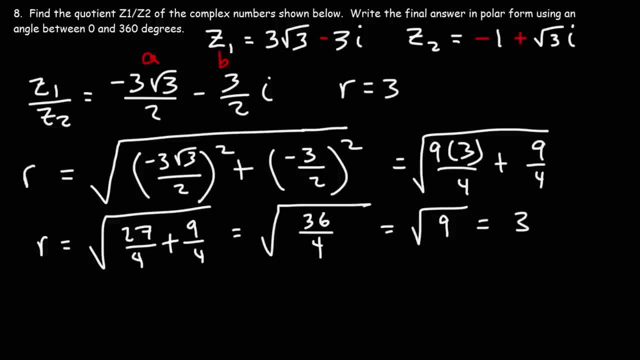 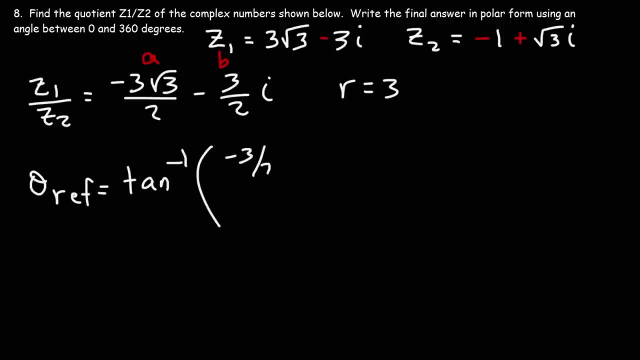 so we get that r is equal to 3. now the next thing that we need to find is the angle, theta, but we're going to find the reference angle first. so this is going to be arc tangent: b over a, b is negative, 3 over 2. 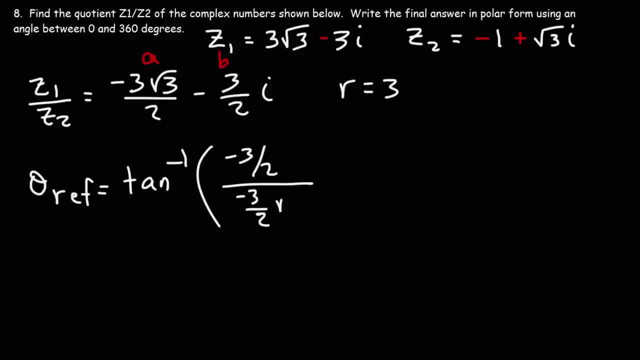 a is negative 3 over 2, but times the square root of 3, so we could cancel negative 3 over 2. this gives us the arc tangent of 1 divided by the square root of 3, and we can rationalize this if we want. 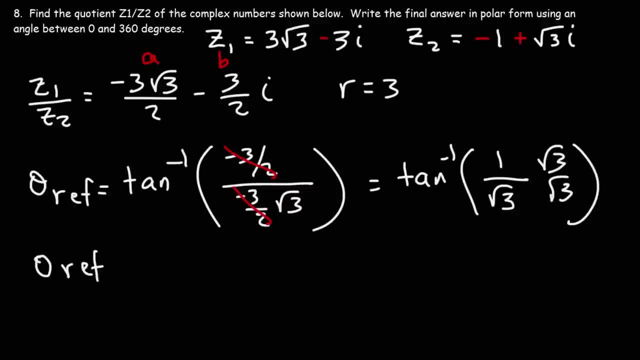 to. so this is arc tangent square root 3 over 3 and this is equal to 30 degrees and you could plug it in your calculator. tangent of 30 degrees is first. we have to make sure it's in degree mode. tan 30 is 0.57735. 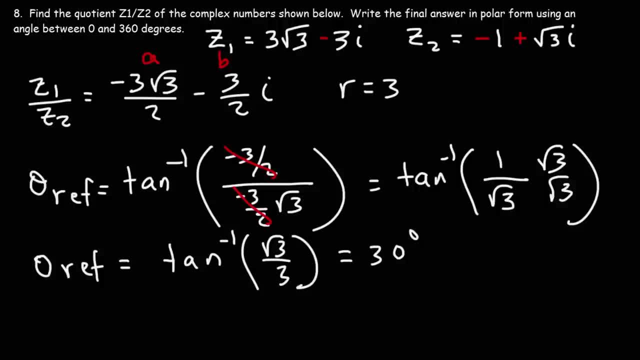 which is the square root of 3 over 3. so it helps to know the 30-60-90 triangle to figure this out now, even though the reference angle is 30, that may not be the final angle that we're looking for, so we need. 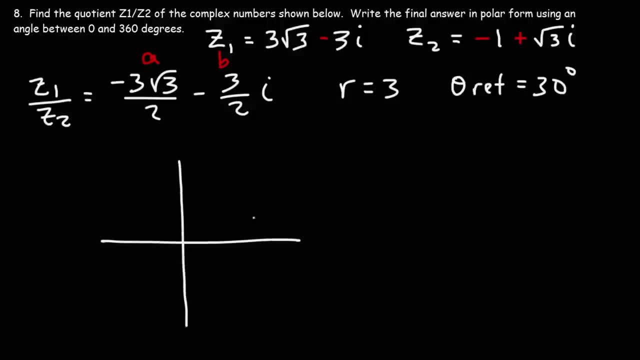 to adjust it. a is negative and b is negative, so the real angle that we're looking for is in quadrant 3, so this is the reference angle 30, that's the angle inside the triangle. we want the angle measured from the positive x-axis, so it's 180. 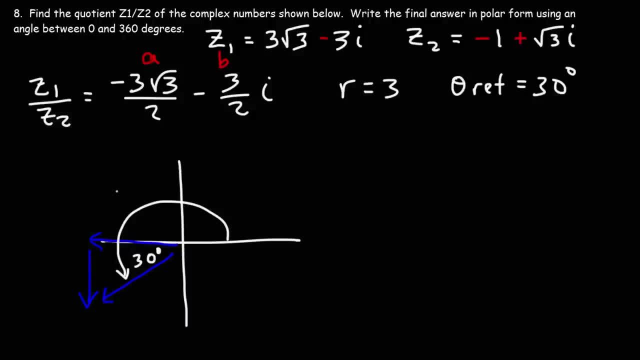 plus 30. so that will give us a combined angle of 210. so now that we have r and theta, we can write our final answer. z1 over z2 is going to be r, which is 3 times cosine of the angle, that's cosine 210. 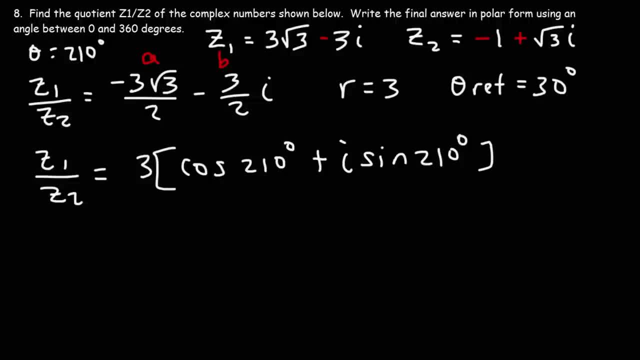 plus i, sine 210 degrees. so this, right here, is our final answer. now let's see if we can get the same answer using another method. so what we're going to do is we're going to convert z1 and z2 into polar form and then we'll divide it. 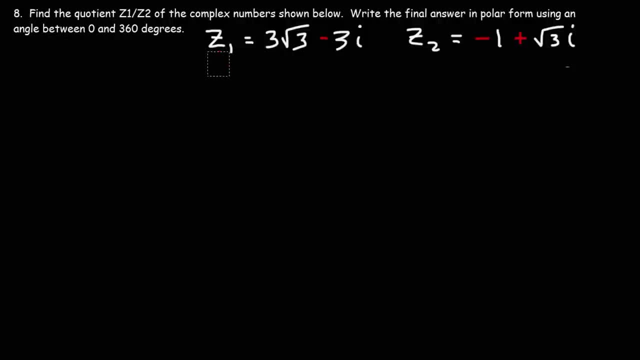 if you need to double check the answer, feel free to rewind the video. so let's convert z1 into polar form. let's calculate r first. so this is going to be the square root of a squared. so a is 3, square root 3, and then 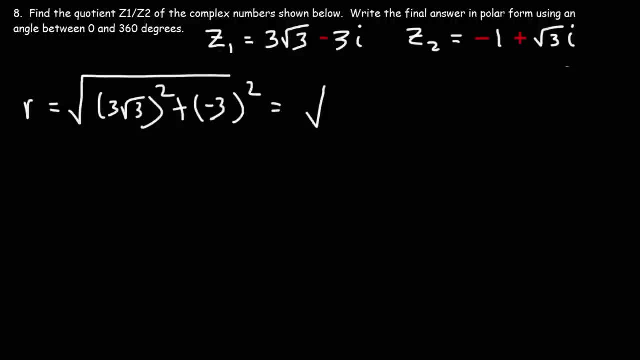 plus b squared, b is negative 3, so 3 squared is 9, and the square root of 3 squared is going to be 3, and negative 3 squared is 9 is 1 as well. so this is 27 plus 9, which is 36. 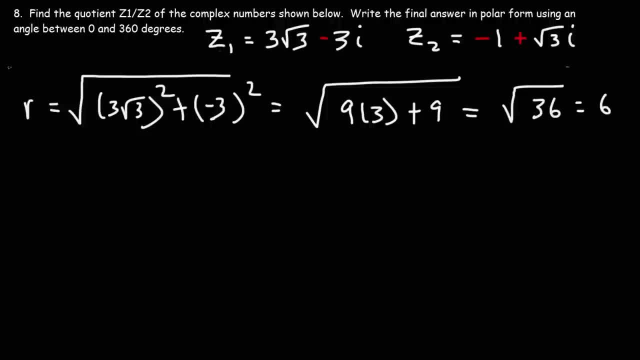 and the square root of 36 is 6. so we got that r is equal to 6. now let's find the reference angle. the reference angle is going to be r tangent b over a. b is negative 3. well, let's use positive 3. 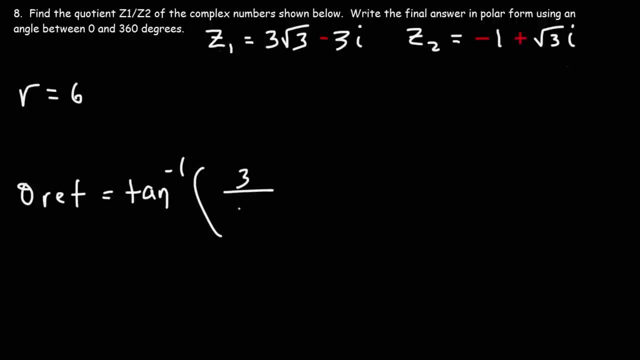 for now, so we can get the reference angle. so positive, 3 for b and a is 3, square root 3, the 3's will cancel. so once again, this is r tangent 1 over the square root of 3, which we know it to be 30 degrees. 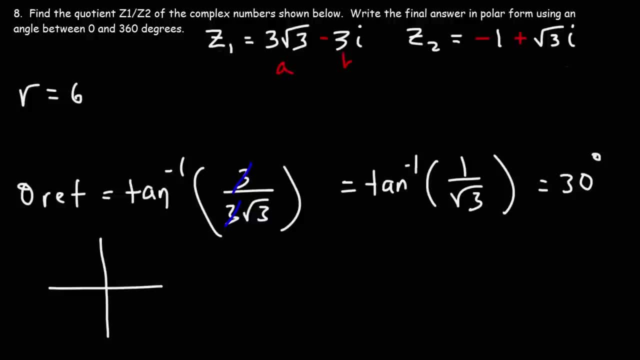 now a is positive, b is negative, so that's positive a, negative b. so that's in quadrant 4, which means the angle is going to be 360 minus 30, so that's 330 degrees. so we can write that z1 in polar form is going to be r. 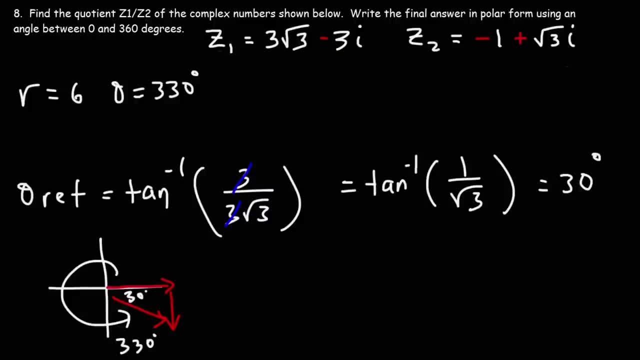 which is 6 times cosine of 330 plus i sine 330. now let's convert z2 to r, which is r tangent b over a b. now let's convert z2 from rectangular form to polar form. so let's begin by calculating r so a. 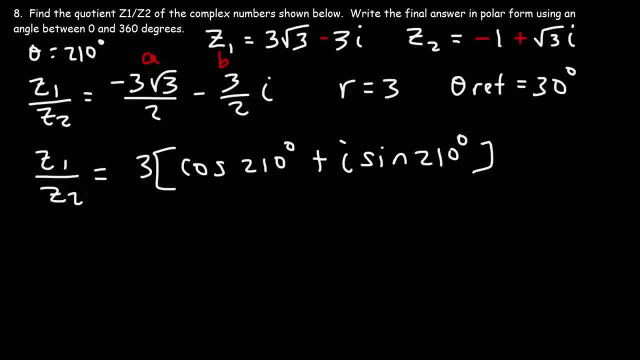 210 degrees. so this, right here, is our final answer. now let's see if we can get the same answer using another method. so what we're going to do is we're going to convert z1 and z2 into polar form, and then we'll divide it. 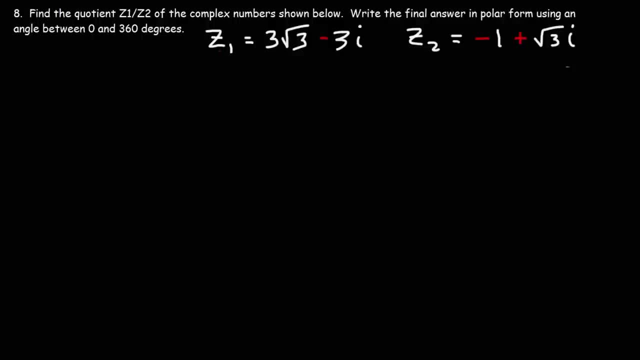 if you need to double check the answer, feel free to rewind the video. so let's convert z1 into polar form. let's calculate r first. so this is going to be the square root of a squared. so a is 3 square root 3 and then plus b squared. 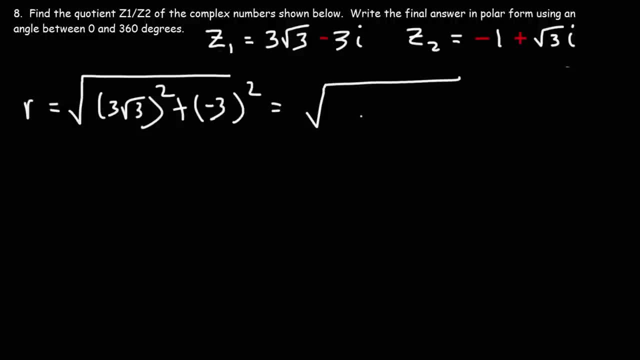 b is negative 3, so 3 squared is 9. the square root of 3 squared is going to be 3, and negative 3 squared is 9 as well. so this is 27 plus 9, which is 36, and the square root of 36 is 6. 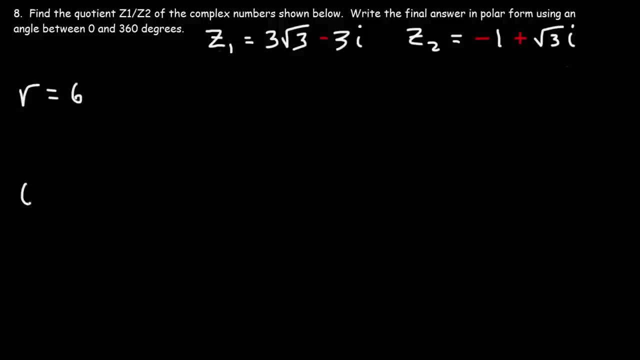 so we got that r is equal to 6. now let's find the reference angle. the reference angle is going to be r tangent b over a. b is negative 3. well, let's use positive 3 for now so we can get the reference angle. so positive 3 for b and a is 3, square root 3. 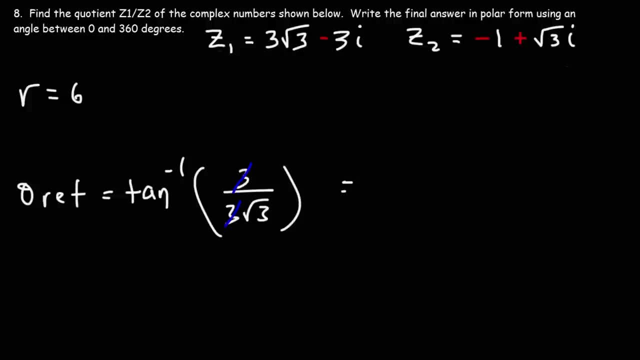 the 3's will cancel. so once again, this is r tangent 1 over the square root of 3, which we know it to be 30 degrees. now, a is positive, b is negative. so that's positive a, negative b. so that's in quadrant 4. 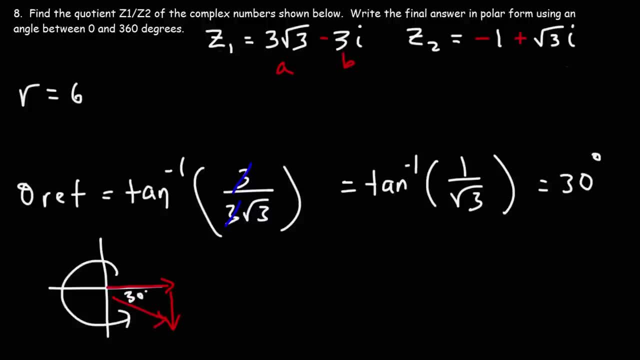 which means the angle is going to be 360 minus 30, so that's 330 degrees. so we can write that z1 in polar form is going to be r, which is 6 times cosine of 330 plus i sine 330. now let's convert z2. 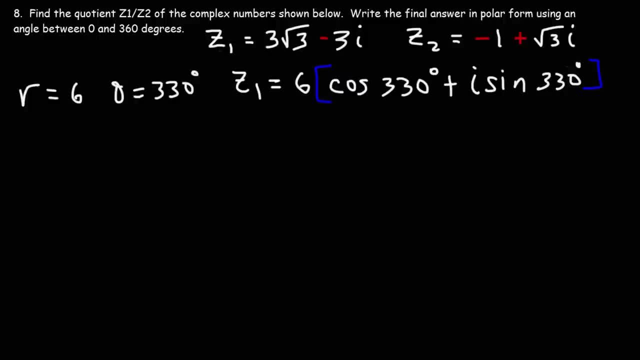 from rectangular form to polar form. so let's begin by calculating r. so a is negative 1, b is the square root of 3, so this is 1 plus 3, so we get the square root of 3 plus the square root of 4. 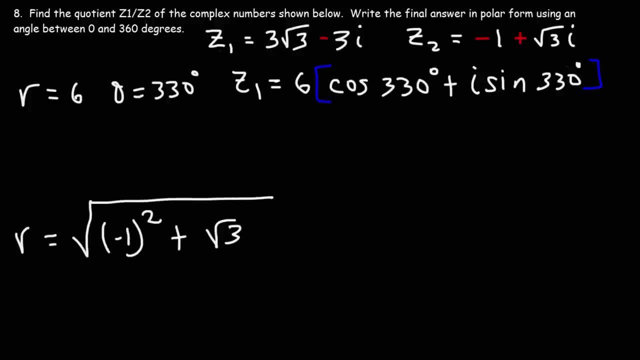 is negative. 1. b is the square root of 3, so this is 1 plus 3, so we get the square root of 4, which is 2, so r is 2. now let's calculate the angle. so the reference angle is going to be: 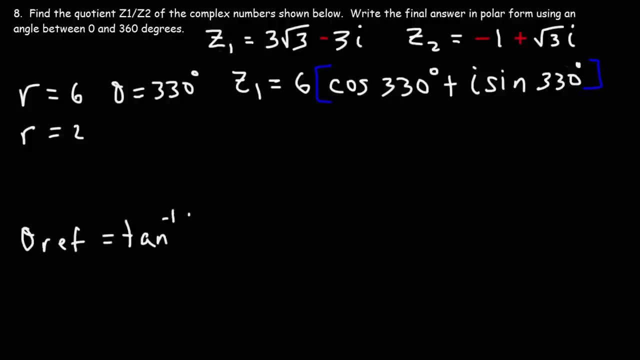 arctangent b over a. b is the square root of 3. we're going to use the positive value for a, now arctan root 3. this will give you 60 degrees. now you can always confirm your answer using the 30, 60, 90 degree triangle. 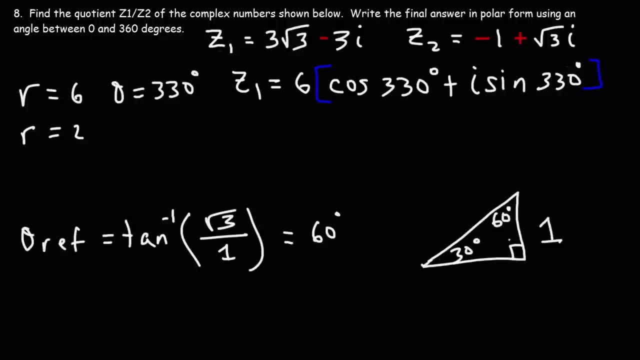 across the 30 degree angle is 1, the hypotenuse is 2. across the 60 degree angle is the square root of 3. so if you want to evaluate tangent of 30, it's going to be opposite of 30 divided by adjacent, based on SOHCAHTOA. 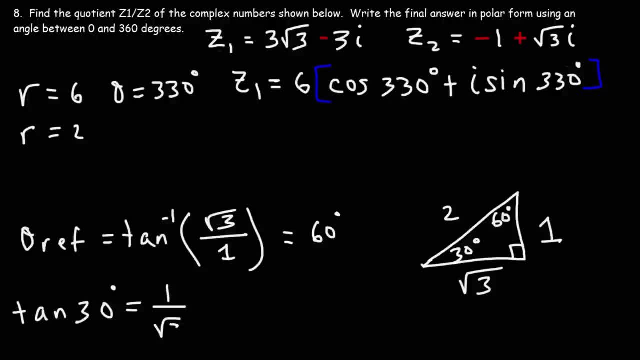 so opposite over adjacent, that's 1 over the square root of 3, which is the same as root 3 over 3. so that's why arctangent of root 3 over 3 was 30, now tangent of 60 degrees. so opposite over adjacent, opposite to 60. 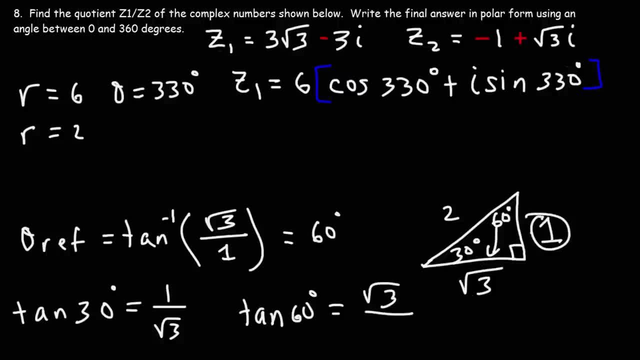 is root 3, adjacent to it is 1, so tan 60 is root 3, so arctangent of root 3 is 60. so that's how you can figure out what the angles are. it's by knowing the 30, 60, 90 triangle. 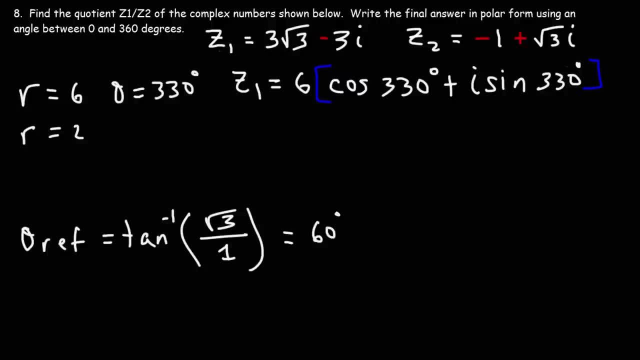 and SOHCAHTOA. so now that we have the reference angle, we need to find out what the actual angle is from the positive x axis. a is negative, b is positive, so this is going to be in quadrant 2. so here's our reference angle of 60. 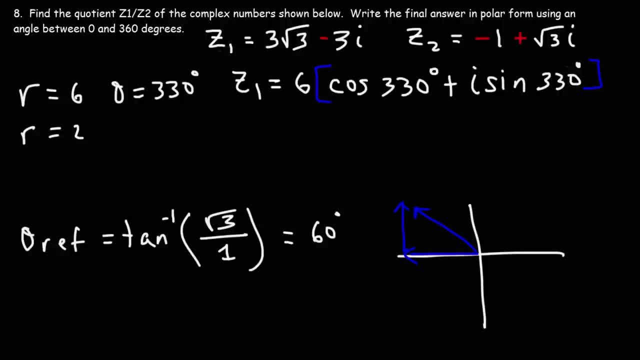 so this has to be 180 minus 60, which is 120. so z2 is going to be r, which is 2 times cosine of 120 plus i sine, which is 2 times cosine of 120 plus i sine, which is 2 times cosine. 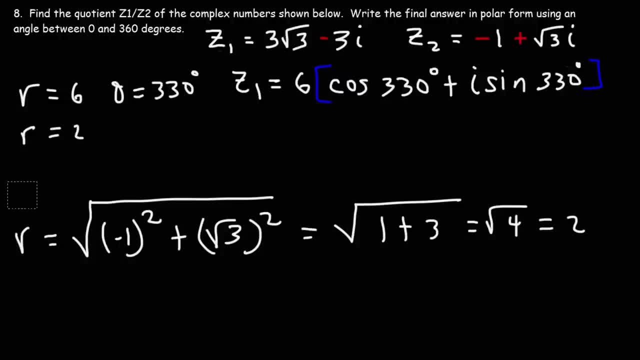 which is 2. so r is 2. now let's calculate the angle. so the reference angle is going to be arc tangent b over a. b is the square root of 3. we're going to use the positive value for a. now arc tan root 3. 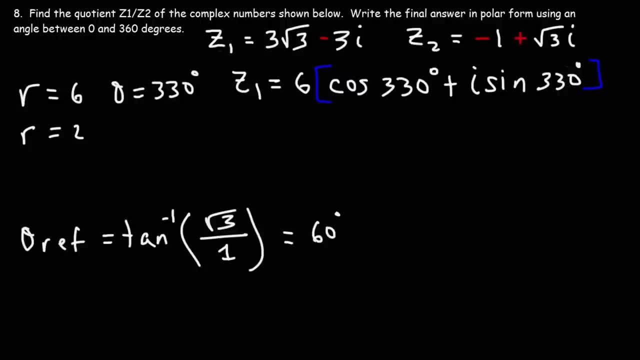 this will give you 60 degrees. now you can always confirm your answer using a 30, 60, 90 degree triangle. across the 30 degree angle is 1, the hypotenuse is 2. across the 60 degree angle is the square root of 3. 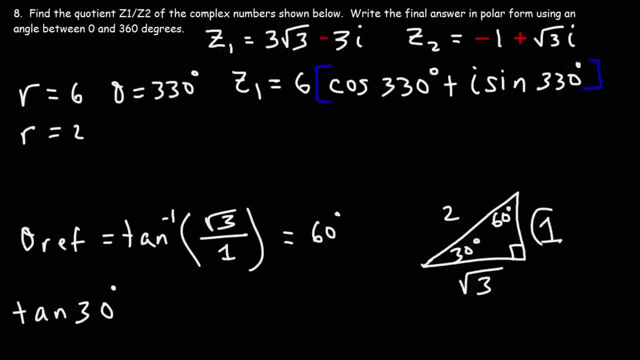 so if you want to evaluate tangent of 30, it's going to be opposite of 30 divided by adjacent, based on SOHCAHTOA. so opposite over adjacent, that's 1 over the square root of 3, which is the same as root 3 over 3. 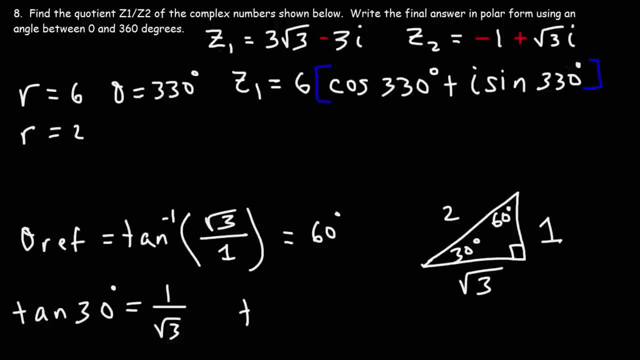 so that's why arc tangent of root 3 over 3 was 30 degrees. so opposite over adjacent, opposite to 60 is root 3. adjacent to it is 1. so tan 60 is root 3. so arc tangent of root 3 is 60. 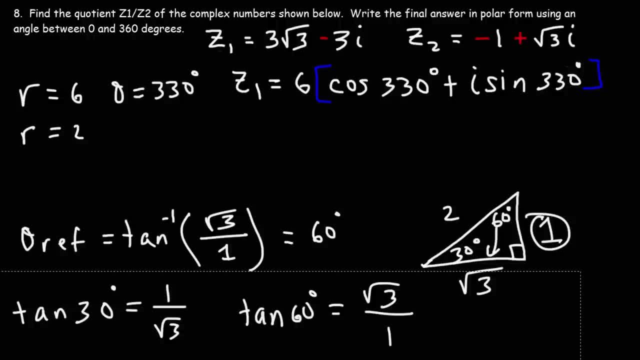 so that's how you can figure out what the angles are. it's by knowing the 30, 60, 90 triangle and SOHCAHTOA. so now that we have the reference angle, we need to find out what the actual angle is from the positive x axis. 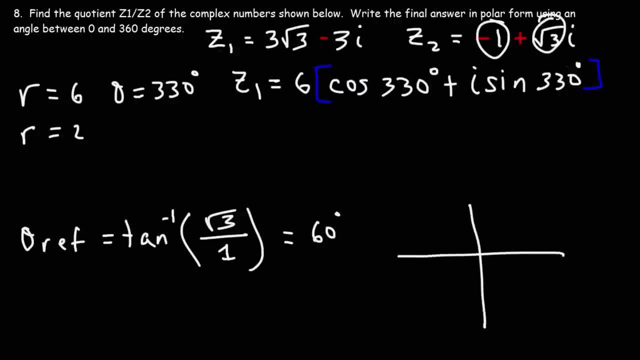 a is negative, b is positive, so this is going to be in quadrant 2. so here's our reference angle of 60. so this has to be 180 minus 60, which is 120. so z2 is going to be r, which is 2. 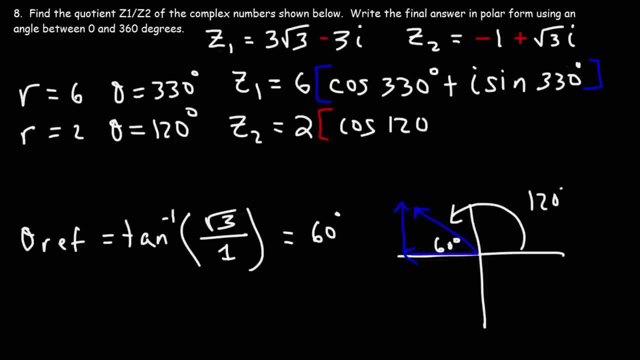 times cosine of 120 plus i sine 120. so now that we have z1 and z2 in polar form, we can divide them to get z1 over z2. so first we're going to divide the r values: 6 divided by 2 is 3.